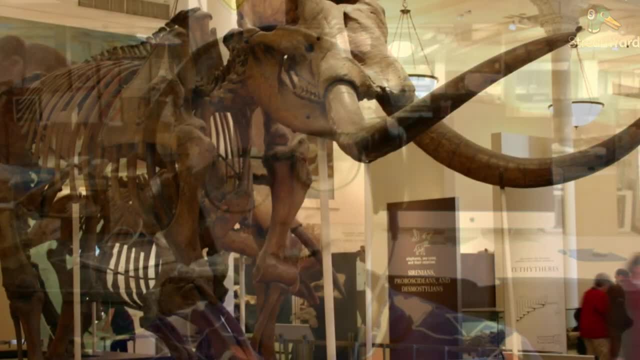 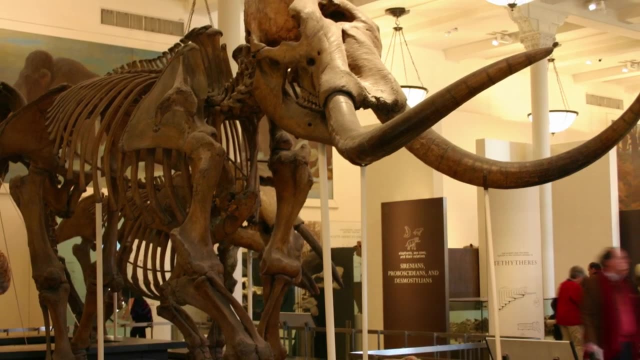 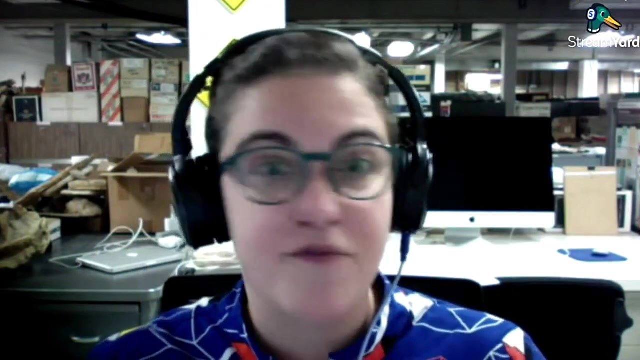 Michigan. So in the state of Michigan, our state fossil is a mastodon, So a type of proboscidean, a type of ancient mammoth, And so growing up I was just really used to hearing about the fossils, that of the animals that used to live where I lived, And I just thought that was super cool. 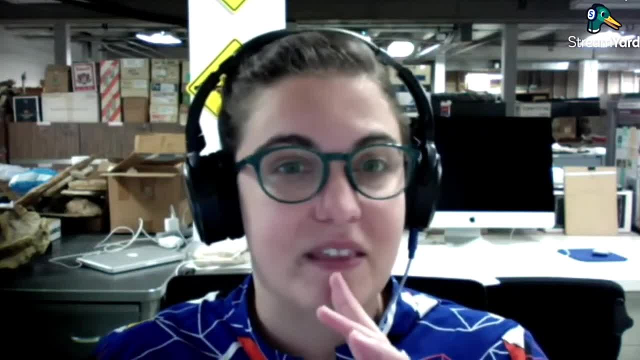 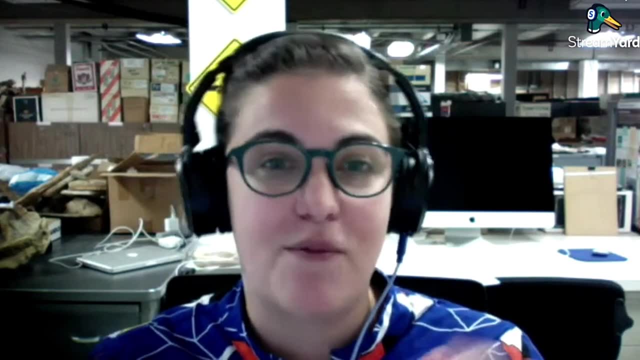 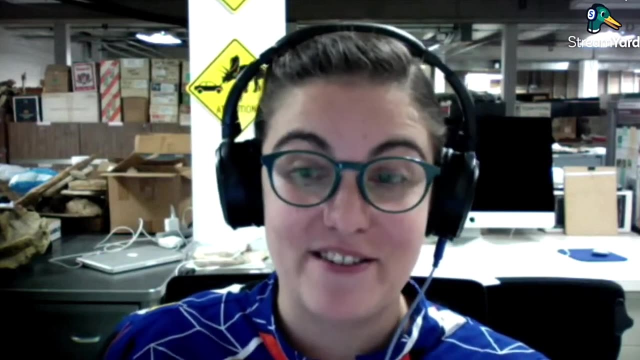 And so I wanted to be a paleontologist for ever. One of the when I was in kindergarten, I wrote this like no, it was in first grade. I wrote this like all about me thing And it said: when I grow up, I want to be a paleontologist, But I wanted to be a vertebrate paleontologist. 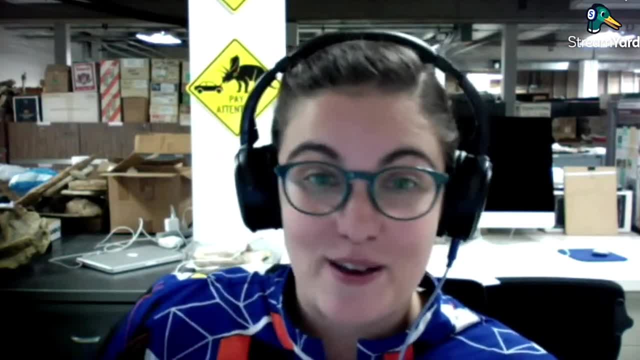 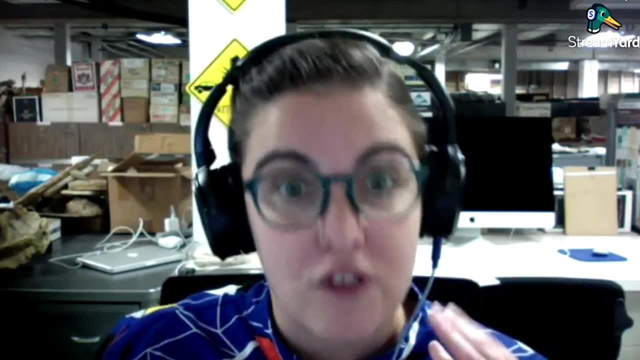 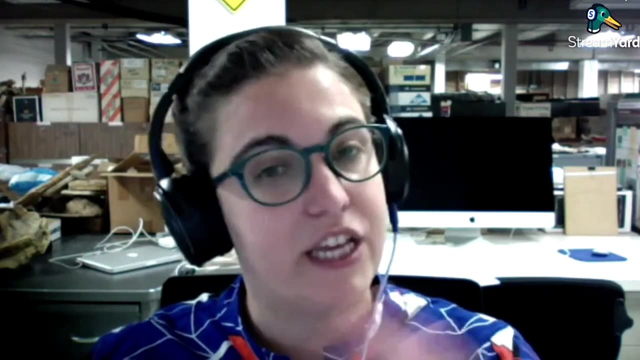 I wanted to study mammoths. That's what I thought that I wanted to do. I had studied plants and everything because I liked the whole environmental perspective of things, But I was specifically interested in mammoths. So in my undergrad I specialized in like paleo ecology and paleo. 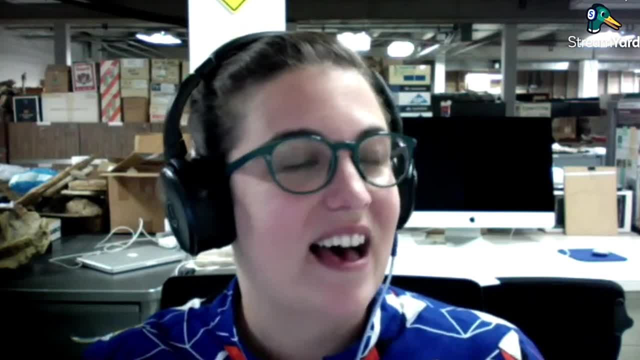 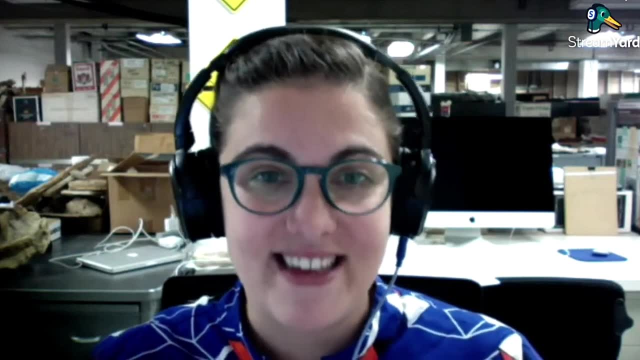 environment And I was like I want to be a paleontologist. And I was like I want to be a paleontologist But I did two different internships in South Dakota working on fossil mammoths, Like that's what I thought I wanted to do. And then I started my master's And when I 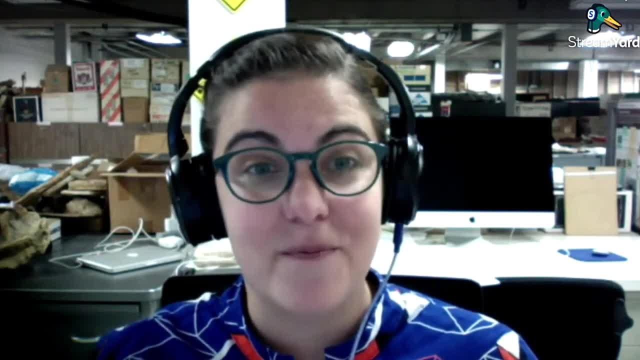 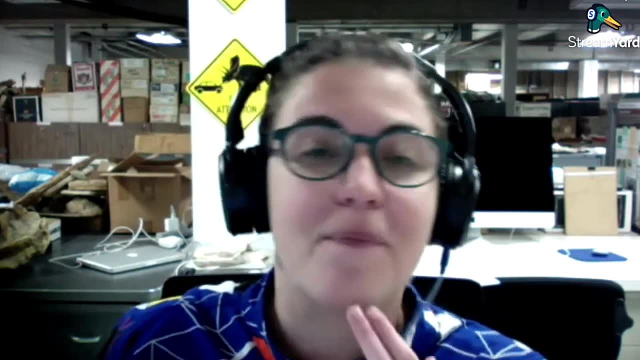 got there, my master's advisor said: so you'll be working on fossil plants, And I was very taken aback. I was like it's fine, A master's is only two years, Like I could deal with plants for that long. And then I realized that the questions that I was more most specifically interested in 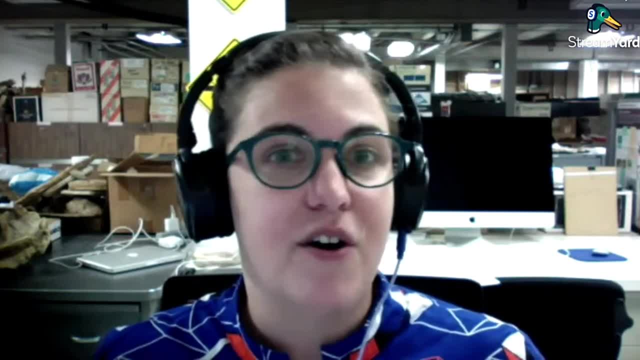 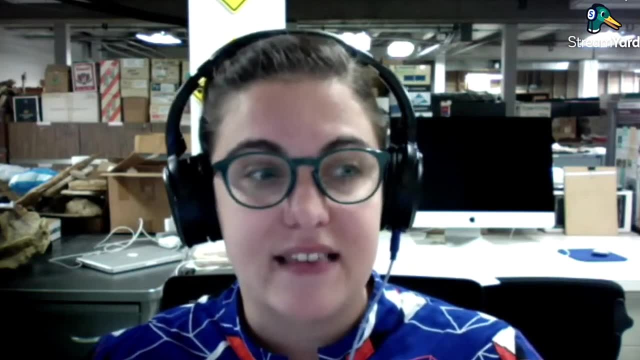 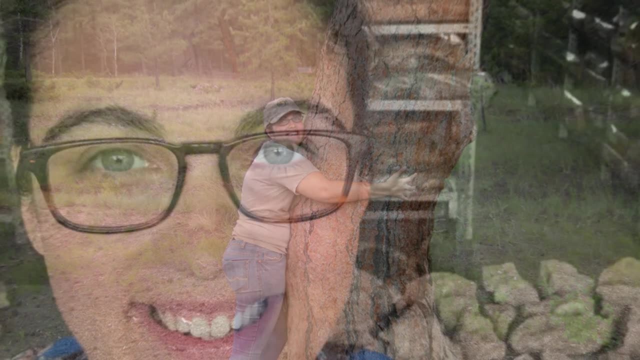 in paleontology were best answered with plants. So, even though I still have a soft spot for vertebrates and I have a lot of training in vertebrate paleontology, I realized that plants were the way to answer all the questions that I was really interested in, Because in undergrad I had taken- I had taken- vertebrate paleontology. 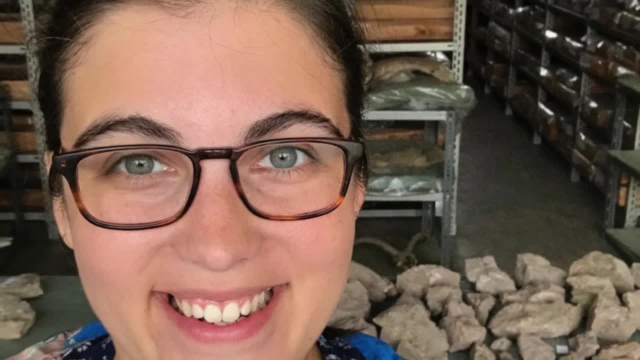 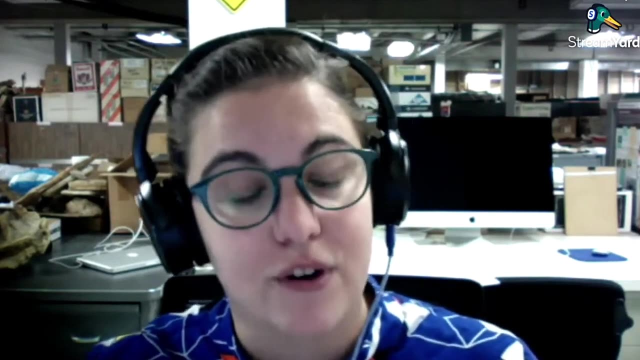 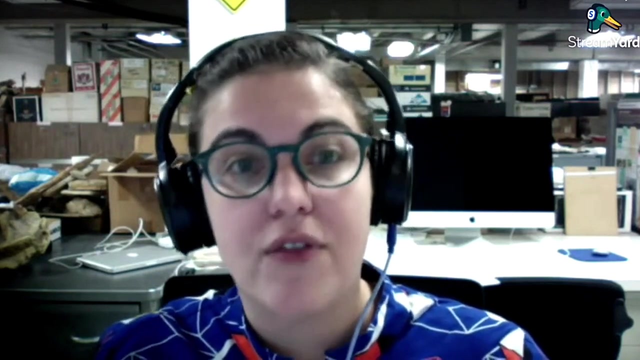 classes, but I had taken also more like paleobiology classes, So anything alive. I had also taken a whole lot of botany classes. I had taken these field courses in botany, So I was very comfortable with plants, more so, I realized, than many people are, And so that was part of the 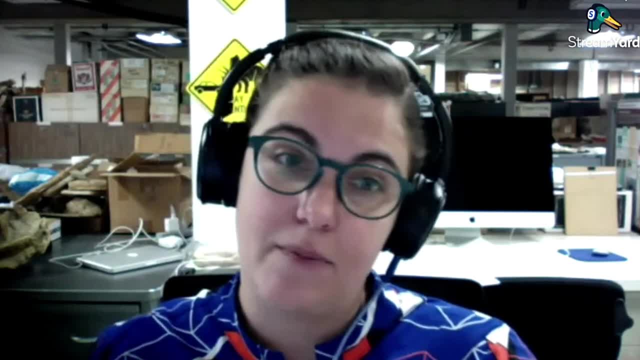 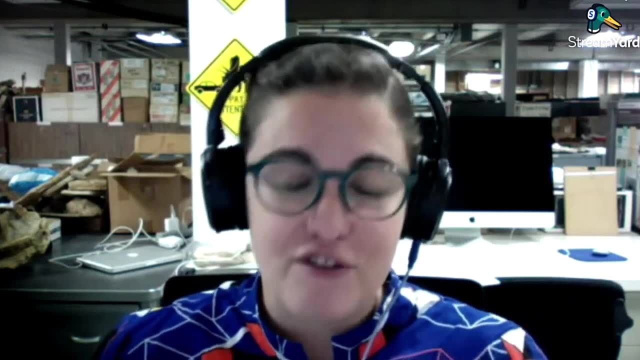 reason why, when I got to my master's, that my advisor was like: you're working on plants? It's because, even though I hadn't focused on them, I wasn't afraid of them, And so when I finished my master's, I realized, okay, I'm committed, Like I am team plant all the way. I've realized what I'm. 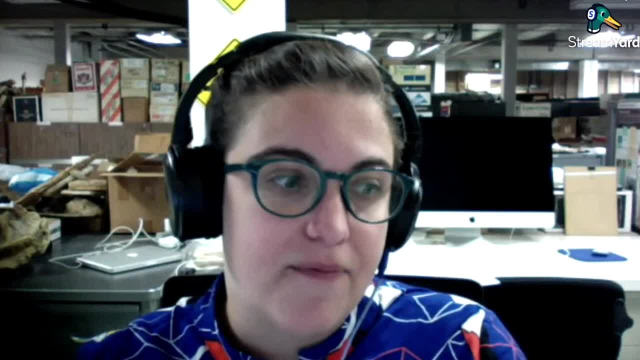 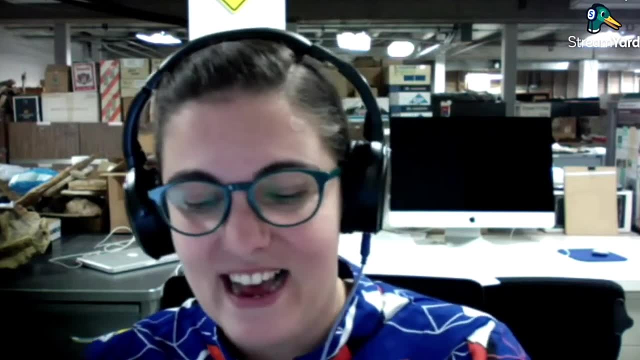 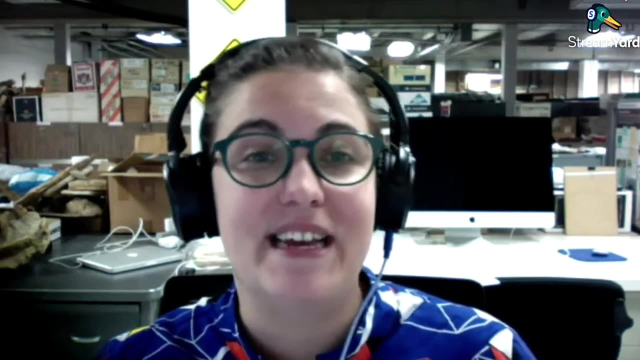 interested in And then. so when I did my dissertation for my PhD, I went all out from the beginning: this is what I'm interested in. But then, at the end of my PhD, I needed a job And, like I said, I have training in vertebrate paleontology but also invertebrate paleontology. 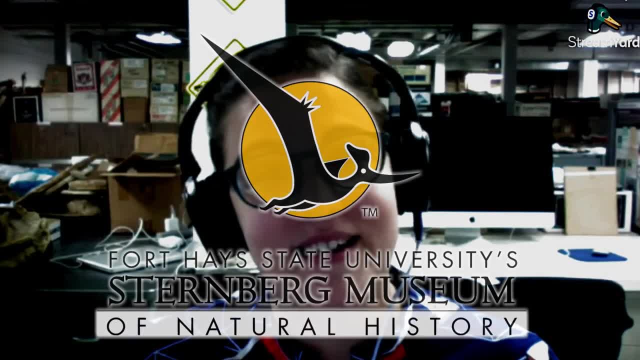 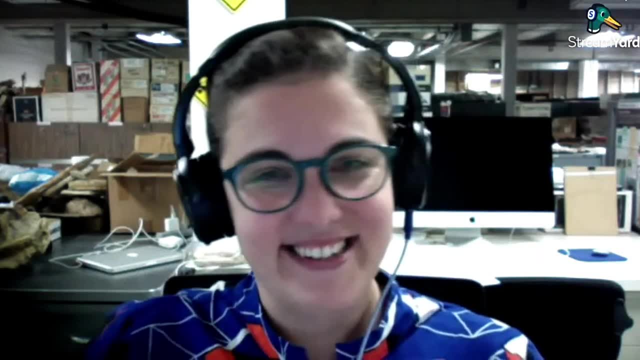 as well as paleobotany. So the Sternberg Museum needed a collections manager. It's like, hey, I can do anything, So I ended up here. Ellie, you are a paleobotanist, So I guess a good place to. 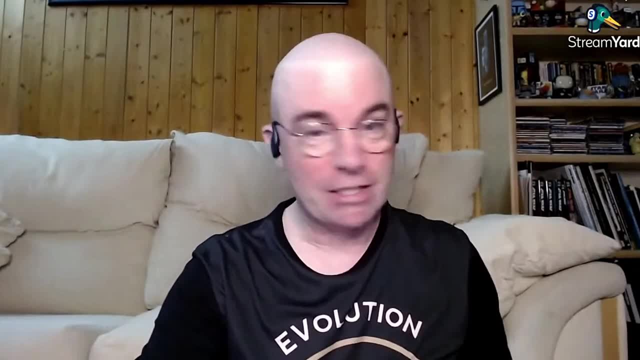 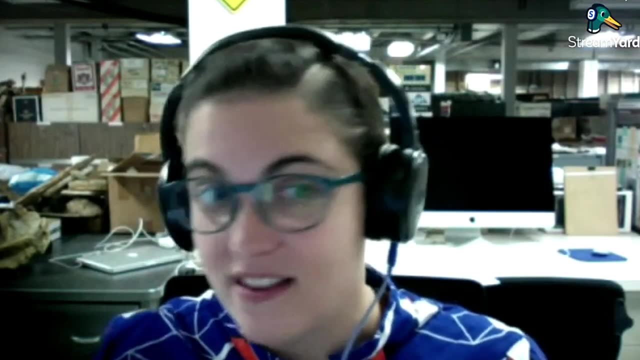 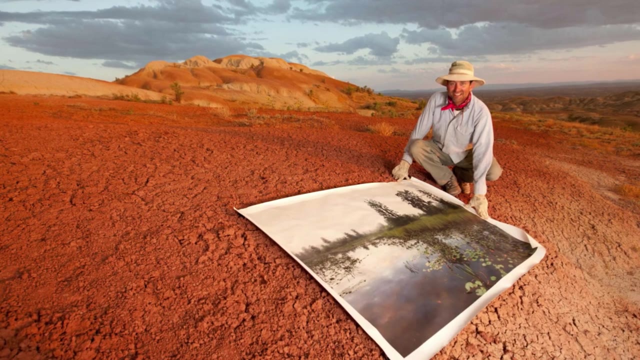 go is: what exactly is a paleobotanist And what do they study? All right, So in the most literal definition we study ancient plants, paleobotany, ancient plants. But that's unhelpful. That doesn't really describe what we do. 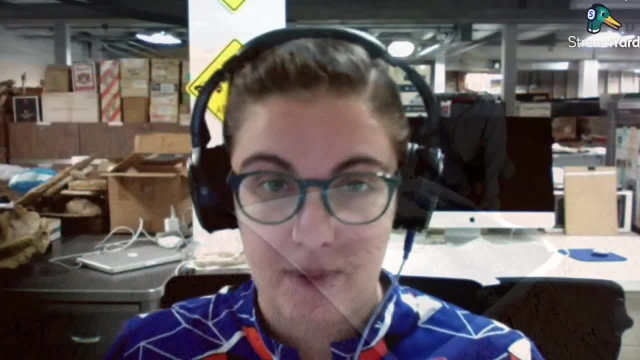 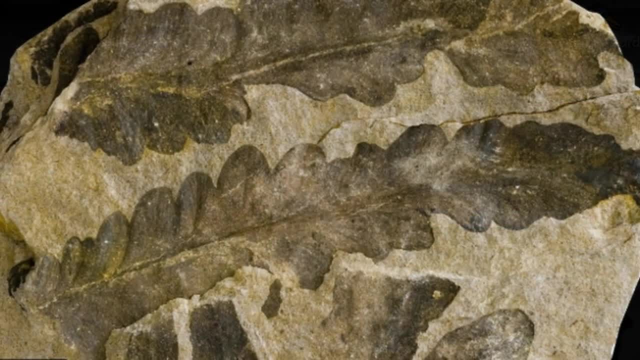 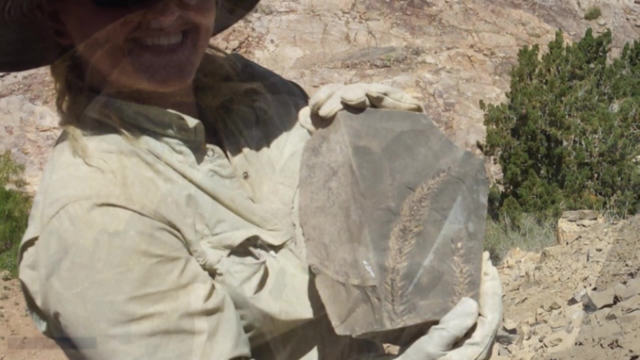 So, broadly speaking, there are two main types of paleobotanists, basically broken down into what you want from the plants that you're studying. There are the more taxonomic, systematic paleobotanists. So they will look at plants and they will try to actually identify them, figure out who they are related to. 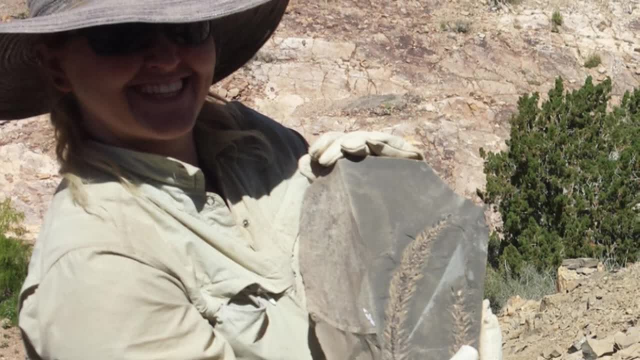 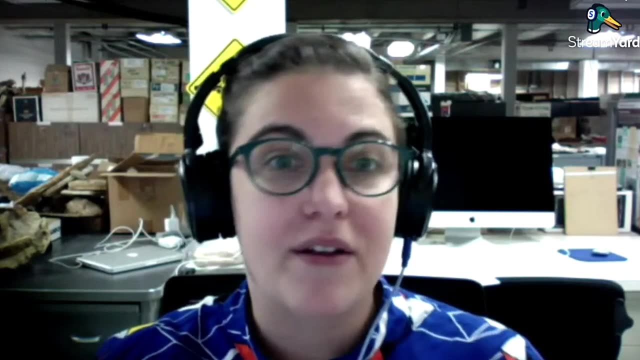 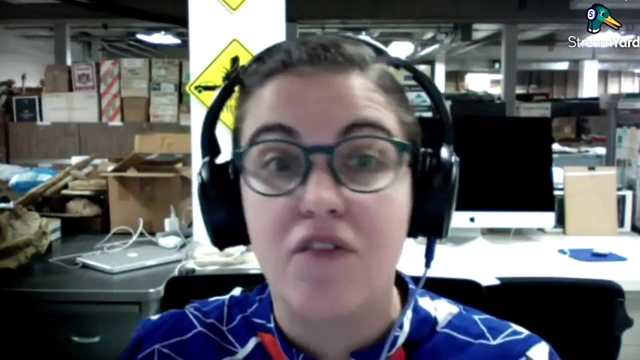 so that we can understand the history of life in that way, understand these family connections and where these groups originated, when these groups originated, things like that. So that is one way of coming at paleobotany And it's very important. 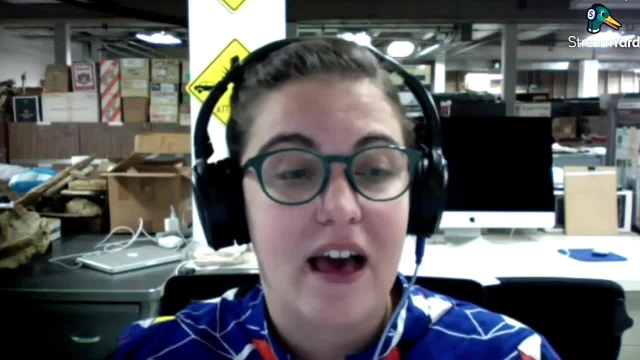 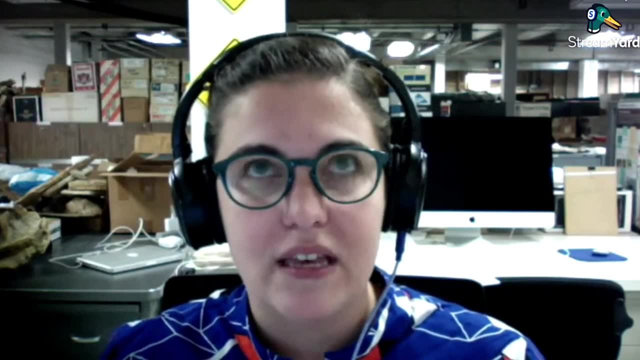 That is not the flavor of paleobotany that I do, though. So the other half of us, I would say, are the ones of us who are less concerned with the identity of the plants. I don't need to know what species it is. 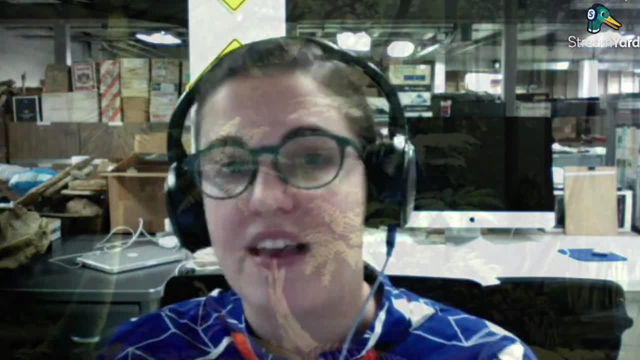 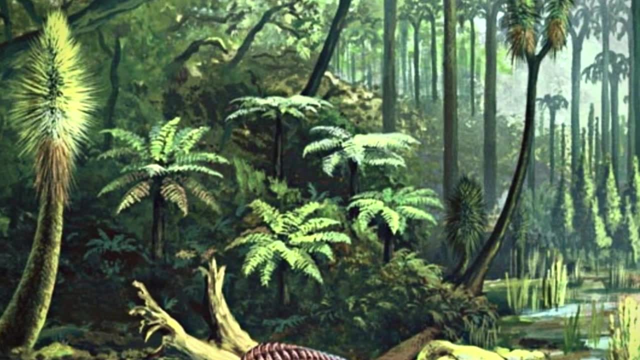 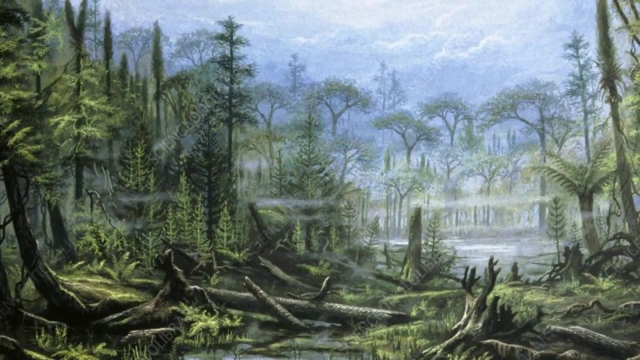 but we can use plants more of as a vessel, as a time machine for understanding the broader environment. So either the paleo environment, the paleo climate, the paleo ecology, where it doesn't necessarily matter the precise affinities of the plants themselves. 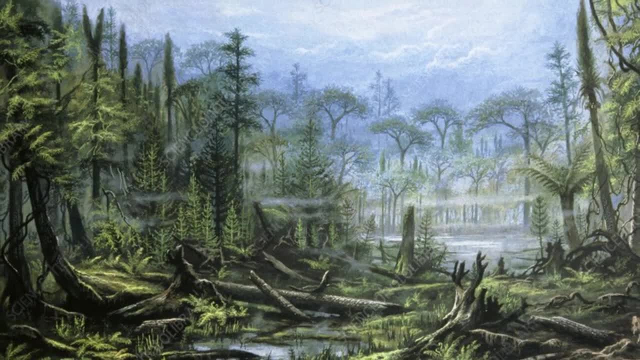 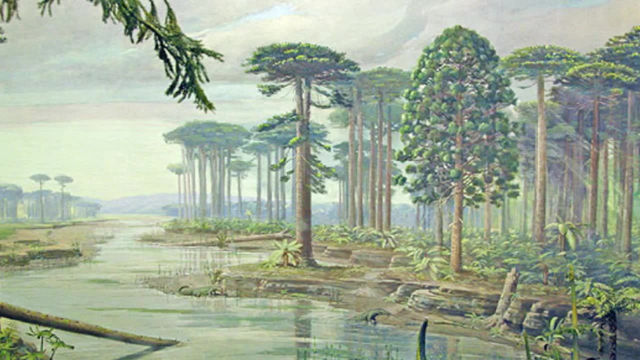 but, more broadly speaking, we can understand the bigger picture, So understand things about how CO2 has changed through time, how temperature has changed through time. So both of these parts of paleobotany are very important and they are important to each other. 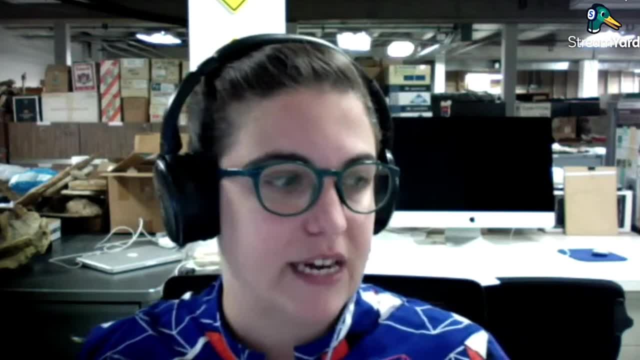 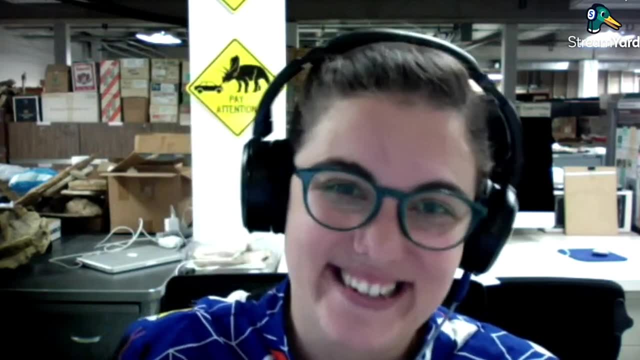 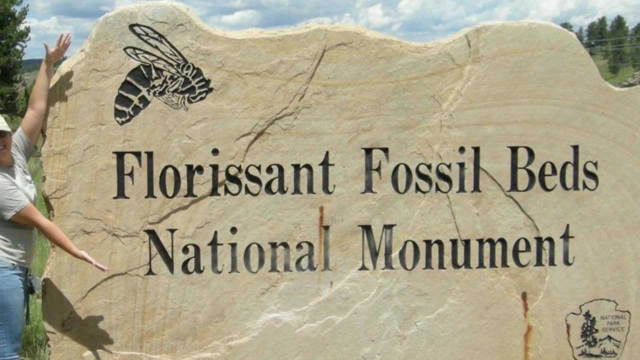 They're complementary, but they are kind of two different ways of being a paleobotanist, So you're kind of a plant-time traveler. Yes, I think you've called yourself that before. Yes, it is one of my favorite ways to refer to myself and what I do. I am a time traveler. 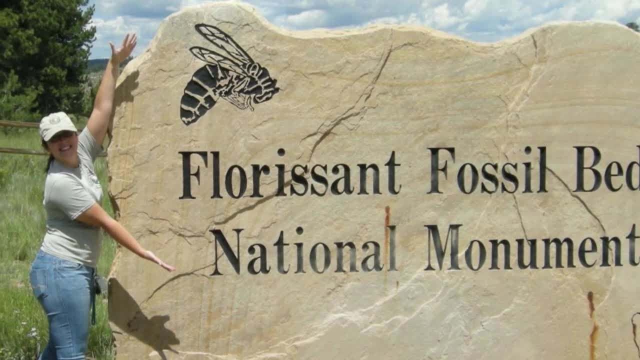 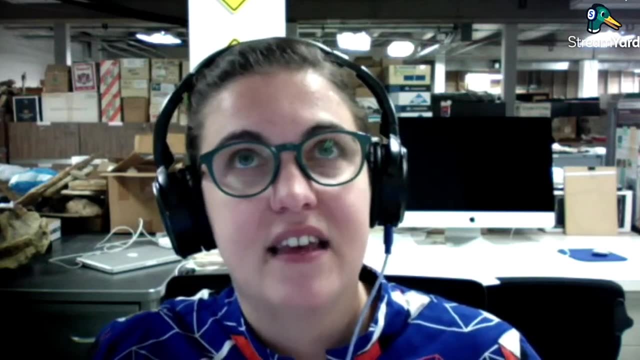 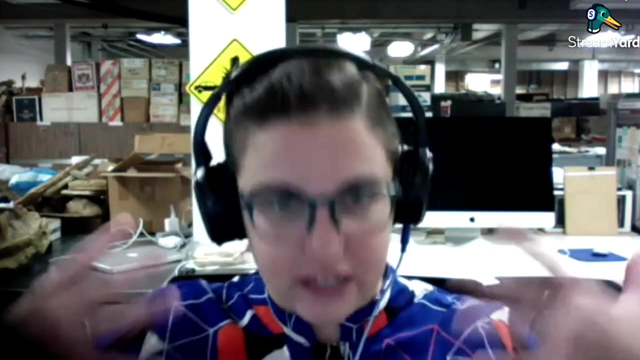 What I do is time traveling. I think it's a good way to really help people understand what I do, because the thing about time traveling is that you're using all of your senses right Like if you were to get in a time machine. 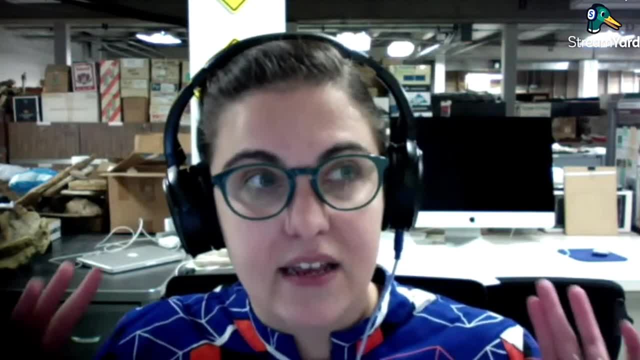 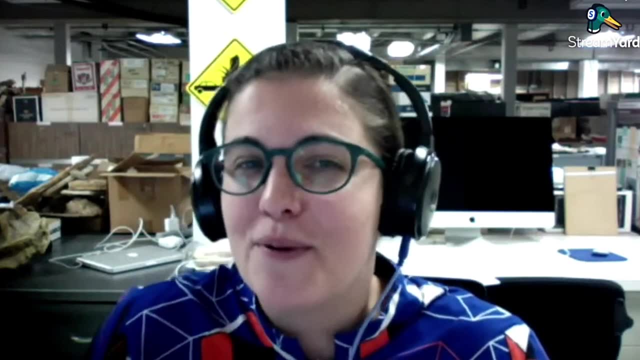 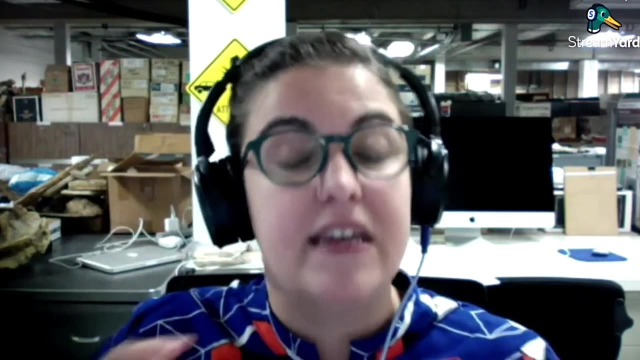 go back in time, go forward in time, whatever. The difference between that and- just like I don't know- seeing a picture or watching a movie is that all of your senses are engaged. And that's kind of what we're doing with this kind of paleobotany is we're trying to engage as many parts of the environment. 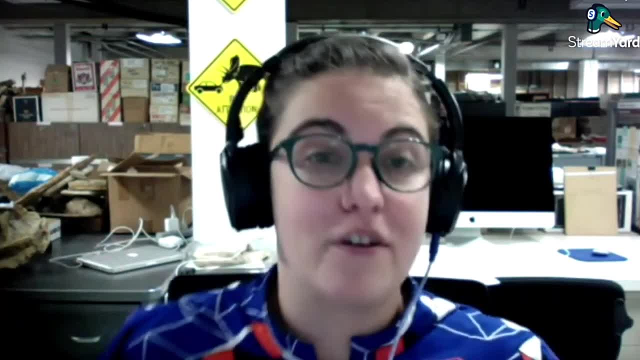 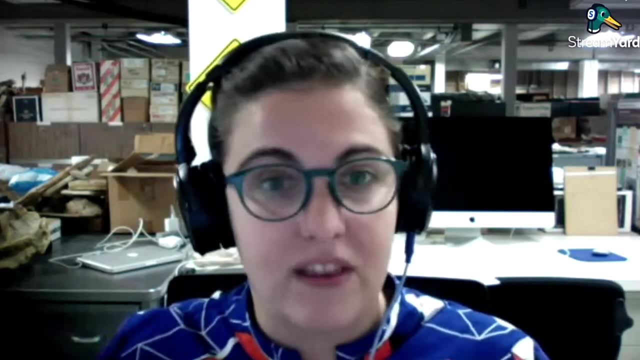 as we can. We can make it three-dimensional understanding, a four-dimensional understanding, because we're going through time And it's more than just this was here, Like no, no, no, this was here and this is who it lived with. This is what the 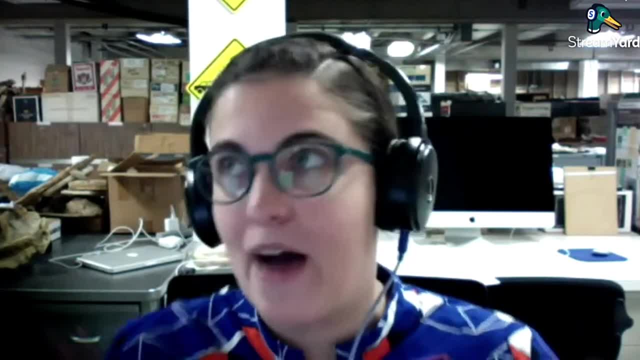 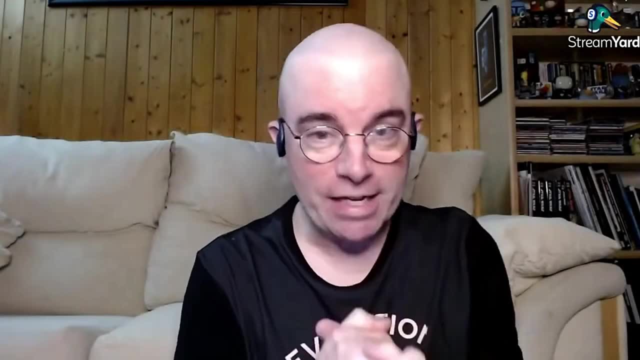 how warm it was, how cold it was, how rainy it was, how much CO2 there was in the atmosphere. Just trying to get a much more complete picture. Okay, let's begin at the beginning. the origin of plants. How far back do plants go, and? 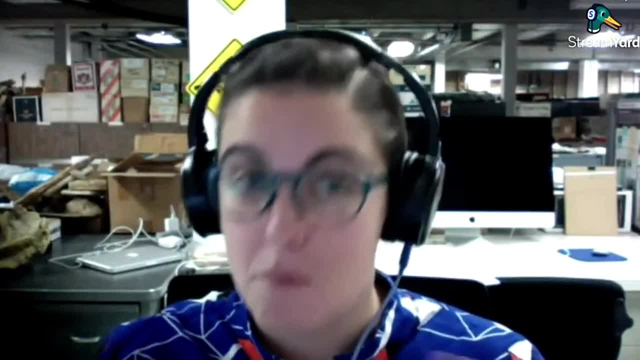 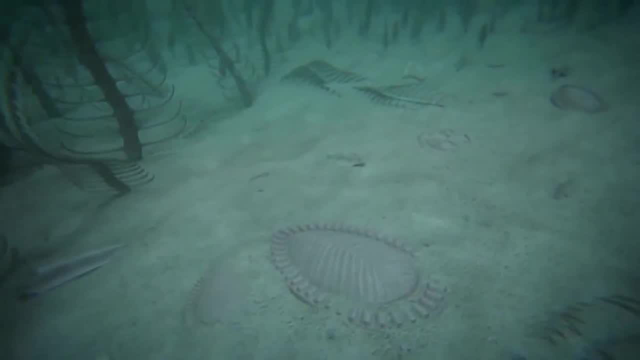 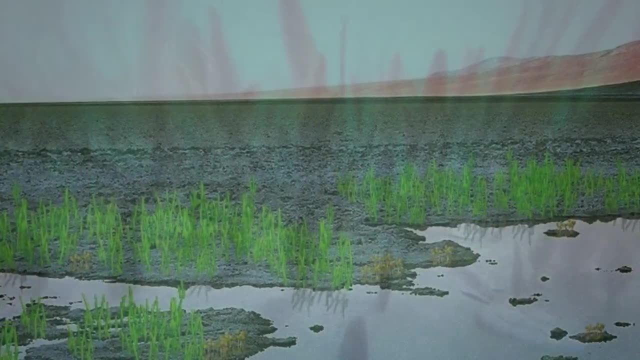 how do they evolve? Alright, so, like most life on Earth, they had an aquatic origin, So they did not originate on land, but they got there pretty quickly. So as of now, our understanding is that there were at least some plants on land in the Ordovician. 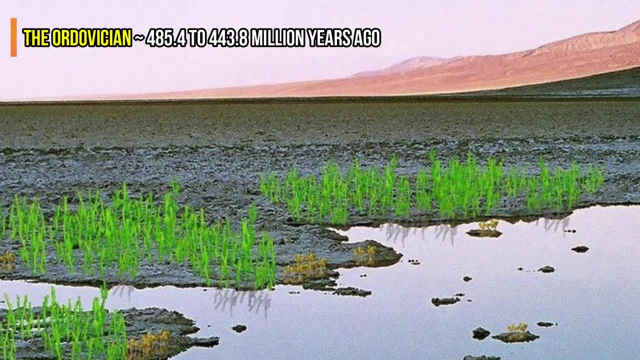 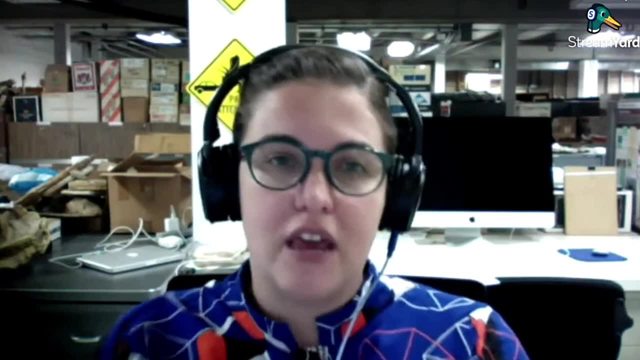 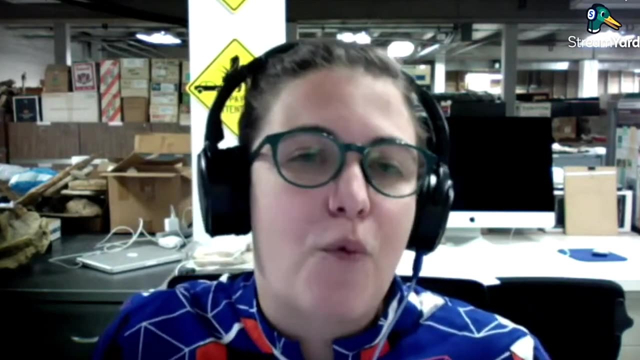 And we keep pushing when in the Ordovician further and further back. So it used to be that, oh, it was the late Ordovician And now it's like, well, maybe it's actually the middle Ordovician. So they, the earliest plants, were related to aquatic things that we would now probably. call algae. We would not. we probably wouldn't actually identify the ancestors of early plants as plants. So when the plants came on land they were most similar to bryophytes and ferns and liverworts and hornworts and those little things. So these are. 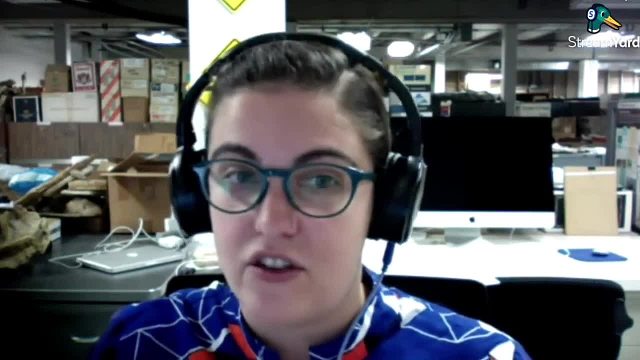 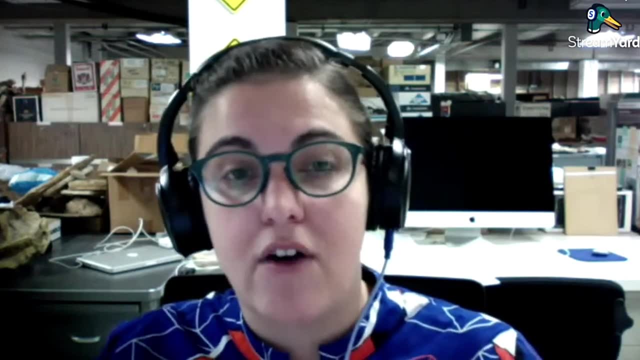 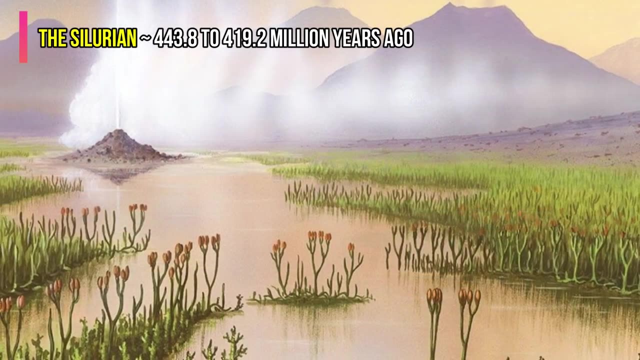 spore plants. they don't have seeds and they are non-vascular plants So they don't have- basically don't have- tubes in them to move water or nutrients, So they are very low to the ground. Some of the reconstructions I have seen of these early like Ordovician and Silurian environments are basically moss swamps. Because nothing was very tall and they were pretty restricted to wet environments. They weren't getting very far away from, you know, streams and lakes and things like that. They needed to be close to water. It just seemed like moss and fern-like plants ruled the world for a long time. Oh yeah, Moss like moss are the original life on Earth, Like their life on land, at least Like it's moss. You need to respect the mosses. But it didn't take long for plants to really come into their own. 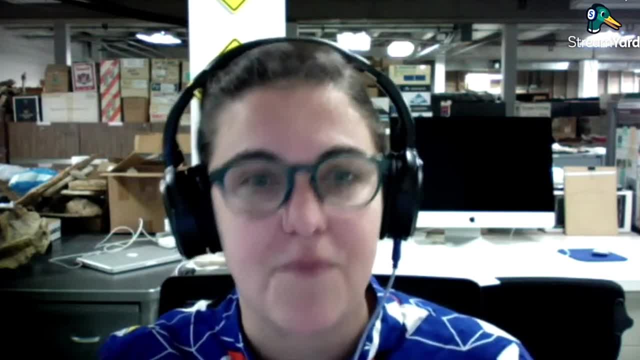 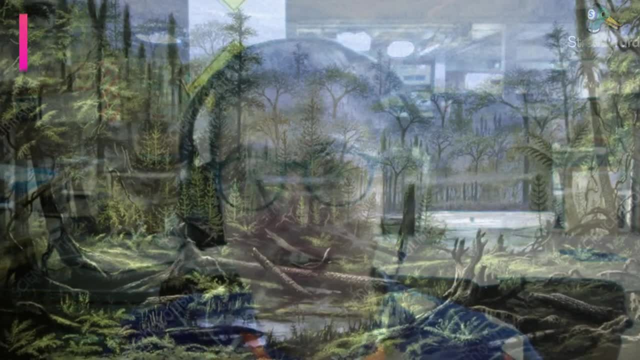 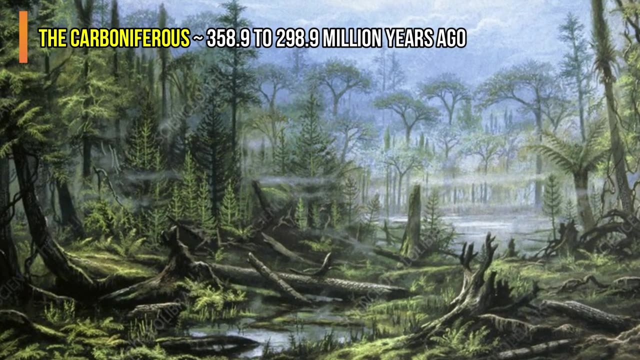 So you have the Ordovician, and the Silurian is mostly mosses and the like, And then, by the time you get to the Carboniferous, you have trees. So so they are mostly related to ferns, but you have trees You would. you would recognize it as a tree. You might not recognize a tree that looked like that A lot of. when I was taking paleobotany, my professor would always describe the Carboniferous forest as looking like a Dr Seuss forest. Because, like the shape of the trees is completely different from what we're used to with gymnosperms and angiosperms, today The, the ferns, aren't shaped like that, But because plants had all this time: they had the Ordovician, they had the Silurian and then in the Carboniferous, by the time you get to the Carboniferous, like plants have established themselves, And they basically terraformed the world in a way that made it habitable for animals. So plants aren't the only thing that are pumping out oxygen. So they take in CO2 for photosynthesis and then they release oxygen as a byproduct. They're not the only ones doing it, but they are. 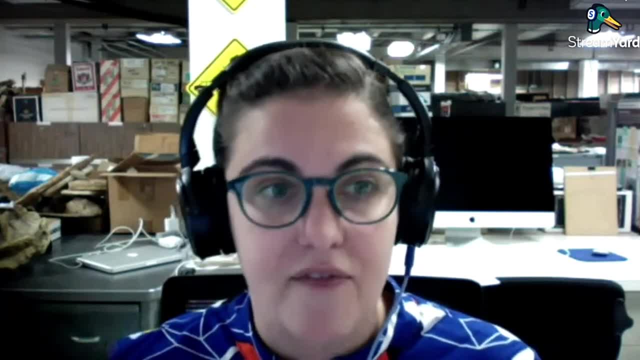 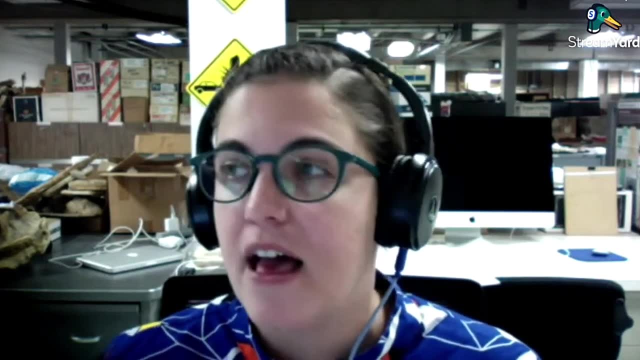 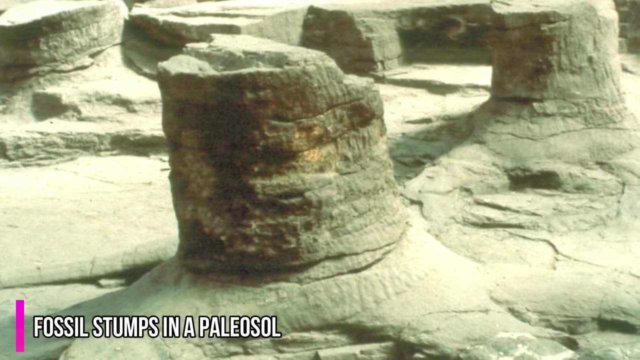 major players doing that. So you have this, this change to a very oxygen-rich atmosphere during the Carboniferous, And then, in addition, one of the big arguments in actually paleopodology, so the study of fossil soils, is whether you can have soils without plants. 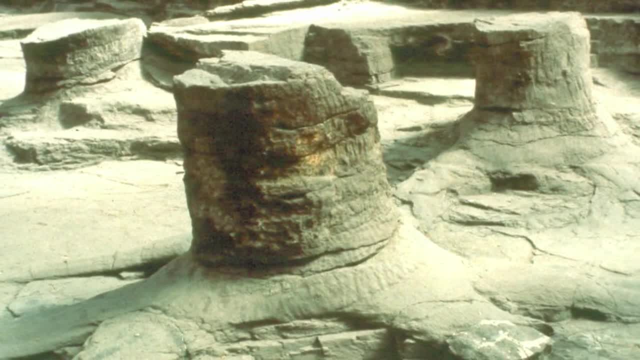 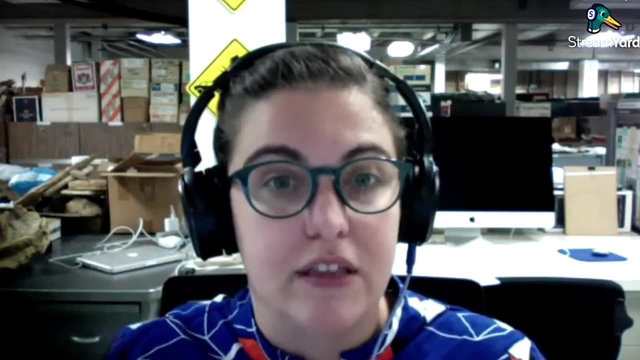 Because plant roots in plant like bio-turbation, moving of the soil with their roots and, you know, pulling nutrients out of it, altering the soil in that way. Can you have that without plants? So this combination of changing the 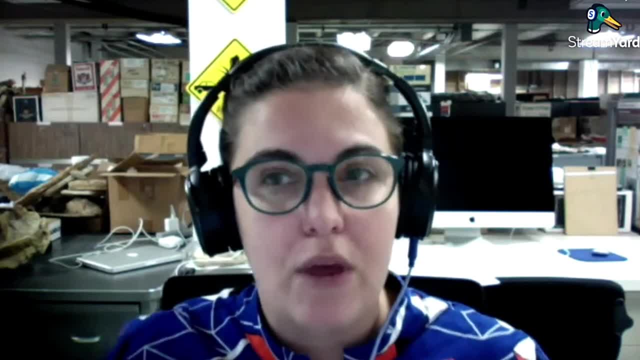 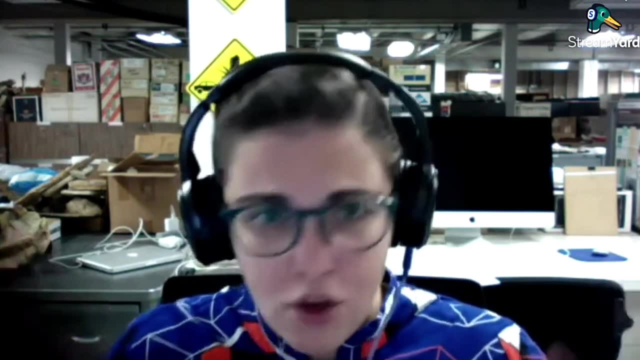 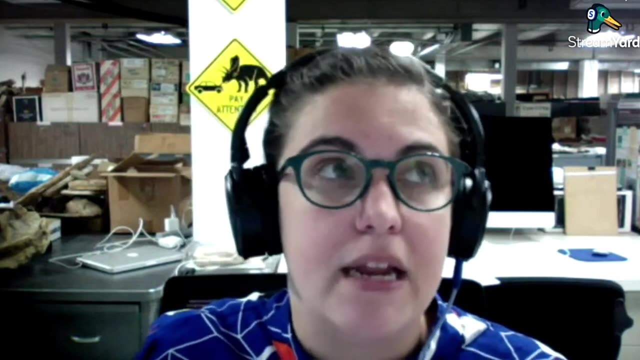 literally changing the the world, literally changing the environment with these more complex root systems, with the way that they interact with water and nutrients. Also, trees- um they they're dropping leaves. that is reintroducing nutrients into the environment. there are radiations of fish during the Carboniferous because there 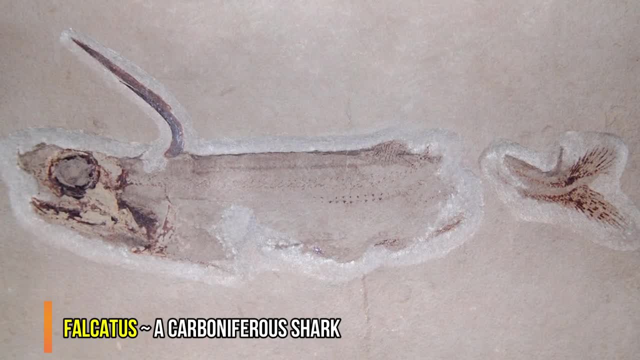 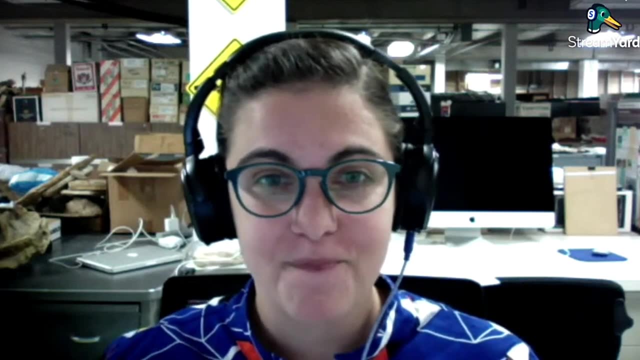 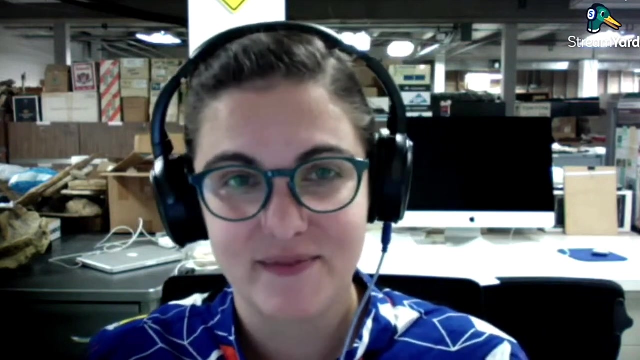 are so many nutrients in freshwater environments because of these trees, and I suppose it's bit of a paradox because we think you need soil, but soil, as far as I know, comes from degraded plants and leaves and things. but what? what were these trees sitting in? or these early ferns sitting in before there was soil? so if you think about before the ferns, with the more complex root systems, you have mosses, and mosses don't really have much of a root system at all. if you think about mosses, they will happily grow on a rock they don't really have. any roots, so they're not going to. they don't need soil per se, but over time you have the, as you have these plants with more extensive roots. you know, plants are really good at breaking down rocks. that's. that's what they do physically and chemically, and so that's. 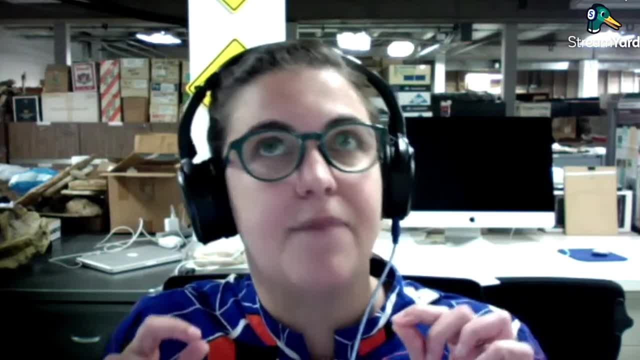 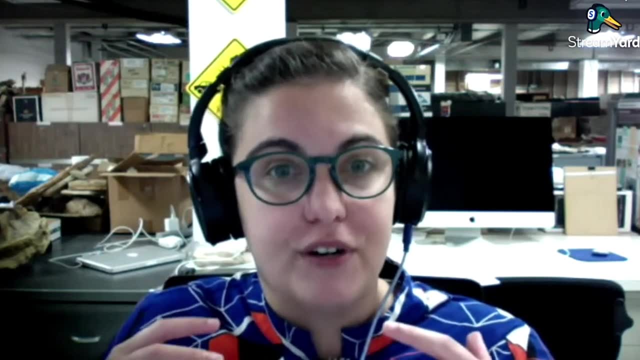 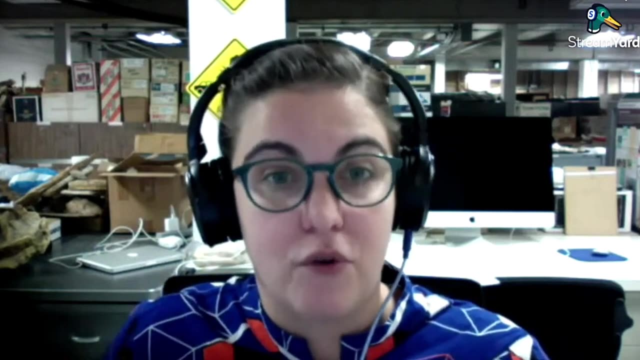 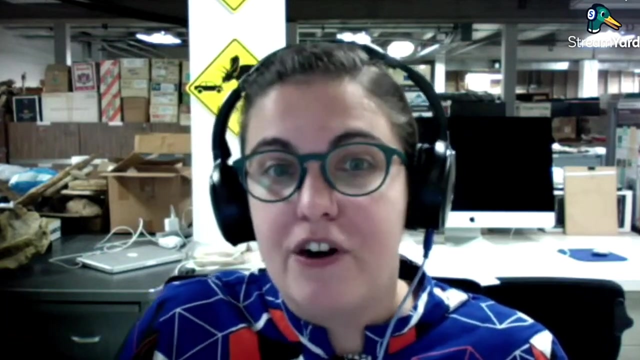 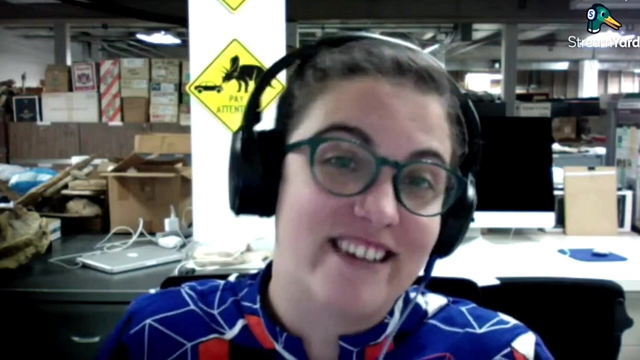 the change you see, like the depth, because basically, like, as plants are physically able and chemically able to alter the parent material, whatever the rock that they're there, they're on, and then you begin to form soils. so basically, you had a moss on bare rock to tree ferns with actual, recognizable soils. honestly, after not very long geologically, and just out of interest, if you were to time travel, to say the silurian or something, you wouldn't last very long without an oxygen, the right kind of oxygen to the breathing apparatus, right, exactly because there wasn't really really have life on land. it wasn't really habitable for animals on land, um, so yeah you. would need like full-on diving bell, diving suit. you know you're, you're functionally going to an alien planet. if you go to, if you time travel to land before the carboniferous, you are going to an alien world. it is not going to look like anything that any human alive is used to in any 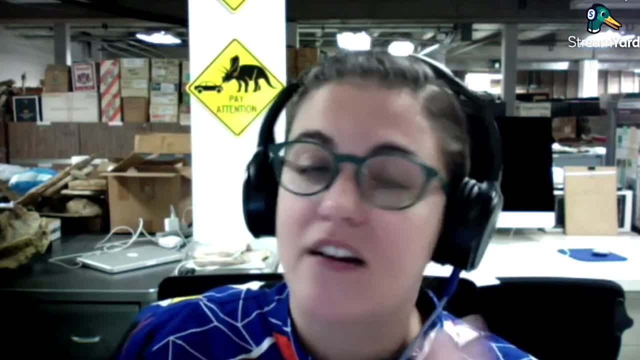 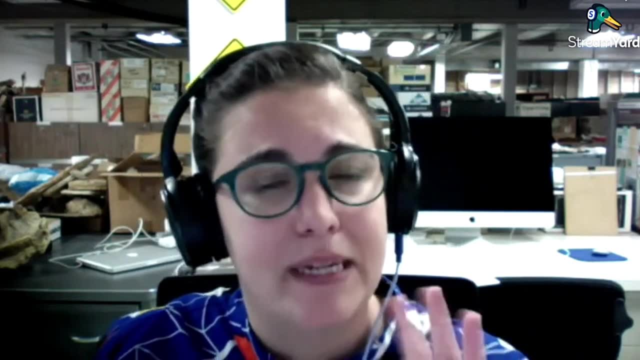 way, the carboniferous is weird, but it's recognizable. right like there are insects, there are early um, like amniotes. there are animals that we would recognize and the plants look, i don't know, vaguely plant-like, but in the silurian and ordovician, and especially if you 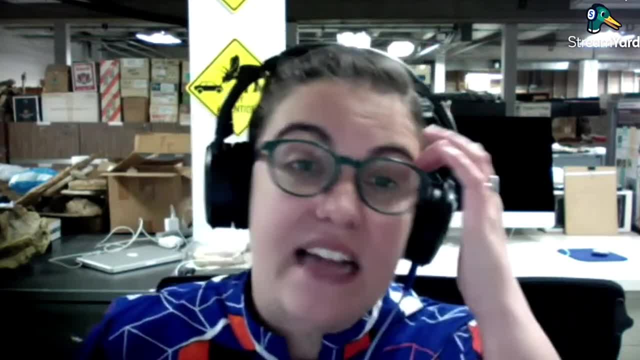 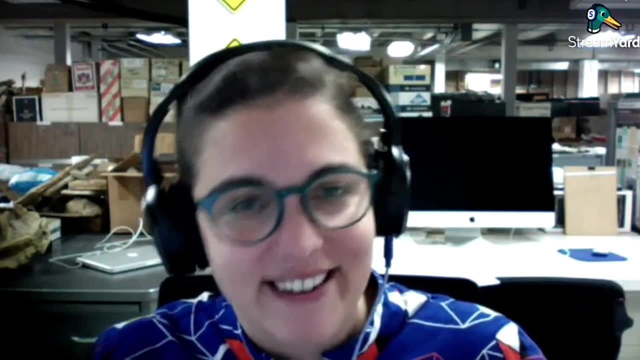 went back to try to do sci-fi. i'm a man, yeah, exactly, exactly it would. it's kind of like being on the moon, right, like i mean, a little bit there's water, uh, maybe more like being on water on mars: there's water and there might be like little crusts of moss and stuff, but 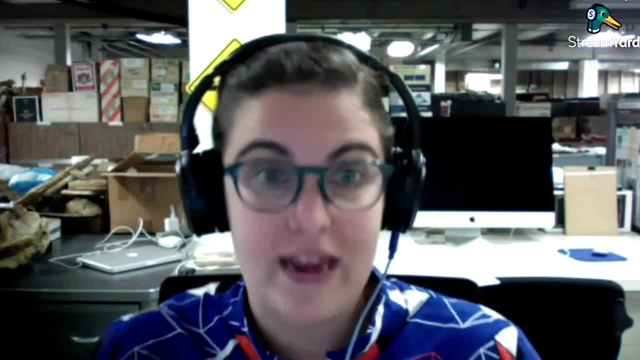 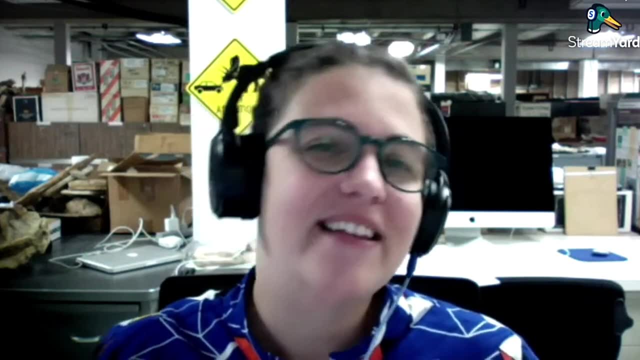 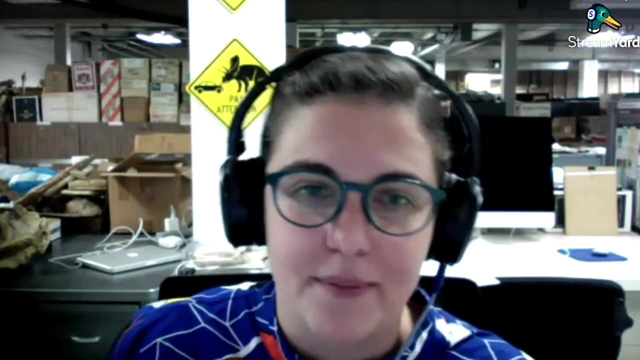 it's completely different from any world that we know now. am i right in saying that plants ruled the world longer than animals have? oh yeah, well, it depends on your definition of the world. if you mean like the planet, no, we've been here about the same amount of time. um, still, yes, but the plants got on land first, i see, and and were there any mass extinctions of plants? we think of mass extinctions of animals, but did plants have any or or none at all? okay, so this is actually incredibly contentious in the paleo body community. oh no, no, it's, it's, it's really. 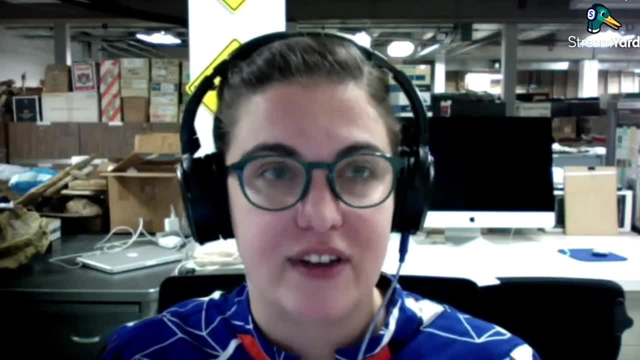 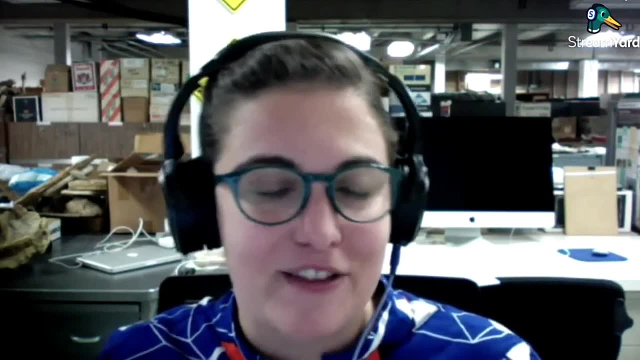 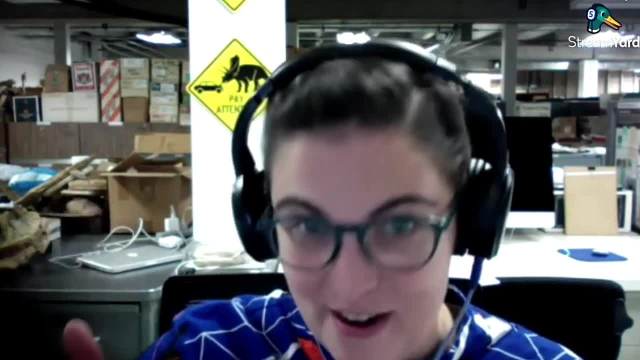 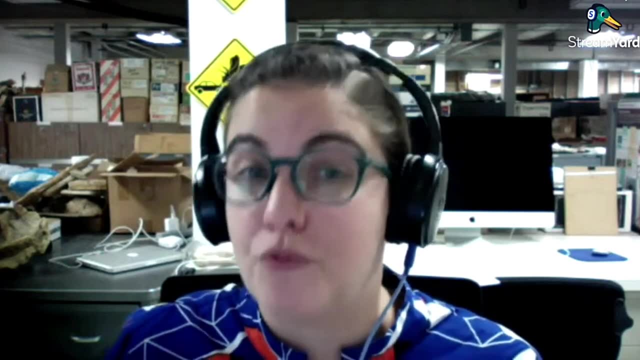 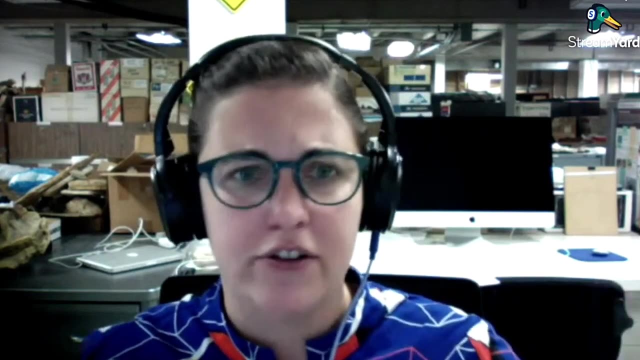 then the end of the, the mesozoic. again you've got this terrible mass extinction. but our understanding of mass extinctions are based on actually primarily marine animal life. uh, so we're, we're talking primarily about marine invertebrates, particularly the older ones, the- uh, the first. 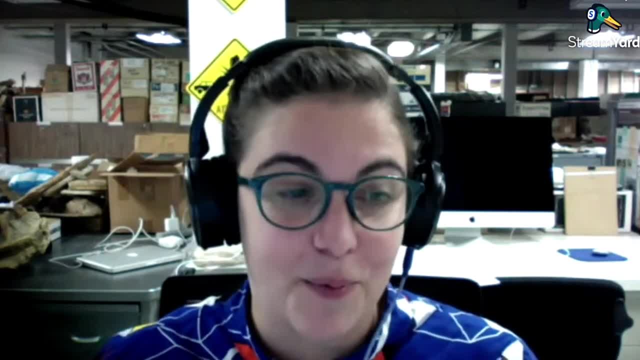 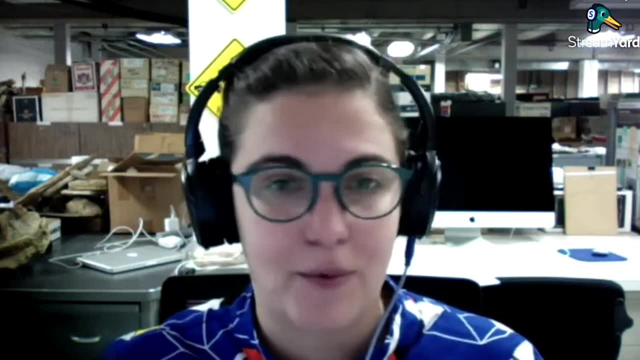 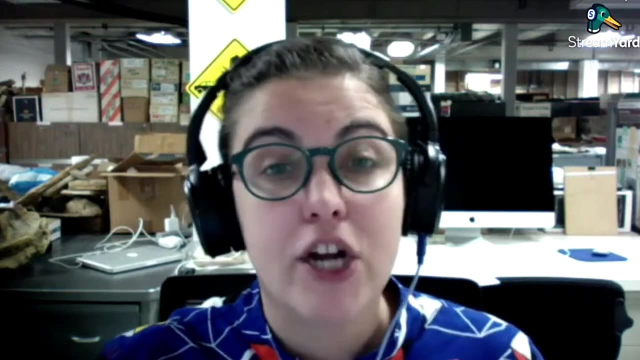 couple, but plants first of all. uh were not on land until sometime in the ordovician, so anything going on before you know the end of the cambrian, they were not on land. um, but in general plants just have a yeah, so it depends on where you're looking, but yeah, in general plants have a different relationship with the world. than animals do, because plants are photoautotrophs, so they are using light from the sun to make their own energy. most animals are are heterotrophs. they are taking in energy from something else, um, so that that difference in energy source is one of the reasons that they are affected differently in terms of 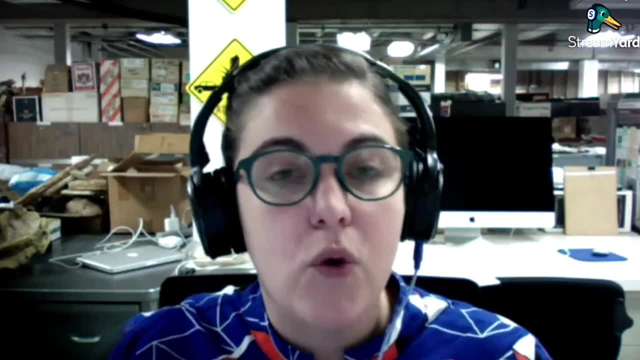 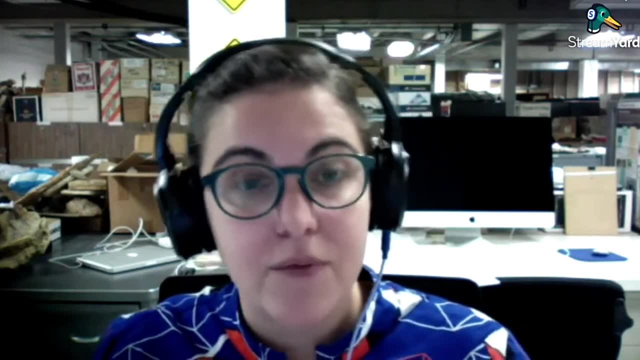 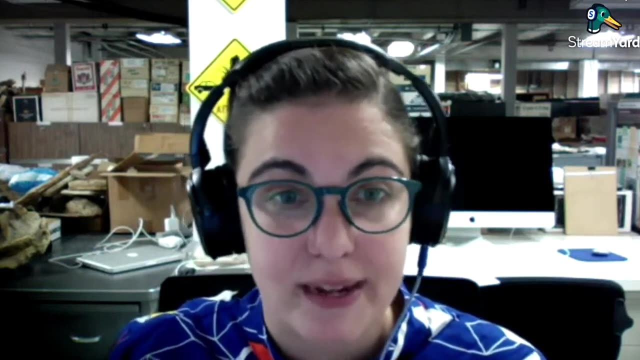 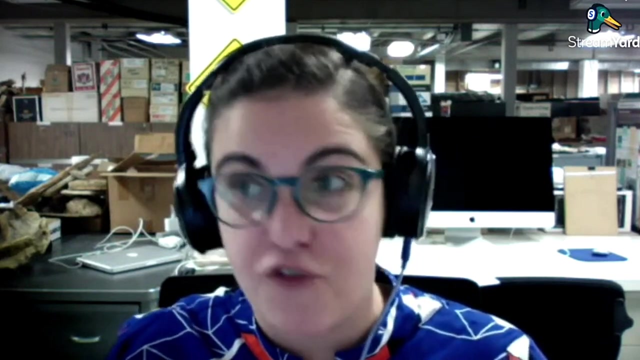 mass extinctions. so there, if you were to base the geologic time scale on plants instead of animals, it would look fundamentally different. and, as far as we can tell, some people say there have never been a mass extinction of plants. most people agree there have been at least one. um, but like that is fundamentally different than understanding. 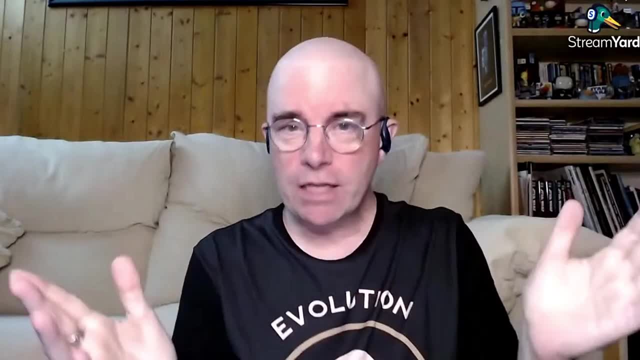 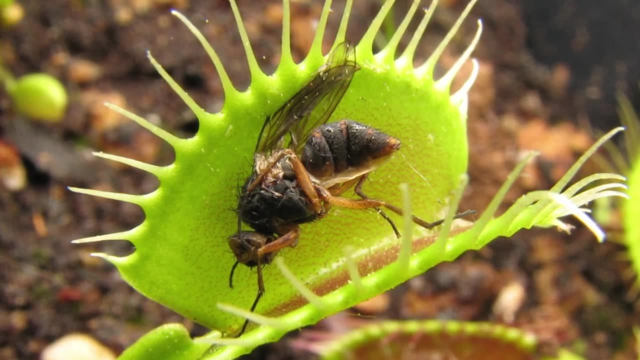 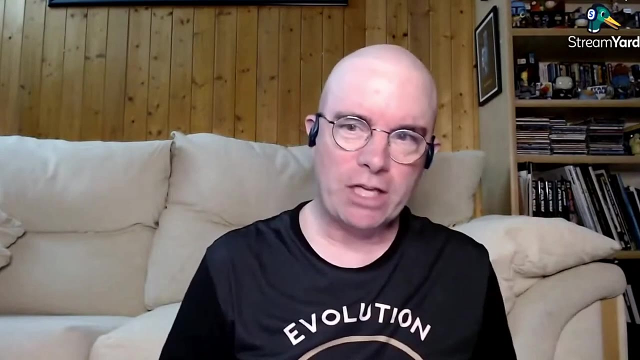 of mass extinctions for animals? well, plants have evolved and diversified in many, many ways. carnivorous plants have always been a fascination for people, feeding on insects and other creatures. there isn't a great fossil record to work from, though, but what do we know about the evolution of these various species? how did plants learn to eat bugs? so everyone loves carnivorous plants. you know it's it's plants doing its best animal impression. so that's a really good question. there are- and it's complicated like there are- so many carnivorous plants. there are much more. there are many more types than most people probably. 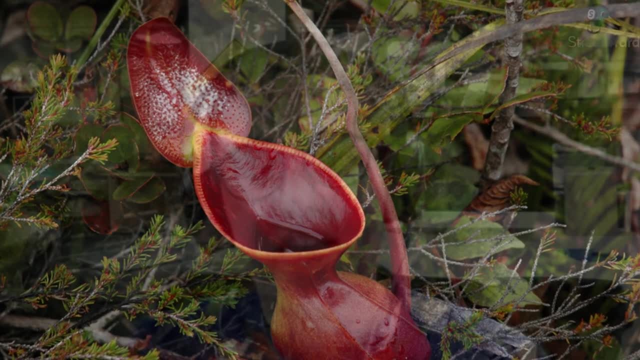 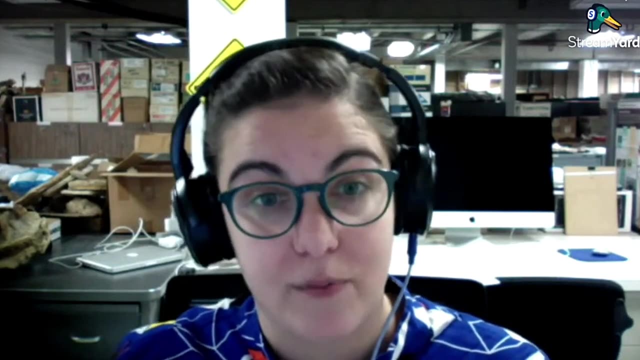 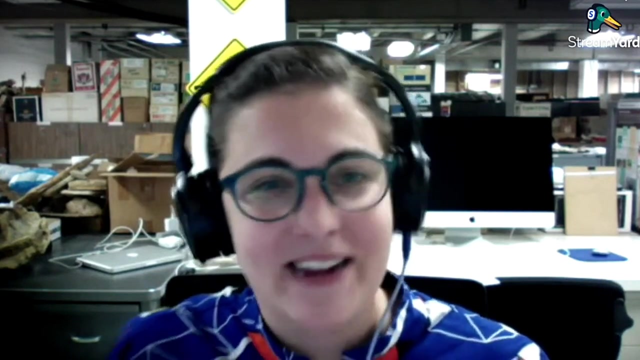 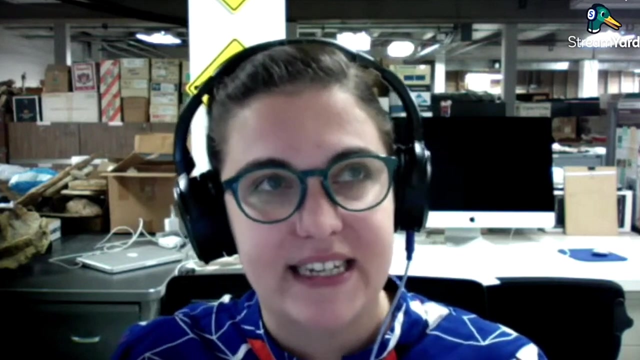 realize: um, the cool thing about it is, carnivory has actually arisen in plants, in the first plants, at least nine times in five different orders of plants. right, so that means that this is not it's not uncommon, like it's not super common. it's not uncommon, it keeps happening and they keep doing it in a kind of similar ways. 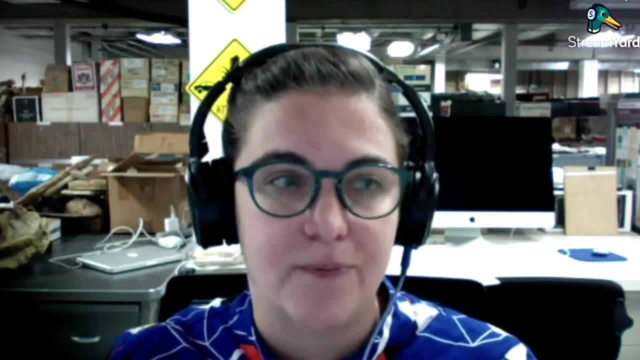 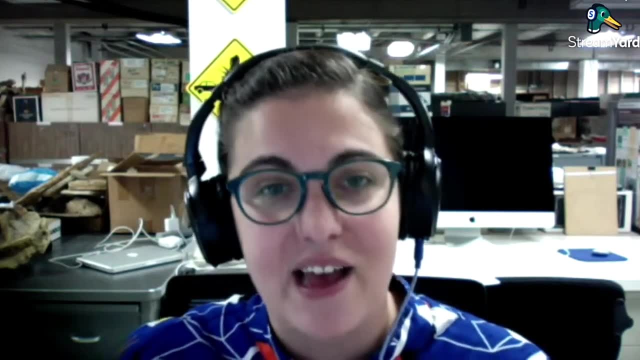 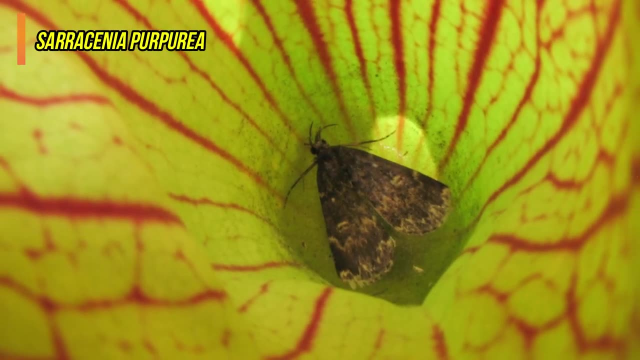 one of the things that's really common is the fact that plants will repurpose enzymes or report purpose secretions to turn them into these things that allow them to absorb insects so they can eat them, because this is similar to what snake snakes did. yeah, kind of yeah. so because this is not a real group, this is. more of a shape and so not all carnivorous plants. you know they're not all related to each other, they don't share common ancestors, so they've done this multiple times. so basically every different group has some sort of enzyme, has some sort of secretion, because a lot of plants have like either nectar in their flower or nectar in other places on the plant that they're able to kind of change in some sort of little way. um, but yeah, so we think of, we kind of think of carnivorous plants as being like, yes, this is a. plant. it eats insects. there you go, but they are parts of their, their ecosystem. so it's actually more complicated than that and they are ecosystems until themselves. um, so you have like insects that will steal insects that have been caught by like venus flytraps out of the venus flytrap, um for pitcher plants. 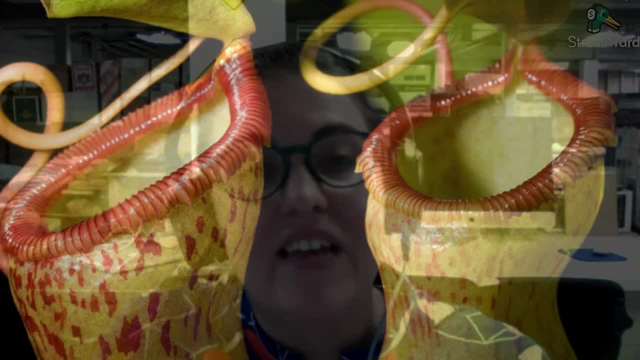 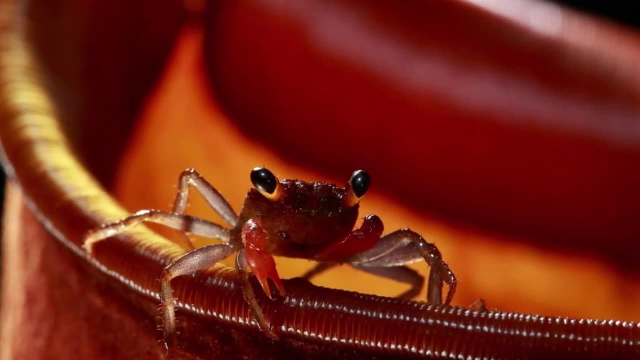 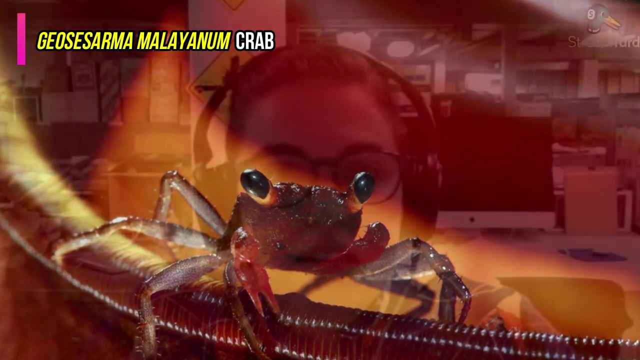 there are entire faunas that can live inside of these giant pitcher plants, so there are species of crabs that are known only from the inside of pitcher plants, and, I think, Indonesia, um, so yeah, these are complicated organisms that all did this independently, and then they're like you know, they're like you know they're. 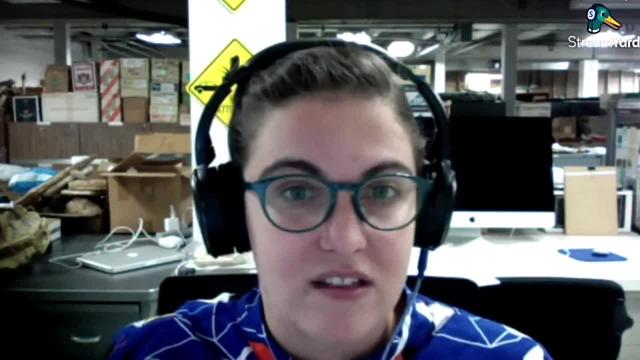 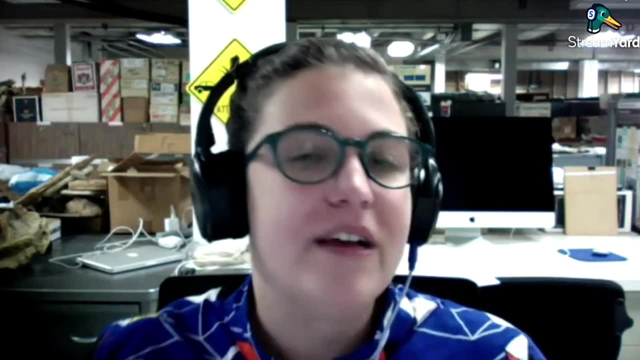 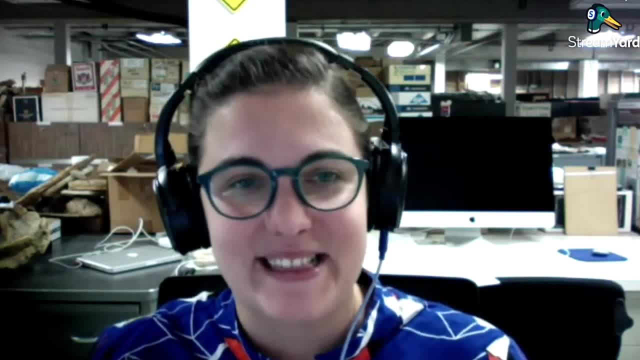 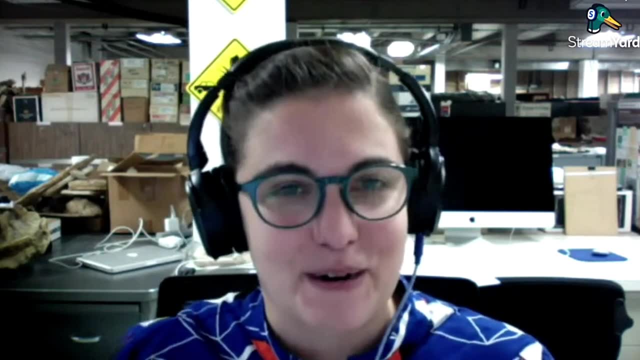 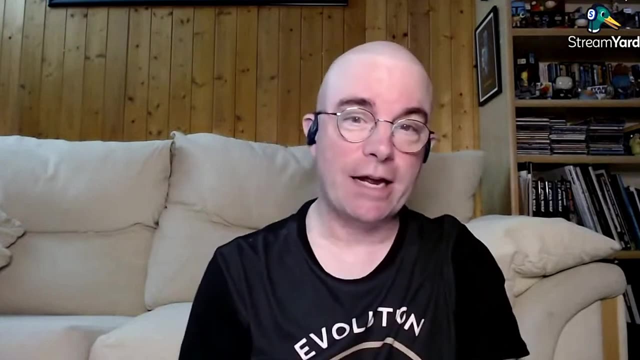 plants but don't necessarily eat the insects that they kill. so they just kill the insects and then don't eat them. those are, those are, strictly speaking, the murder plants. well, people may not be aware that there are a few living fossil plants alive today. I'm thinking of the 9,000 year old spruce tree located in 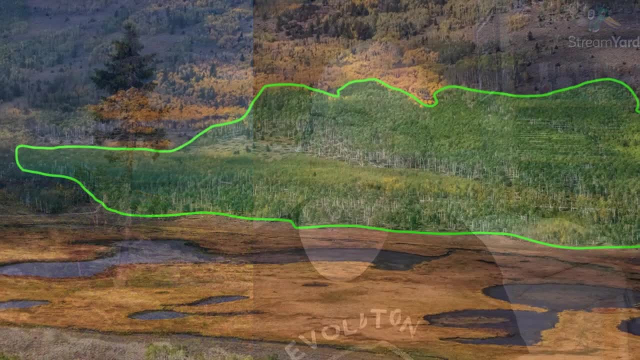 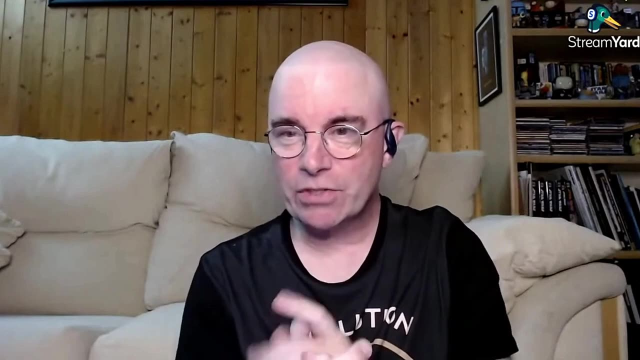 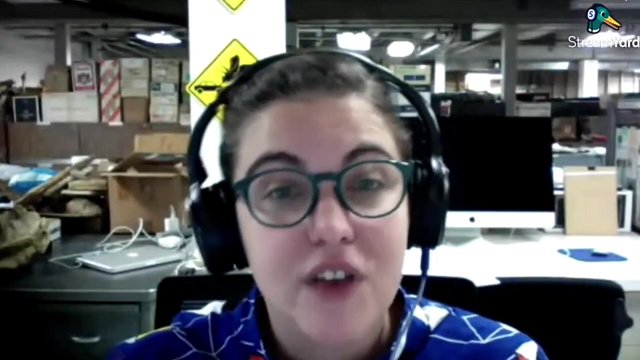 Sweden, Old Chico, but also the Pando clonal colony in Utah, which is possibly close to- I think it's round about 14,000 years old. so what can you tell us about these specimens and how can they help us understand the evolution of plants? so 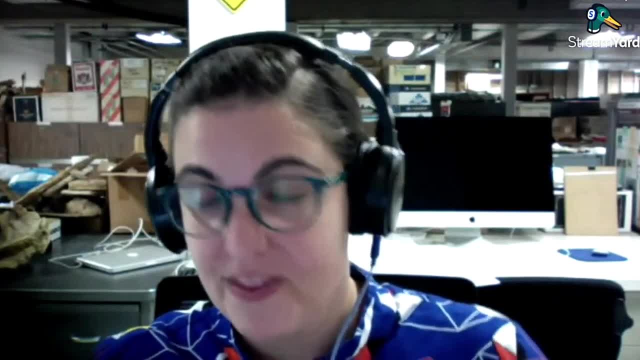 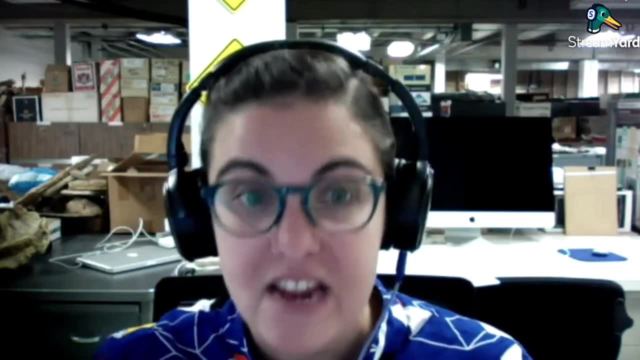 they can actually help us in a variety of ways. so at a minimum, they could tell us how long these species have been around, right? so if you have a spruce tree, an individual spruce tree, this 19th-century spruce tree is a spruce tree and it's a spruce tree and it's a. thousand years old. okay, cool, we know that at a minimum this species has been around for 9,000 years. same with with the Aspen clone Pando. that's 14,000 years old again. that's telling us. okay, at least 14,000 years old, like that is. 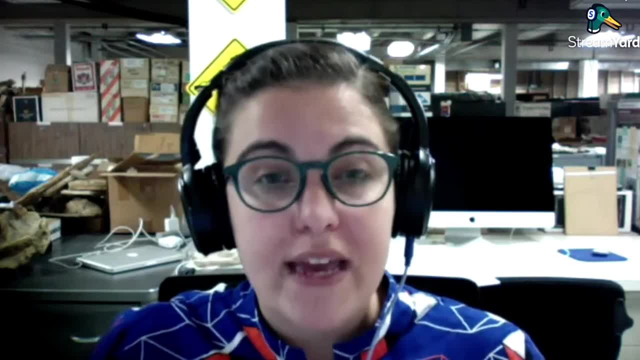 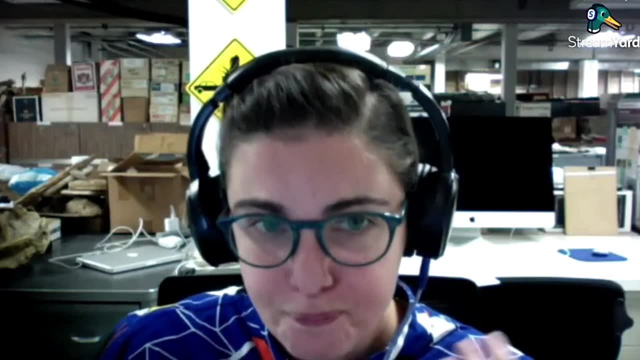 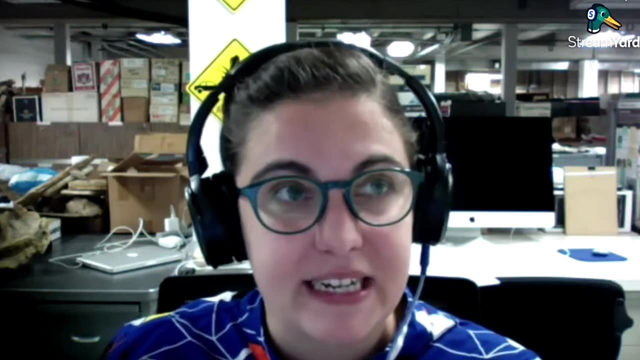 the age of this species. so we can use that as at a minimum to help us understand this. and then, in addition, it helps us kind of understand the different ways of living, because you have to be tough. the thing about plants is they don't move, they're stuck where they, wherever they were born, is where 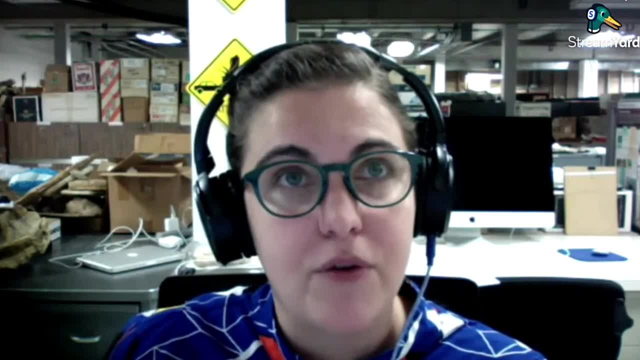 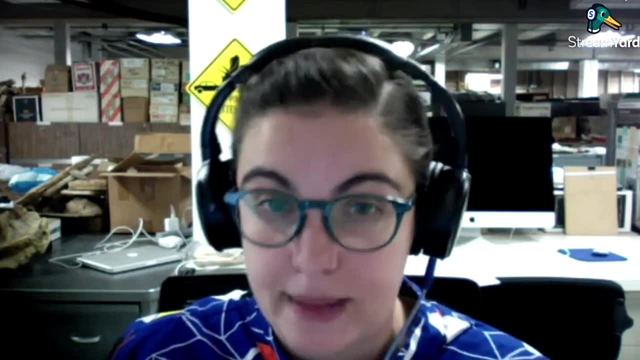 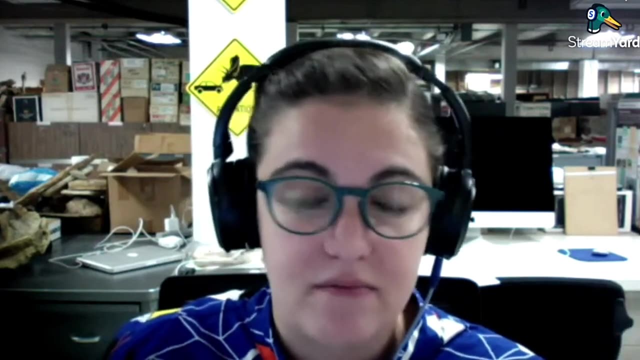 they spend their entire lives and so they can help you understand the environment and how that may or may not have changed, because the plant can't. if it gets too bad, the plant can't just get up and move um, so we can understand it from a from that standpoint as well. 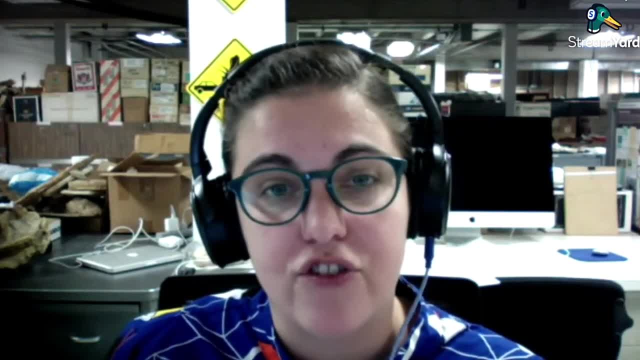 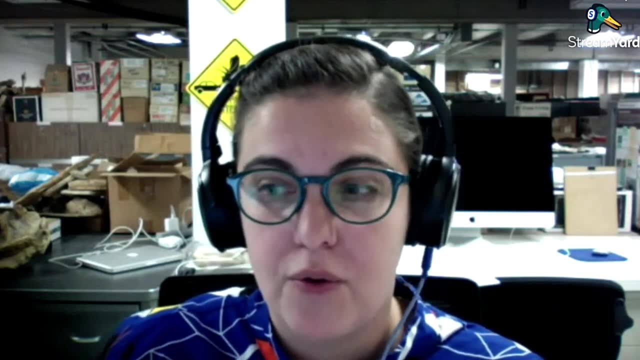 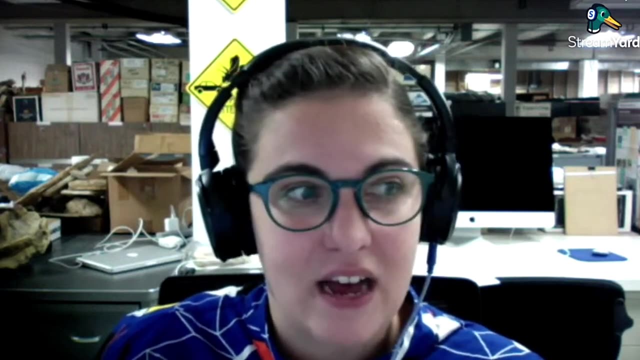 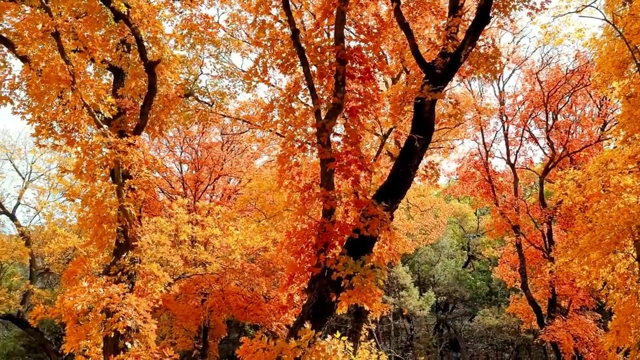 um, it can actually help us understand, like, how things have changed if you look at old individuals or relict individuals, so things that used to have a really widespread distribution but don't anymore, or you find species that are not where you would expect them. there is a canyon in Texas that has maple trees in. 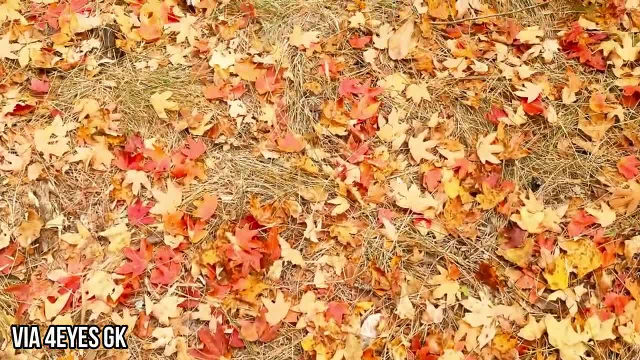 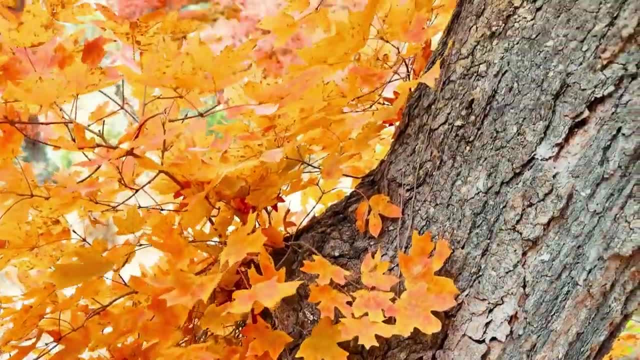 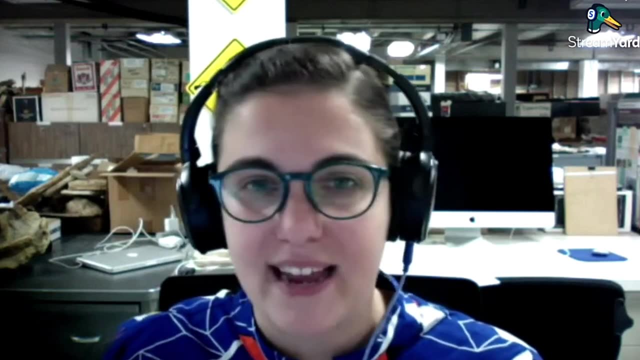 it. they're called the lost maples because during the last glacial maximum there were maples in Texas, because it was much cooler. but once the glaciers receded, these maples got stuck in a canyon and couldn't get out. so all of these things together can kind of give us a more complicated picture of how. 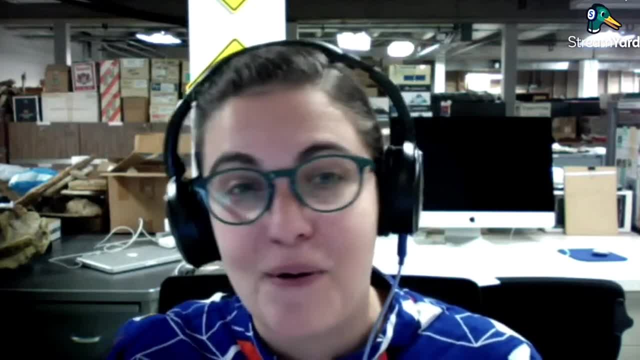 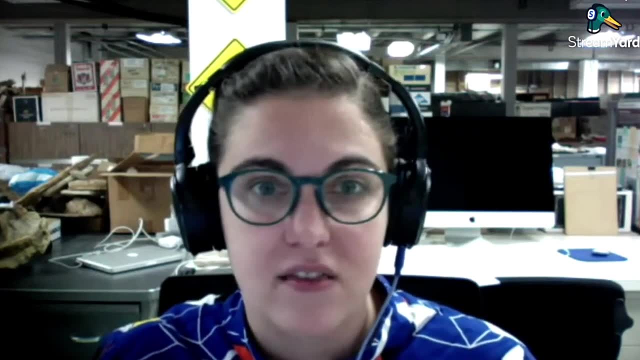 things are we can look at. we can also look at their DNA and see how it may be different from younger individuals of the same species. so we can get a sense for how. how are these, these species, changing genetically and how can we look at how that's changed in the past and how it's changed in the future and how it's? 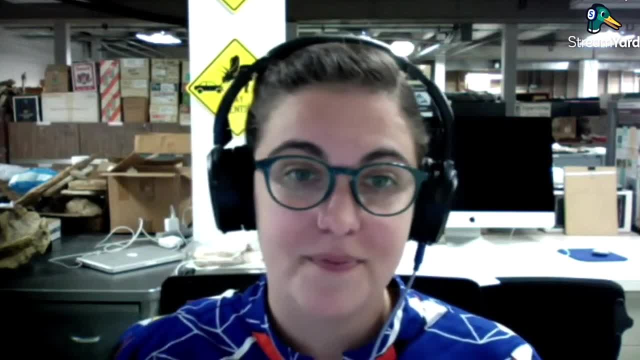 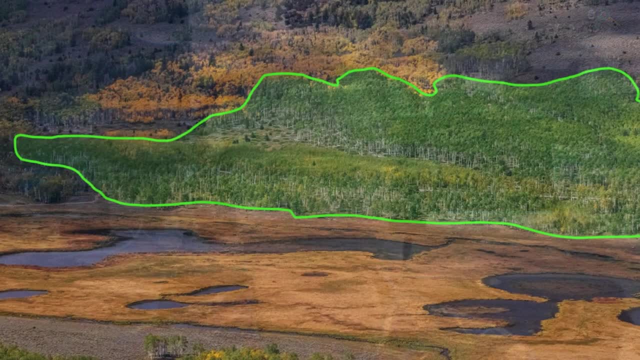 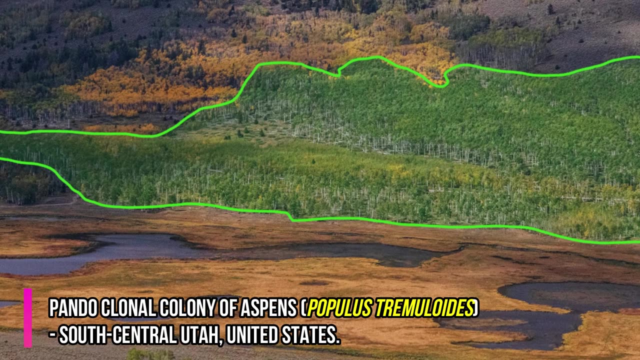 changed in the past and how that may continue to change in the future. so, getting back to the, this idea of a clonal colony, I mean, does it, is it that the plants just clones itself over and over again and appears to be so many thousands of years old? so the way that it works is that plants are not. how is 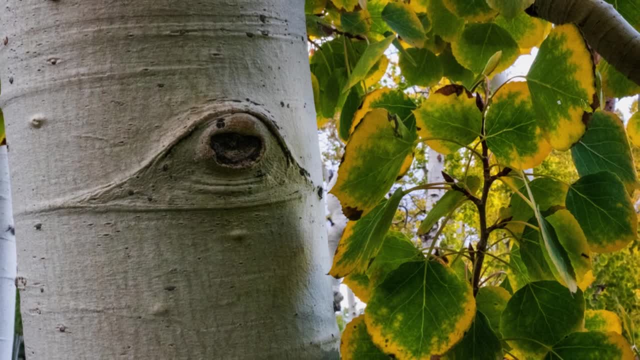 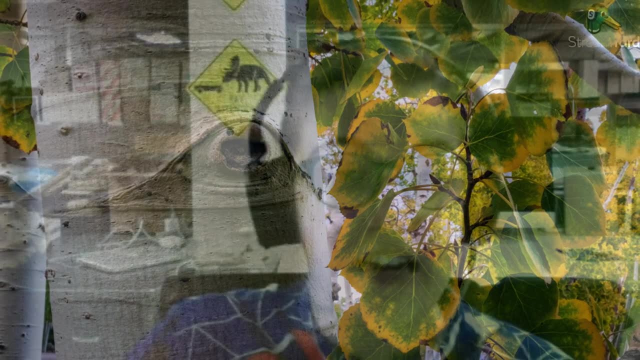 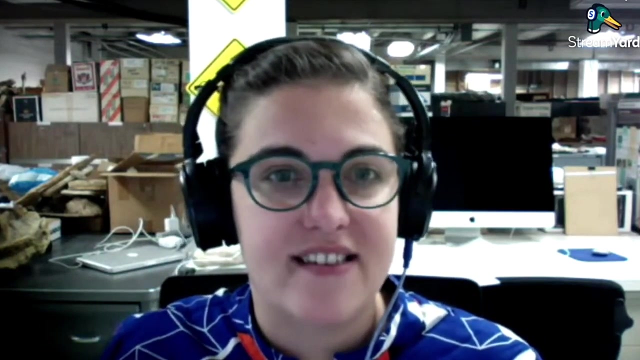 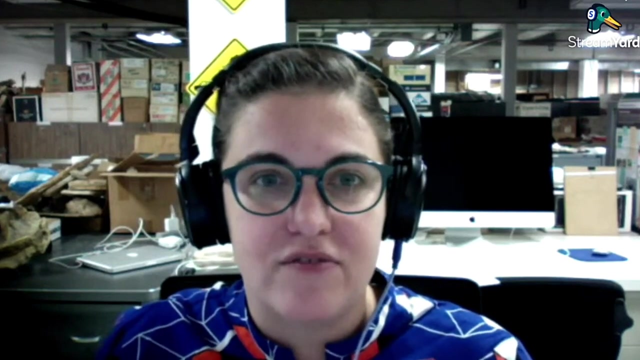 this described to me. plants are not obligate sexual reproducers. plants can just reproduce asexually. they can just vegetate ively, sprout off a clone of themselves. so these are basically just a way to think about. it is just that the, the tree, is basically just adding little bits of 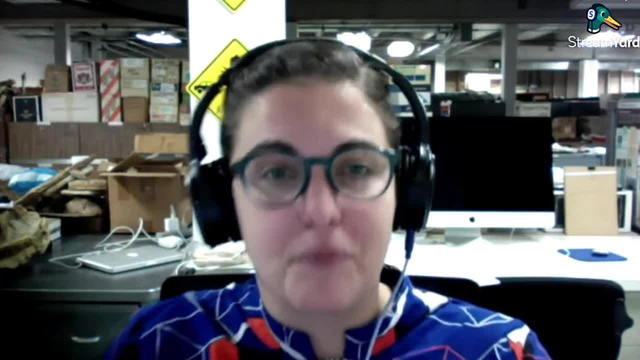 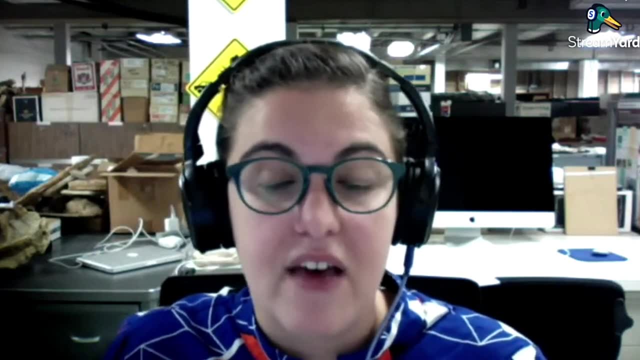 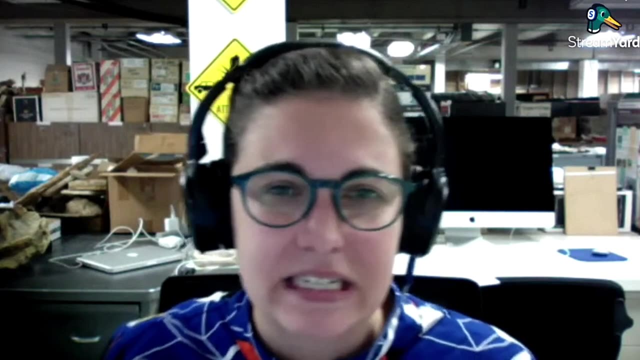 itself. so you could, if you dug back or, you know, explored back, you could probably figure out, like, what the original tree was. but they're all copies of themselves and so, and that's something that plants could do really easily, particularly plants that live in a little less enjoyable, I guess, environments, so like 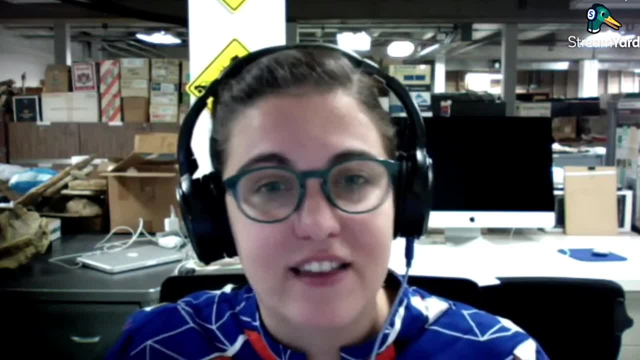 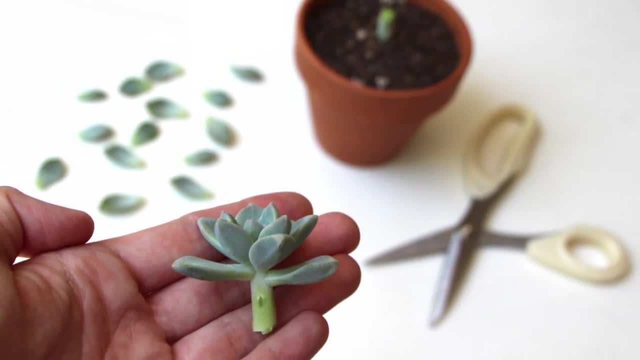 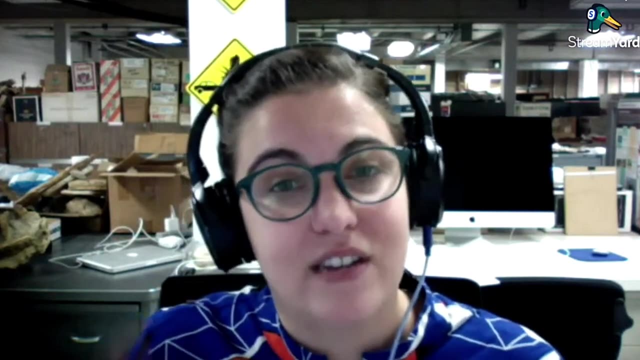 cacti, you know your. that's why like succulents. that's why you can give cuttings of succulents to people and they can grow them. that is vegetative cloning. that is the plant cloning itself and making copies of itself, because it there aren't others, there's its species around in order to pollinate and make. 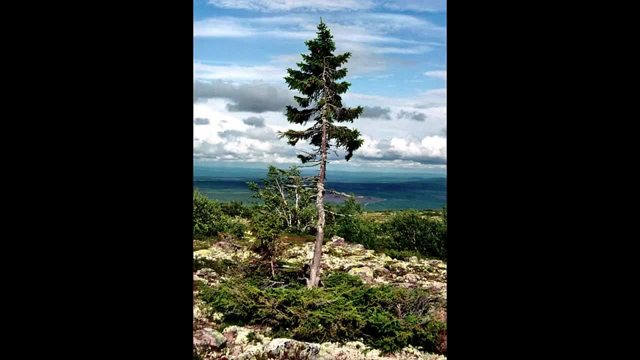 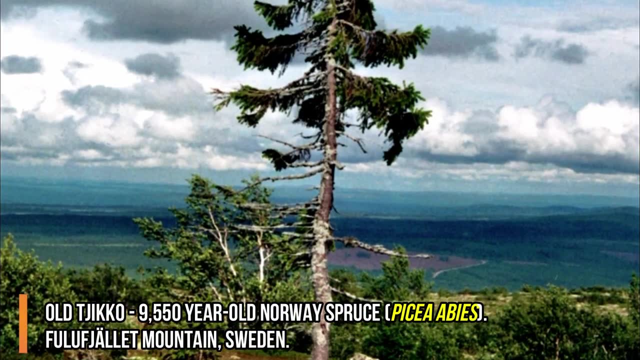 seeds and reproduce that way. The tree in Sweden, El Chico, is that basically one clone of itself, as it were, as opposed to the Pando colony, which is lots of ones which appear to be multiple. So some trees are just really old. 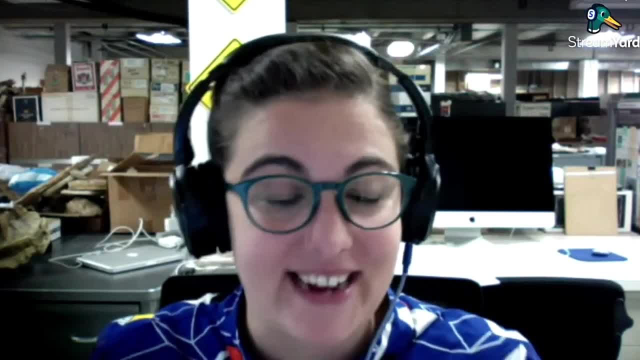 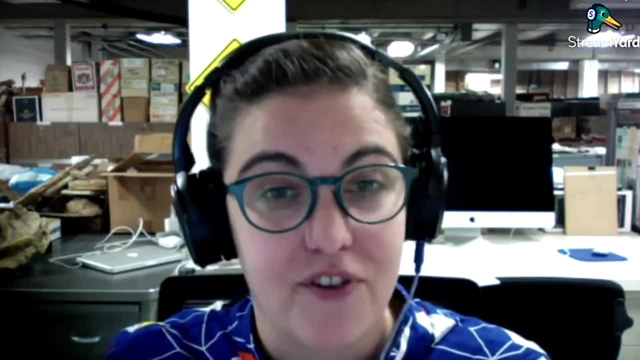 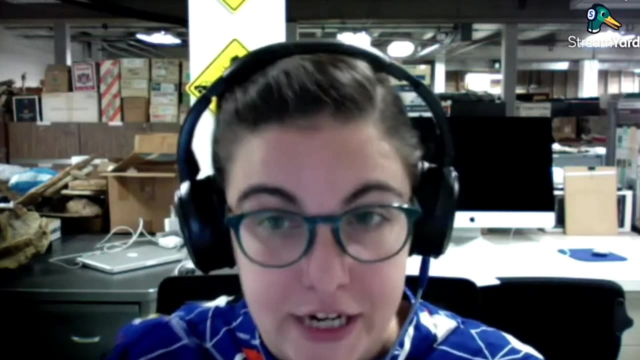 So the one in you know these are basically two trees that are coming at it from. they got old in two different ways. Either you can keep copying yourself so that if some of them, some parts, die, you know you still got more versus. there are some gymnosperms are particularly good at this. So think about, like the bristlecone pines in North America, This is a spruce in Sweden. Gymnosperms are much longer lived than angiosperms. They are a very like slow and steady wins the race. So they're not doing it the same way. 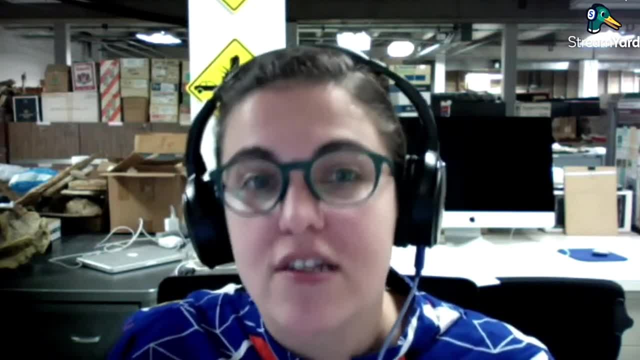 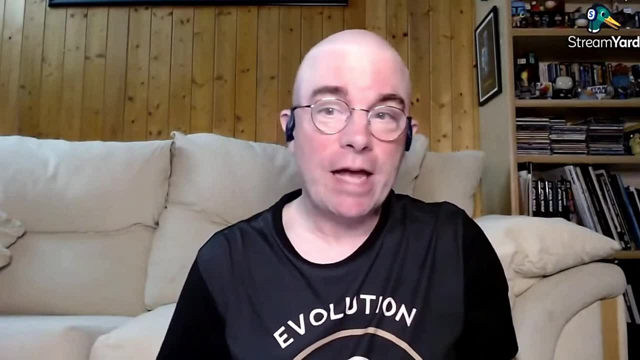 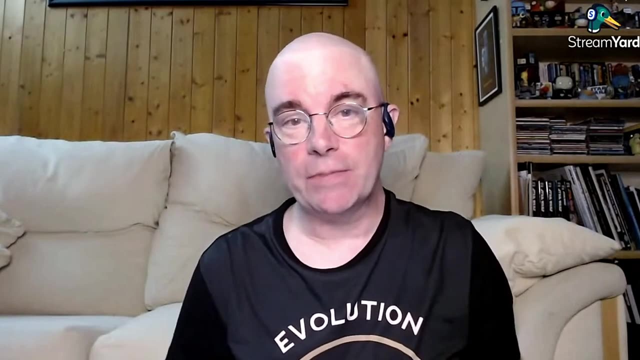 They got old two different ways. The one in Sweden is just a tough old tree. Well, I've interviewed quite a few evolutionary biologists on my channel and more than a few have referenced phytoliths as an excellent way of determining the age of a fossil specimen. 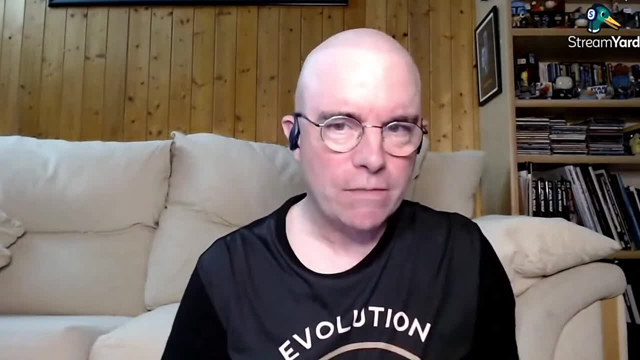 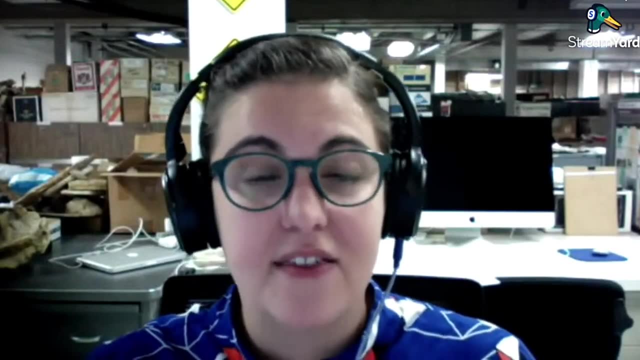 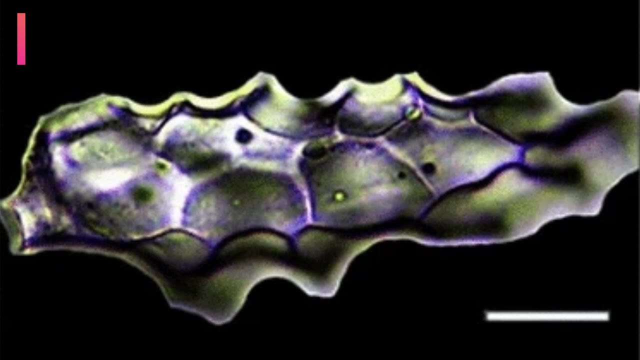 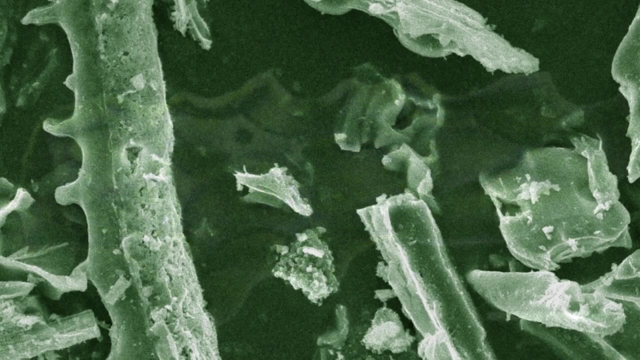 So can you describe for our audience exactly what phytoliths are and why they're so useful? So phytoliths the name. literally It means plant rocks, So they are bits of silica that are embedded in plants. So grasses in particular are famous for their phytoliths. 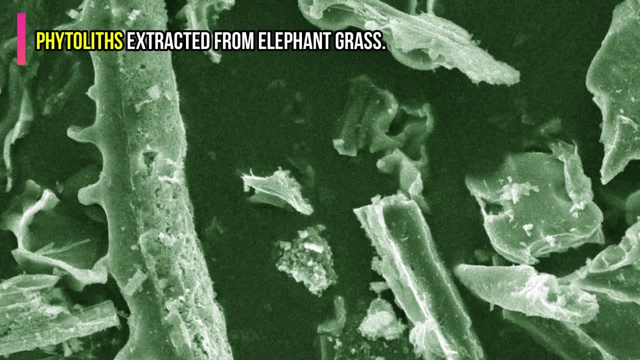 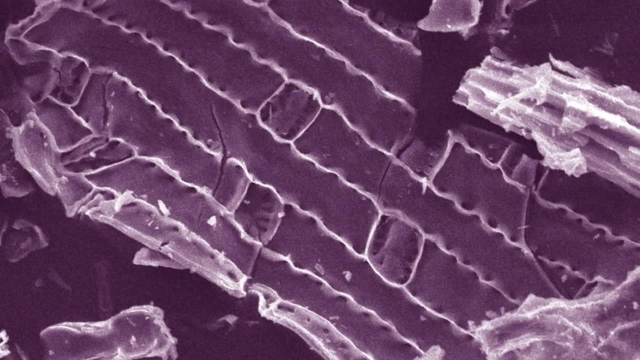 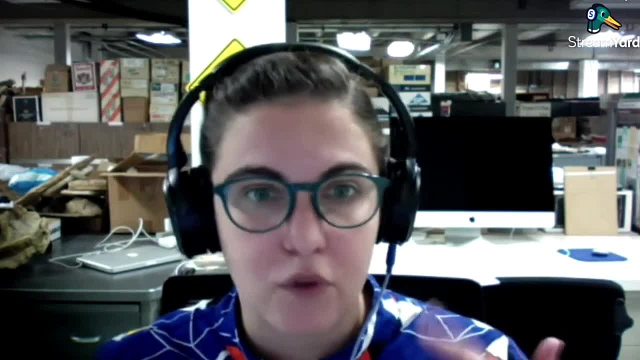 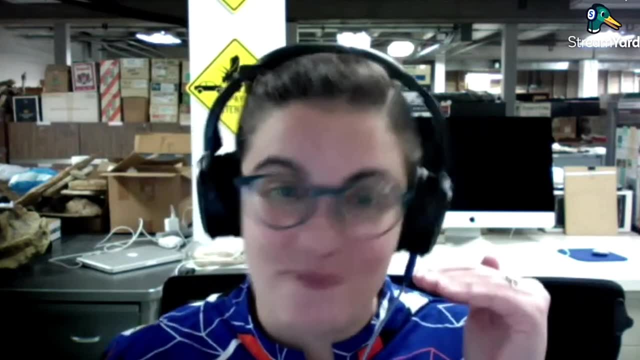 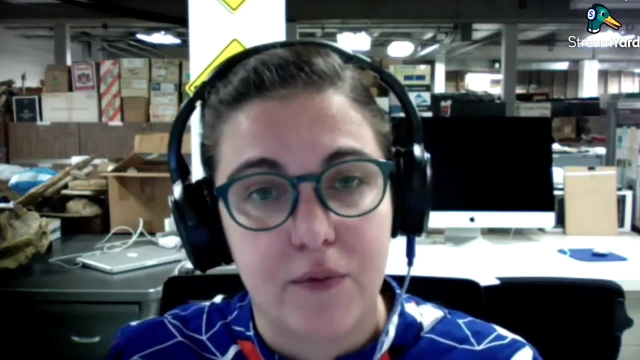 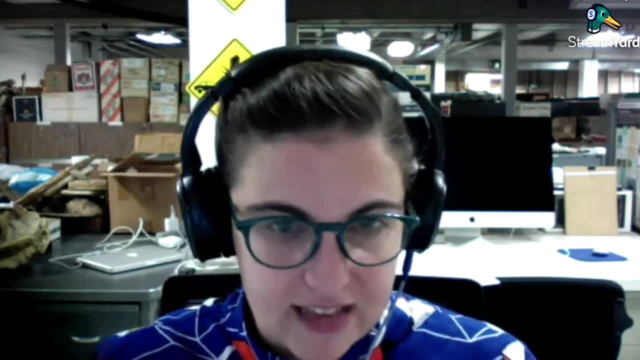 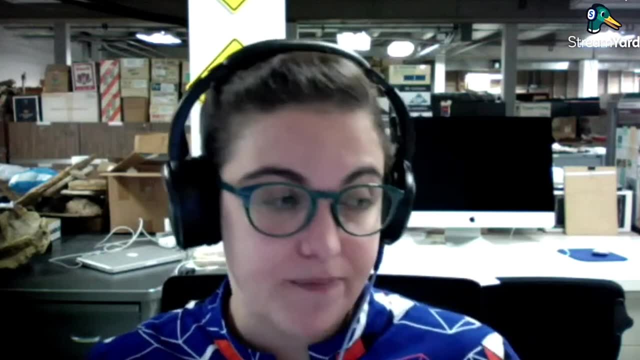 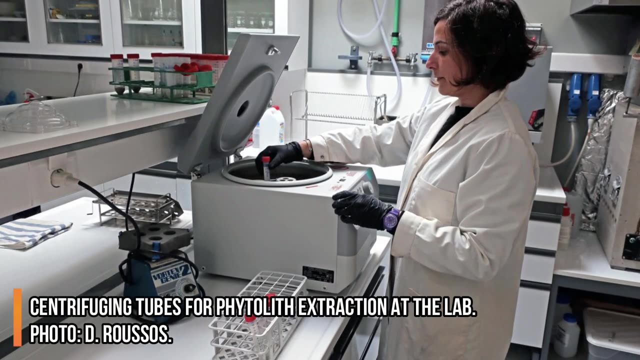 But it's actually much more useful because you can have phytoliths in a variety of different plants. They can help you actually Figure out what plant you have, even if you only have It's literally silica, It's sand. It's virtually indestructible. 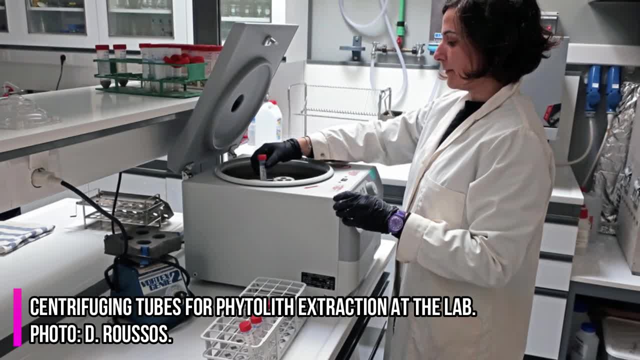 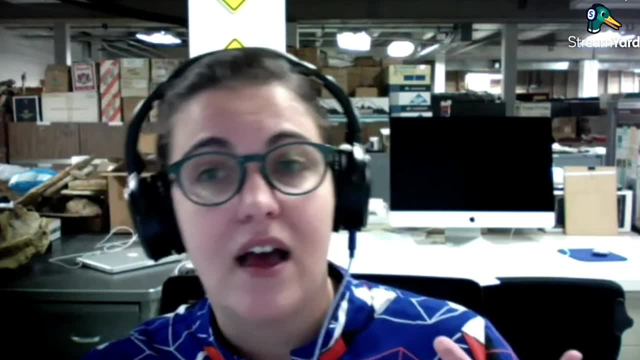 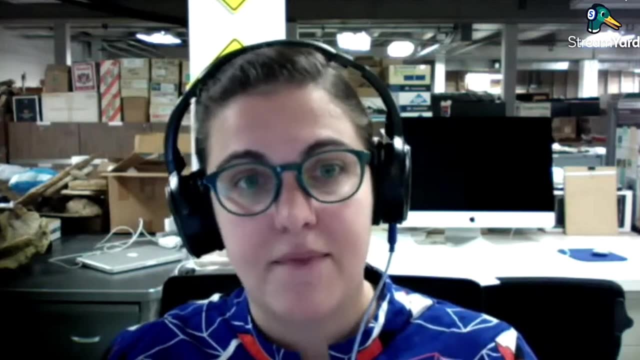 So you can use the shape of phytoliths to estimate what type of plant it is. You can sometimes use it to estimate canopy cover, The shape of these cells that these phytoliths are. they're part of a plant. The shape of them can sometimes tell you the amount of light. 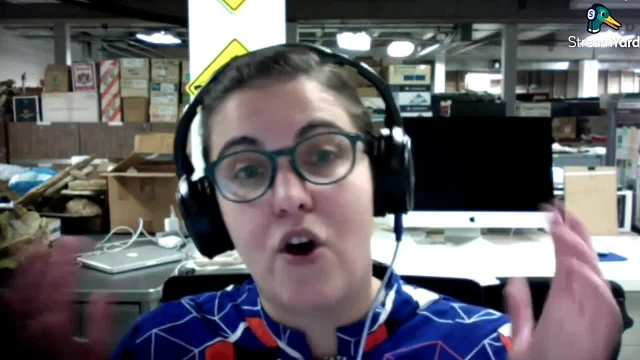 That the leaf got, so you can get a sense. if you have a very open canopy, so there's not a lot above your head, or if you have a closed canopy, there's a lot of stuff going on around above your head. 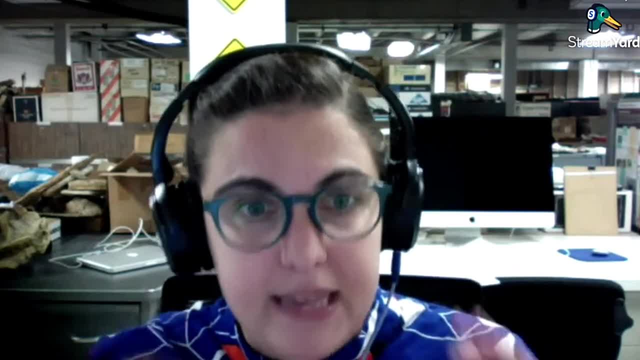 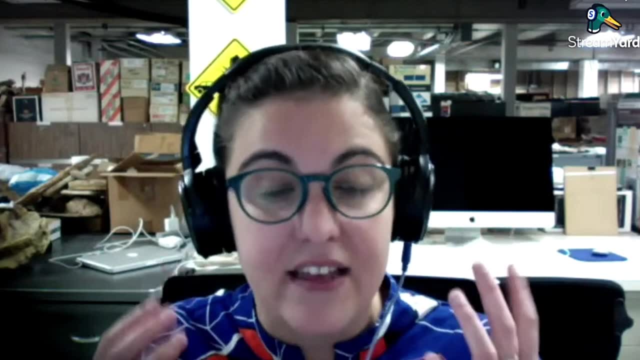 Pollen and phytoliths are basically indestructible. So phytoliths, like I said, they're silica, they're sand, Like it is one of the strongest materials. If you have ever taken a course in geology, you know that. 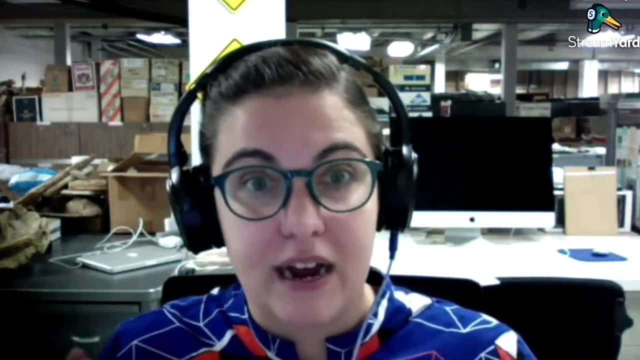 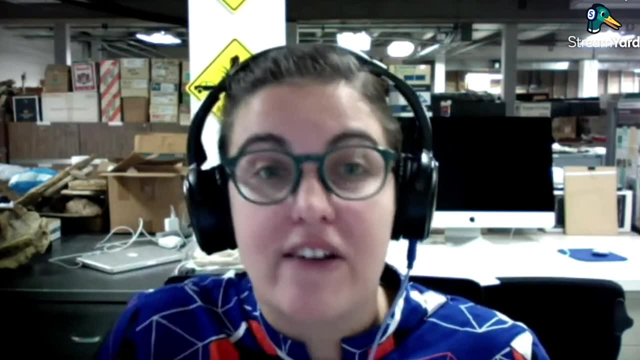 As Rocks break down and weather through time, Quartz, Silica, It's one of the last things to break down, That is, it's very, very tough. So that is why, like silica, these phytoliths are everywhere. 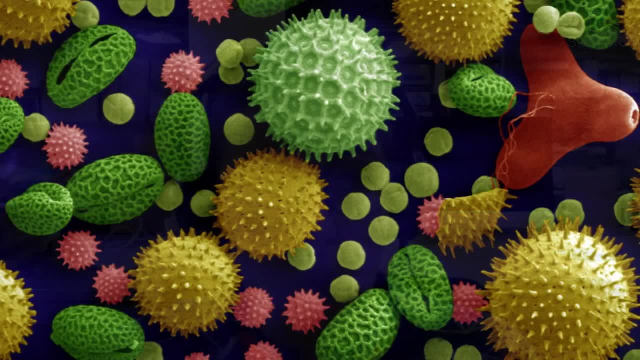 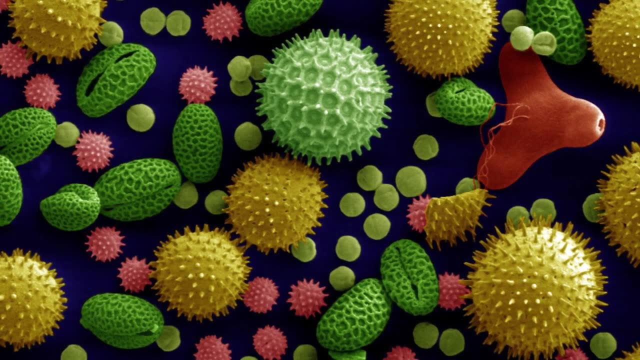 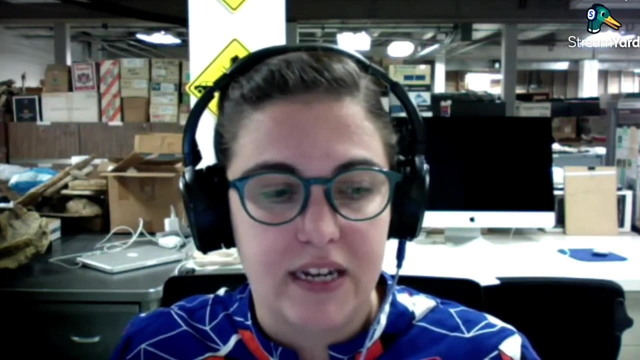 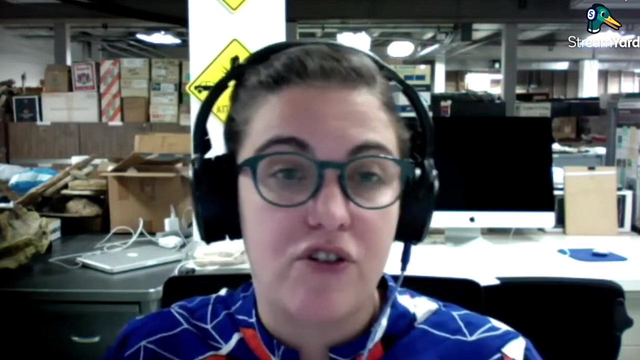 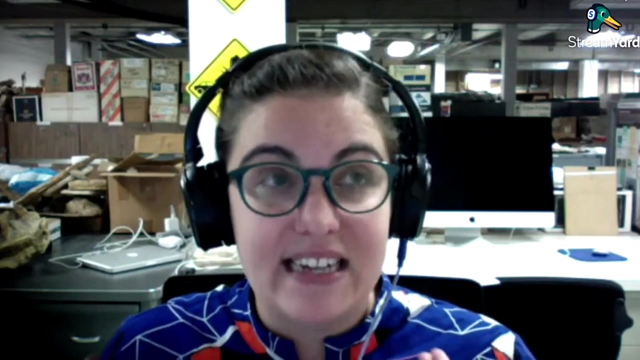 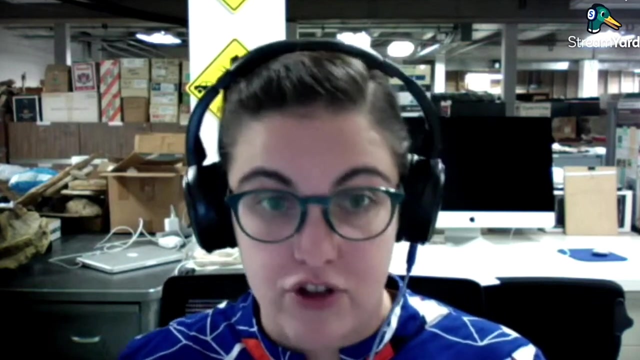 In pollen. pollen is made of polysporin. It is one of the strongest substances that we know of on earth. So even if you don't have, say, a leaf impression- Um, Because that is going to be much more, maybe ephemeral, it's the kind of thing- you need a special environment, you need a special, special situation in order to get that preserved and that is easily destroyed. if the rock that had a leaf impression on it is destroyed, like sorry, your leaf impression is gone, but you can get. 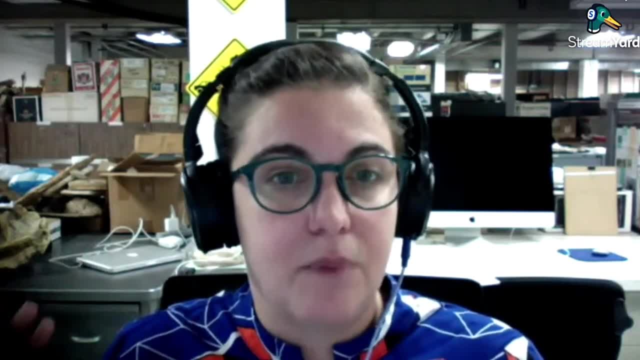 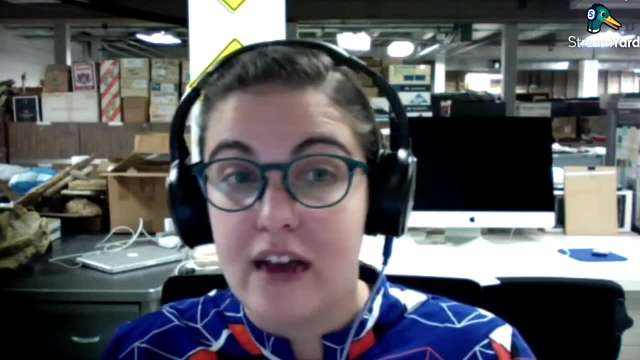 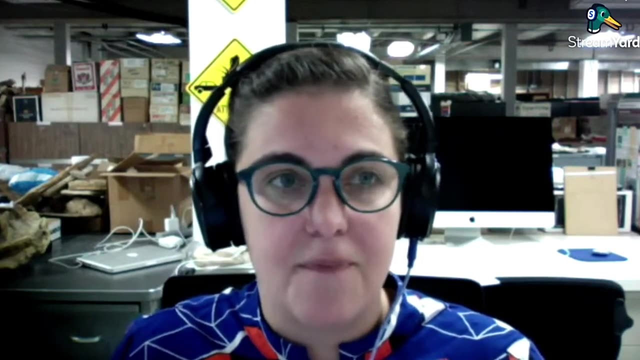 Um, Um, Uh, phytoliths and pollen in a lot of different contexts. It's really interesting because, like I know people who study vertebrate paleontology and you often do not find fossil leaves um preserved with fossil vertebrates, but you often find um phytoliths and pollen. 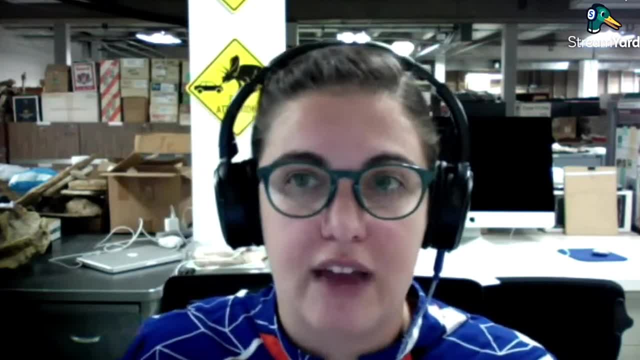 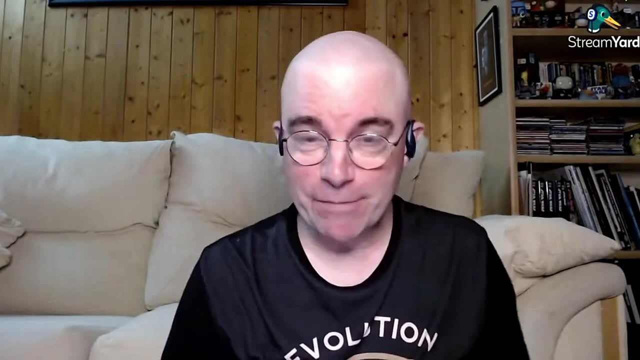 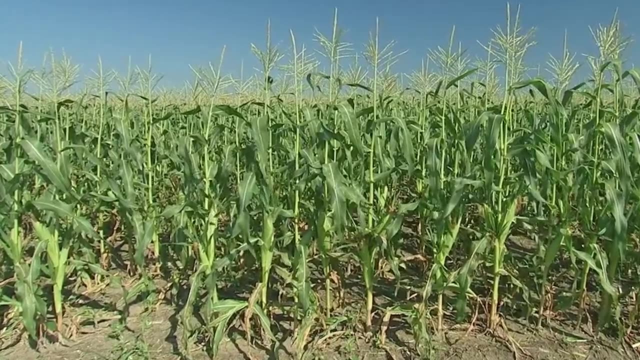 So that's another way to get at that plant picture when you don't have, say, petrified wood or leaves preserved. Well, we humans love to breed and manipulate plants. Yeah, We have in our homes or in our gardens. we've domesticated cereal grains such as corn. but no matter how much we try to change things, it seems that nature has already got the jump on us. 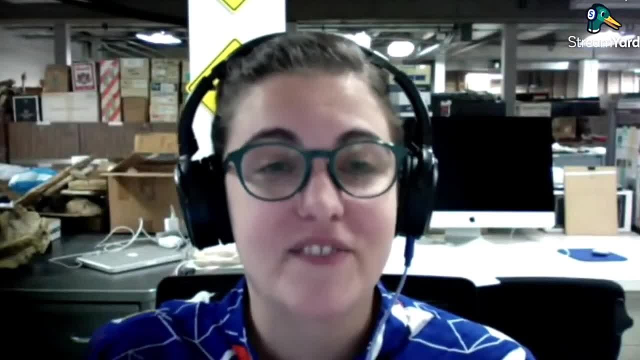 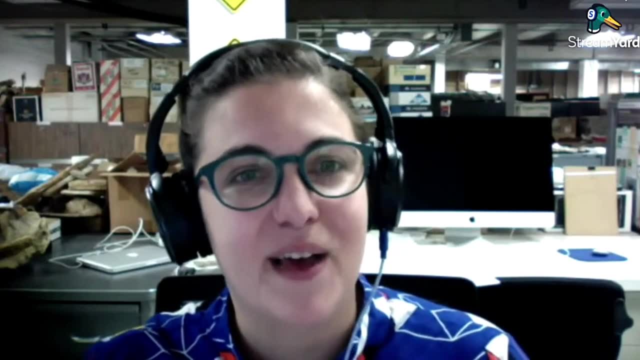 Isn't that right? Oh yes, You humans have loved plants as long as we've been humans. Um, and it's really fascinating to see that kind of play out, um, both archeologically but also genetically. Uh, and it's fascinating because humans love orchids. 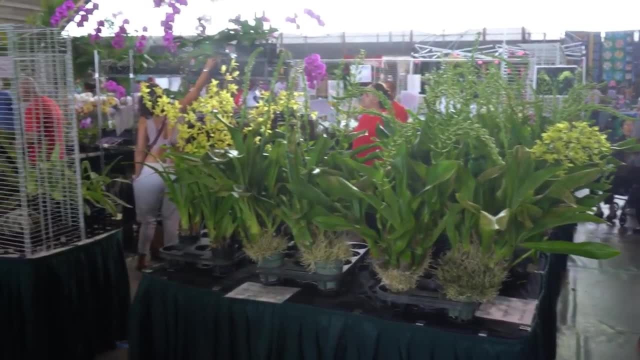 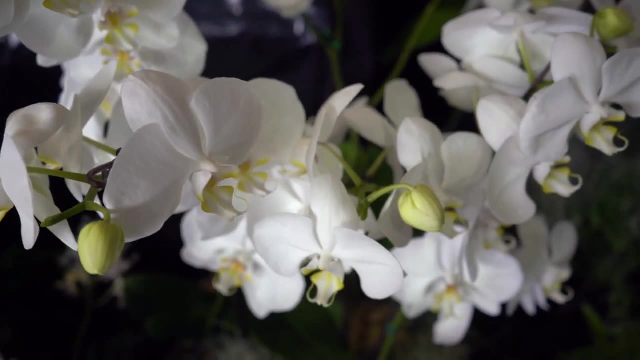 Humans have loved orchids, basically as long as we've lived places with orchids Um like. we see this, this um relationship between humans and orchids in the archeological record in like Greece and Rome, but also China. 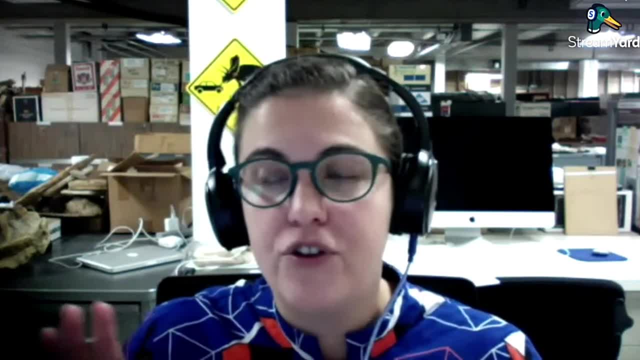 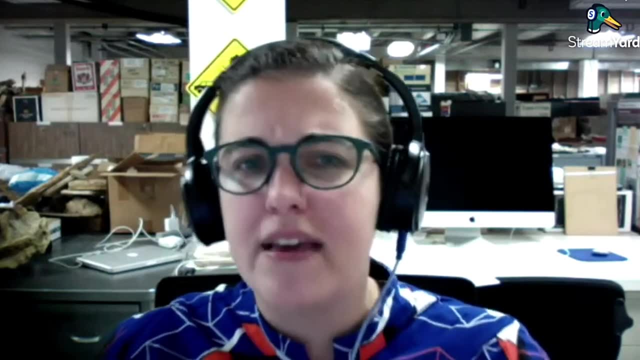 We love orchids, Uh, and so we a lot of people think, and if you do kind of like preliminary research of orchid varieties online, it may seem like: oh yes, humans, We have uh selected all of these varieties and we have, you know, crossbred things. and that's true, we've done. that, but orchids have it like taken care of. there are almost 30,000 species of orchids on the planet and for perspective, that is roughly the same number of species as bony fish. it is roughly twice the number of species as birds and about four times the number of species as mammals. so that's crazy. there's so many orchids right, so like we have hardly made a dent in the number of orchids just by. you know crossbreeding ones that we think are pretty, and part of the reason that orchids are so speciose is just because they are such specialists, so orchids tend to very small. ranges. they are not generalists. you can find them everywhere, but the species will have, uh, very small ranges. but yeah, like humans, humans love orchids, like vanilla, and you know, not just looking at them, but like we think they taste great too. um, and this is something that humans do, we find plants, we like them and we. 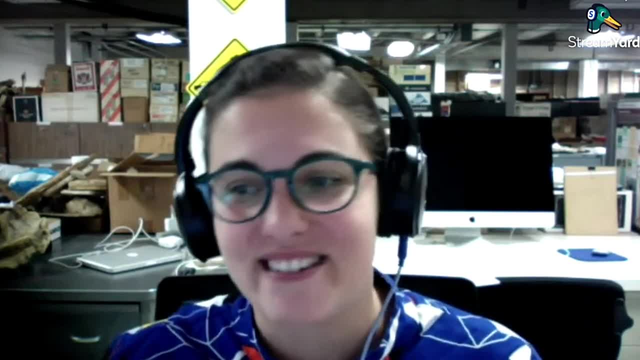 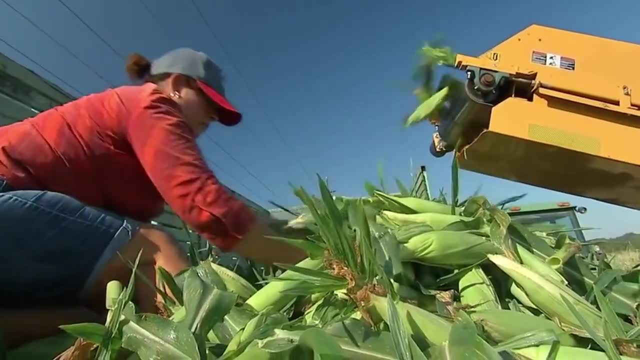 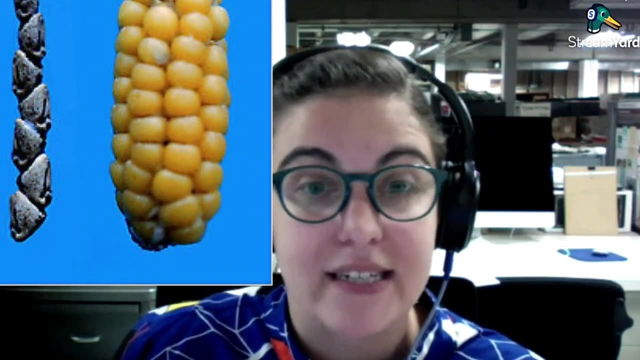 manipulate them? uh, we bring them with us all around the world. um, it's fascinating. you mentioned corn in the beginning. the wild type of a lot of plants is often indistinguishable from the thing that we eat. um, so teosinte, which is the wild type of corn, hardly has any kernels. it doesn't, and it doesn't really. 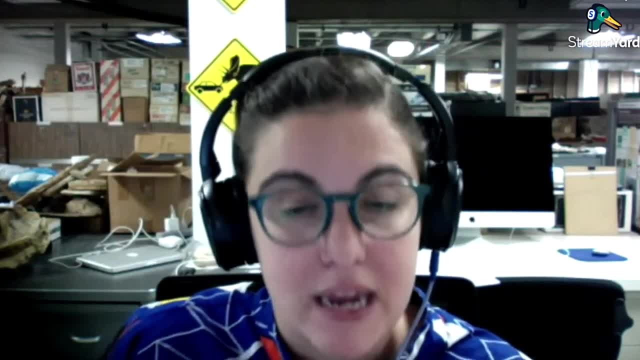 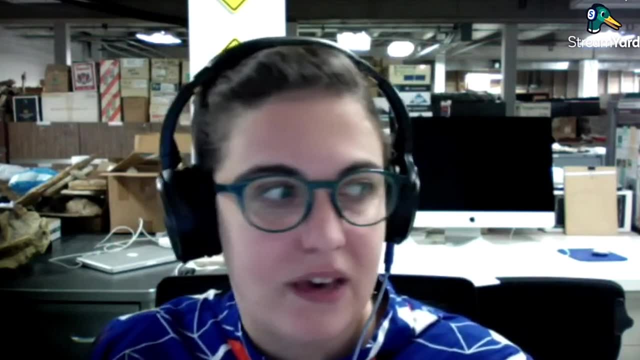 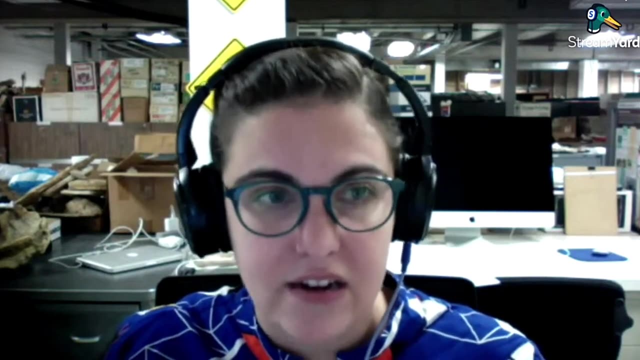 look like corn we have. you know, humans have been manipulating corn for thousands of years to make it the easily- um, the easily edible thing that it is today. you know, if you look at wild types of a lot of cereal grains, they are not nearly as um, easily grown as the things that we eat today. so 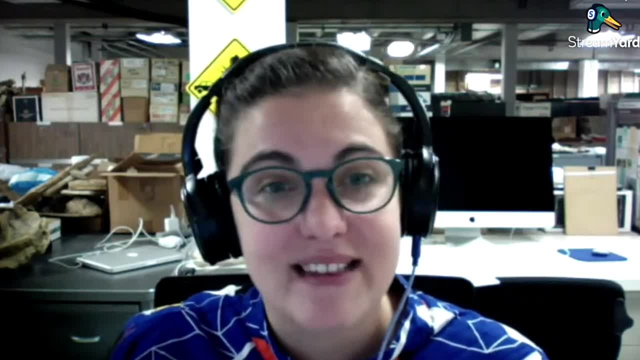 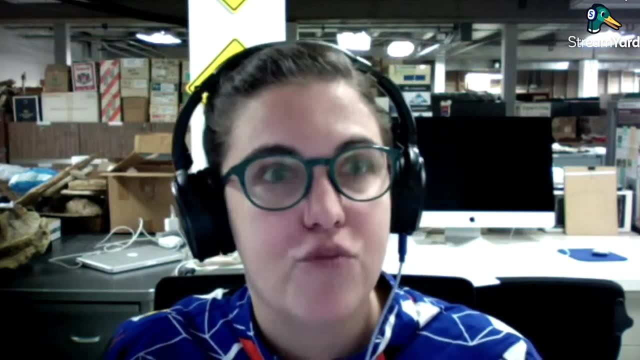 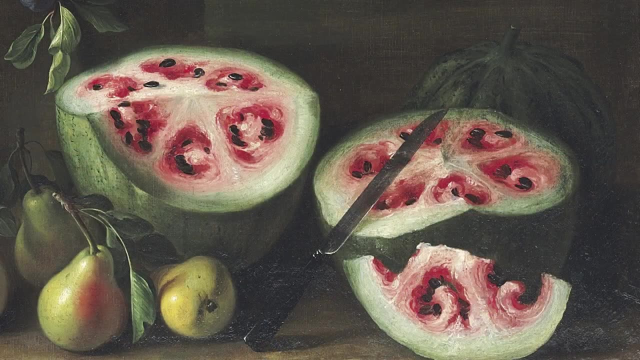 we have domesticated and changed through time. we have domesticated so many plants that people haven't really thought of like watermelons. they used to have um, much more right than than the actual, uh, like edible flesh that you think of if you see a watermelon, if you look at like historical. 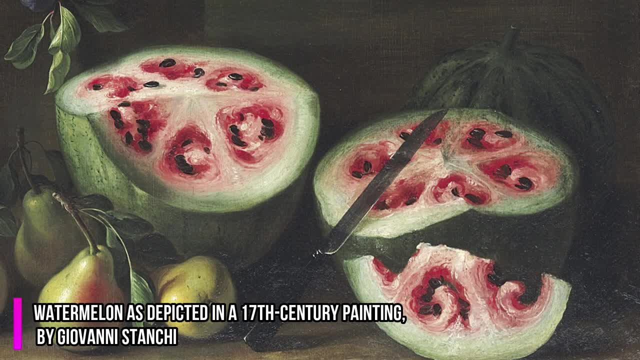 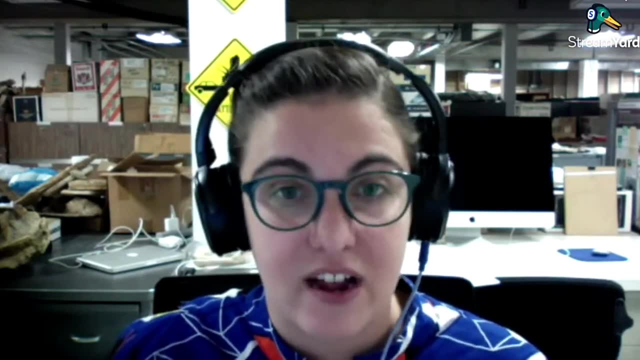 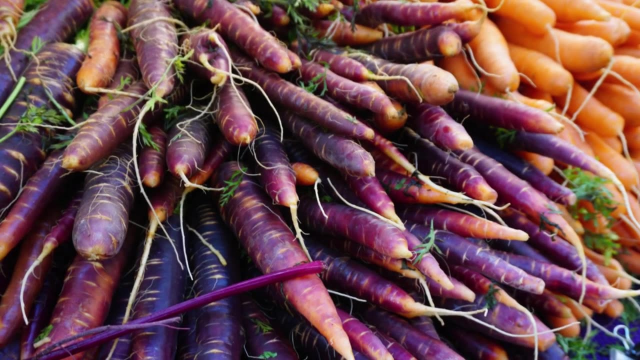 paintings of watermelons. they look nothing like what we're used to. but uh, carrots. carrots weren't orange until fairly recently. they used to be a whole variety of colors. we bred them to have more uh carotenoids in them, and so they're orange bananas. obviously they weren't. 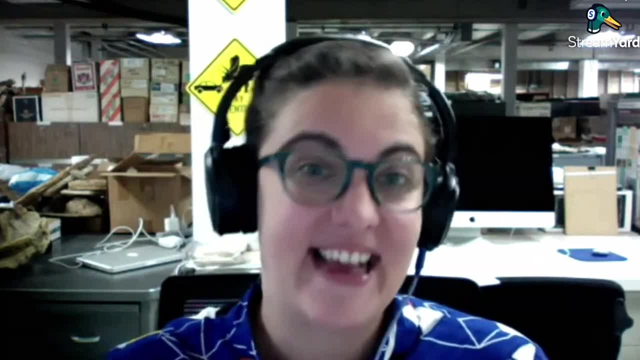 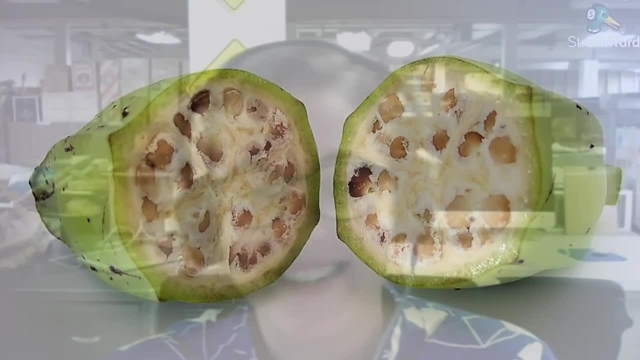 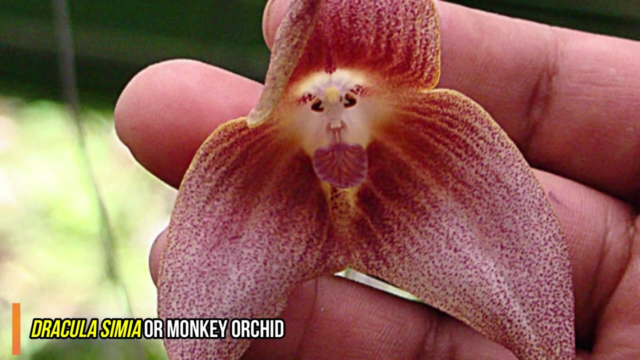 as beautiful, you know. so you see them now. yes, exactly, the bananas, um wild bananas, have huge seeds, oh my goodness. and getting back to orchids, i know i've seen one. i think they call it the monkey face orchid, because it does have a kind of a this, this look, this look of a monkey's face on it. now, surely, that's, uh, humans did that i? i doubt it. you know the the cool thing about orchids is that, um, like i mentioned, they have these really small species ranges. uh, they tend to you just don't have a lot of any particular species in general in the wild. um, you know, compared to how many species there are. 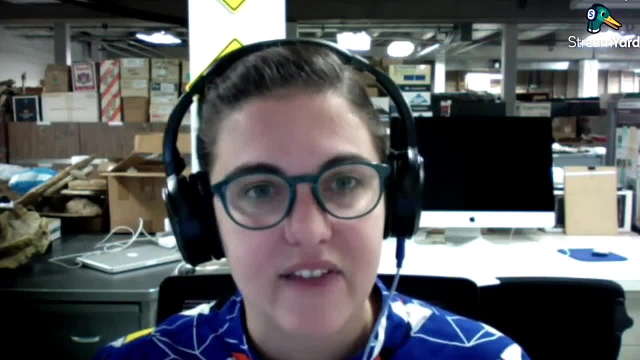 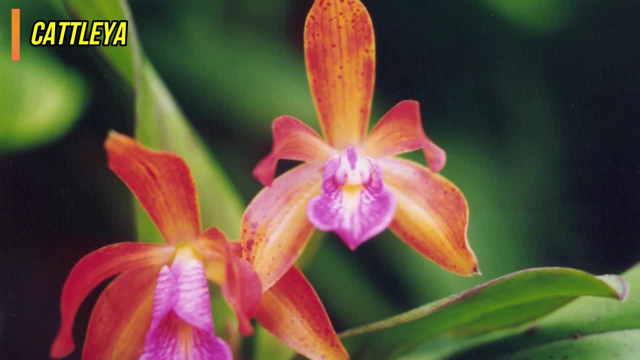 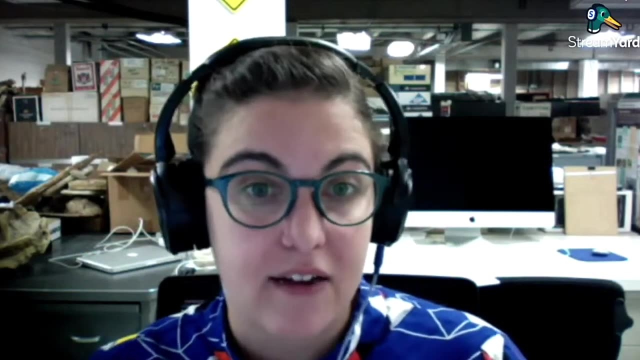 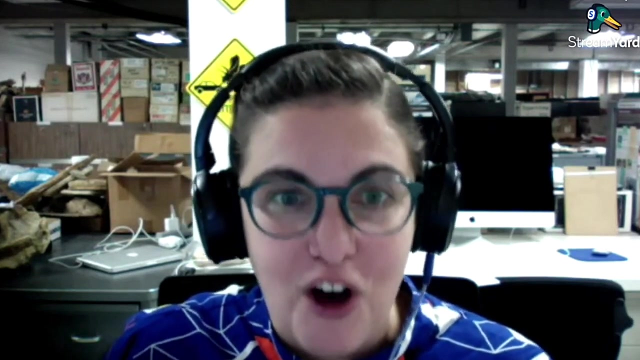 um, and so orchids have adapted in a couple different ways in order to maximize um their reproductive potential. so they tend to they actually flower for a lot longer than a lot of other flowering plants. um, because the longer that you have a flower, the longer you might be. 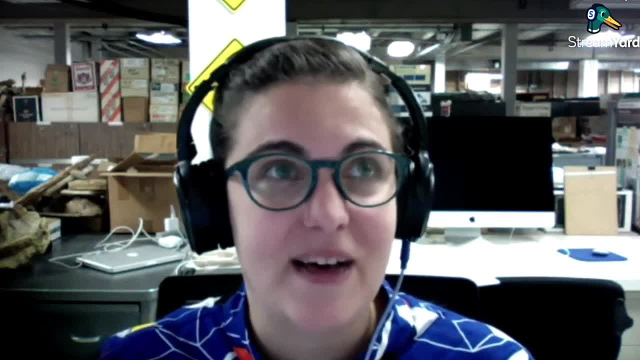 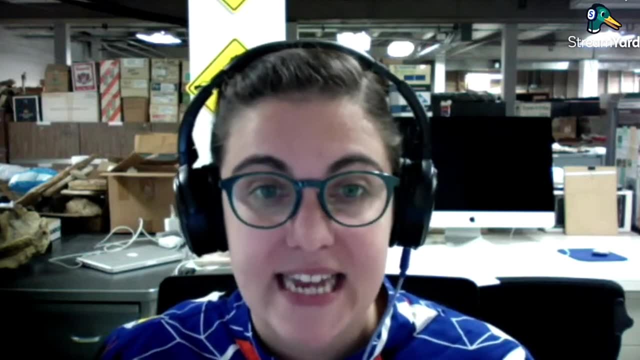 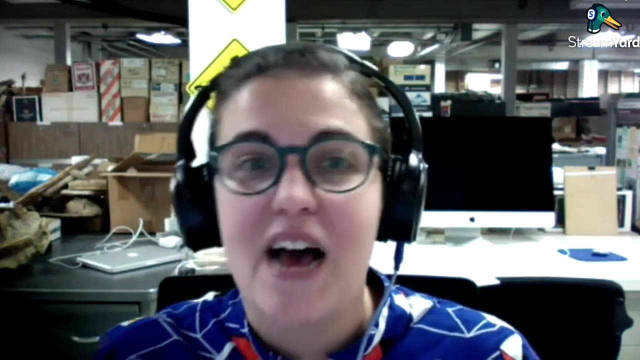 pollinated um. in addition, um, a lot of the reason we see a monkey face is because um orchids tend to have bilaterally symmetrical flowers and they tend to have a lot of different types of flowers, and that's part of the reason why you can see a face in it. um, they tend to have bilaterally. 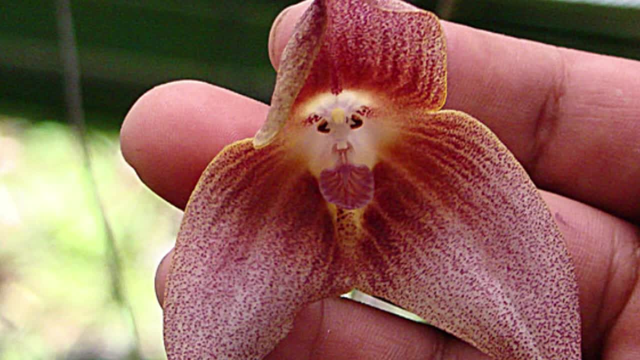 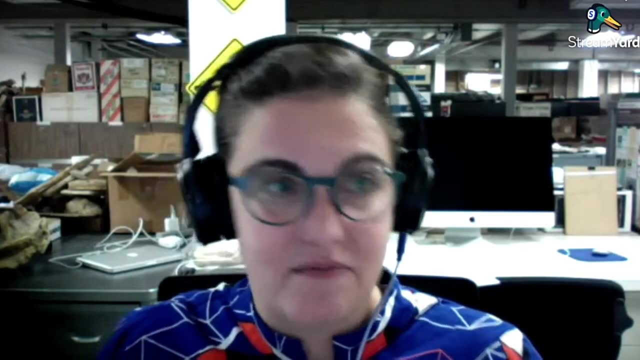 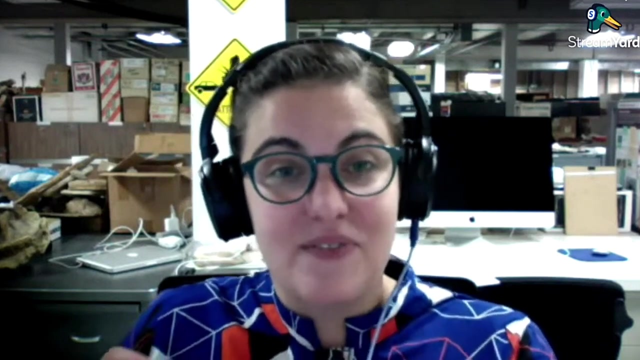 symmetrical flowers and they tend to have, um, a medial petal, so a large middle petal that's on the bottom, in the middle again. so like to kind of. that kind of gives us like a reminiscence of a monkey face. but the reason they're shaped like that is if there is a pollinator, the pollinator will sit on. 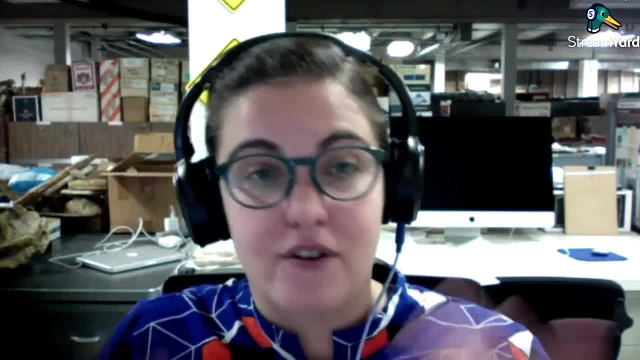 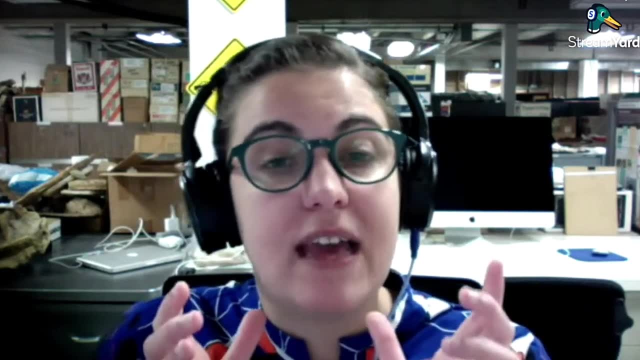 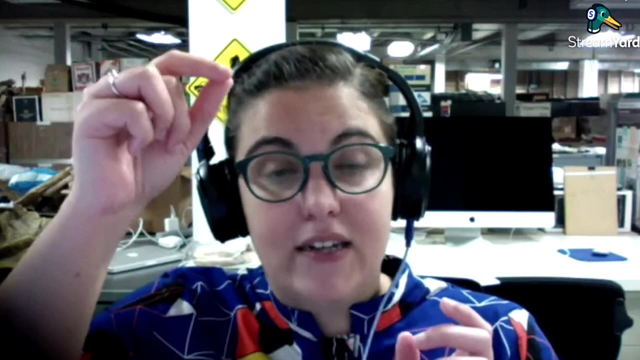 the um, the, the petal. it's like a platform, so it makes it easier than easier for them to collect pollen. but in addition to that, um, those, those weird shapes also mean that if the plant is not pollinated, it can self-pollinate, and if the pollen can fall down into the flower- and it can- it can. 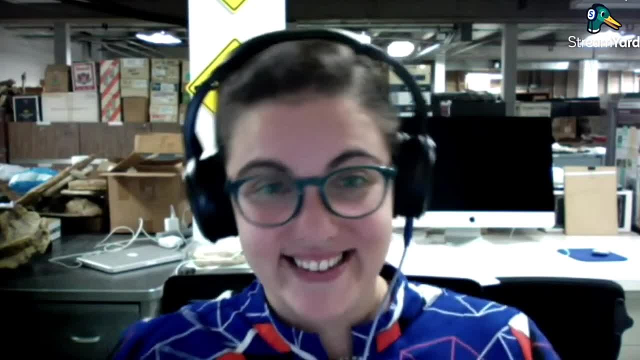 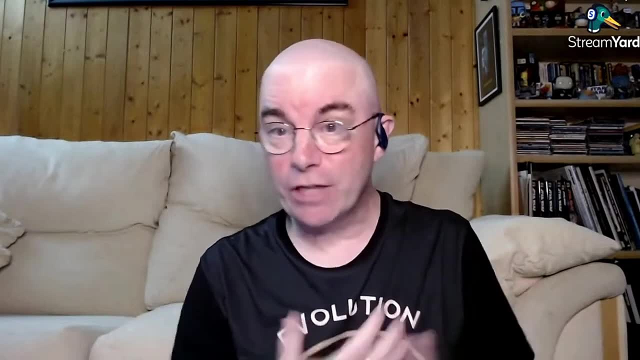 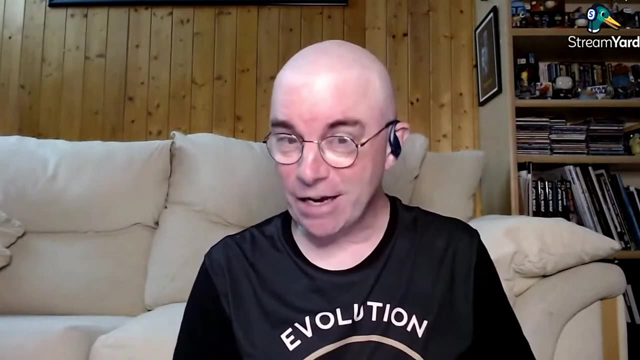 self-pollinate. but anyway, we humans, we see faces everywhere. so, yes, this is true, this is true. well, on this channel we cover human evolution quite a bit. it's certainly one of my favorite topics- sciences- but people may not know that you did your dissertation research in kenya, working with 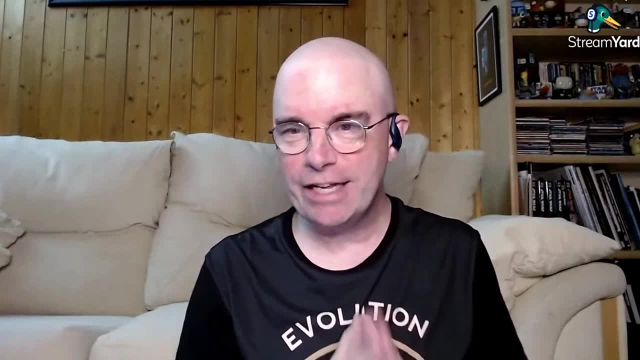 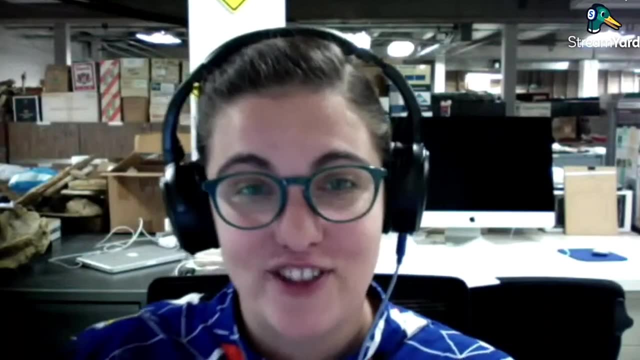 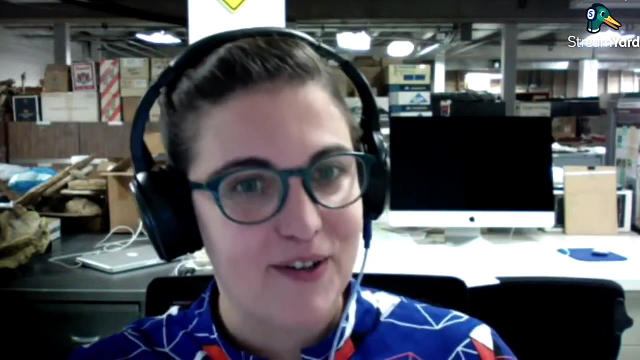 paleoanthropologists on myosin apes and human evolution. so how does paleobotany fit into all of this? so at the very beginning i mentioned that i got to paleobotany the long way and i actually left out a key detail that um. in undergrad i majored in environmental science. i studied 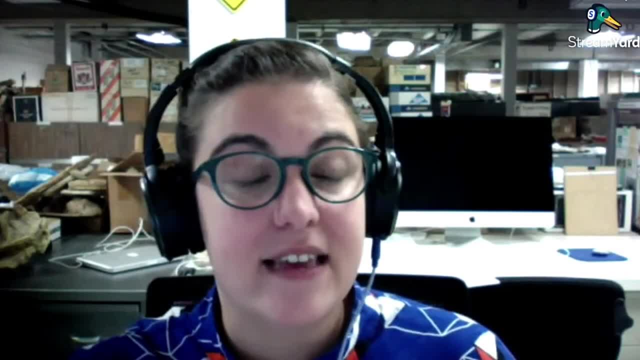 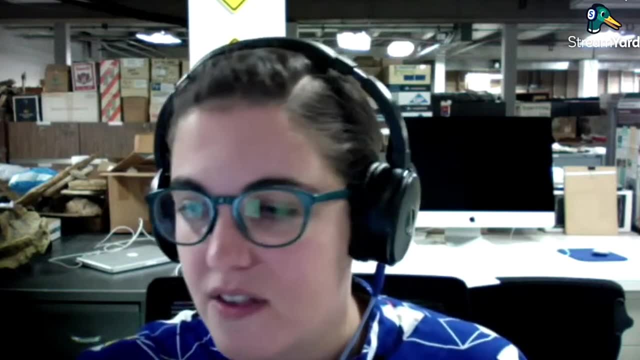 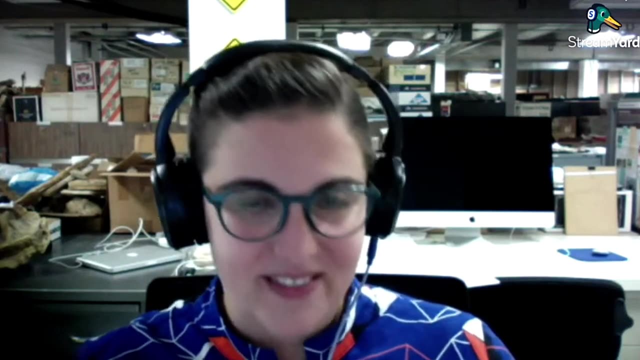 but i took nearly as many classes in biological anthropology. i have always found human evolution really interesting, so that was again one of my early loves. um. and so when i was looking into graduate programs i saw that um, the person who became my dissertation advisor he was looking at 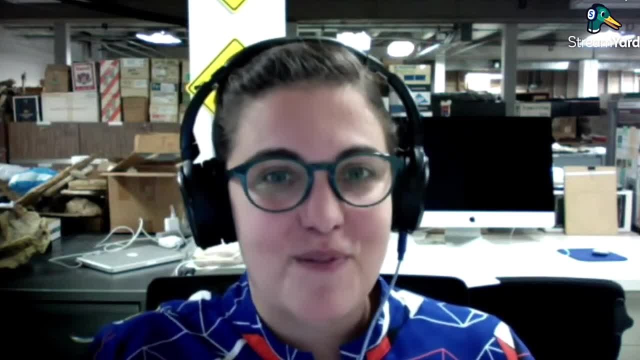 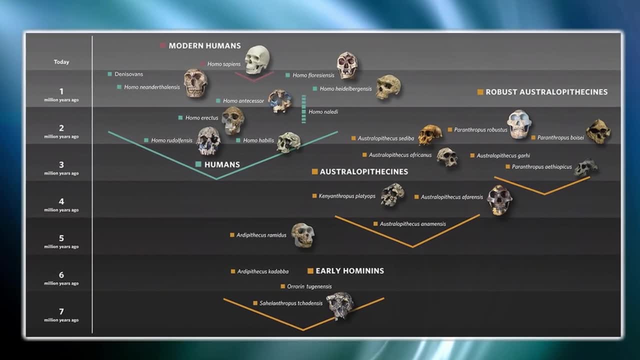 he had a project looking at the relationship between paleoenvironment and paleoclimate using plants and early evolution. so i was looking at the relationship between paleoenvironment and early human evolution and it's like those are my two favorite things, um. so i contacted him and 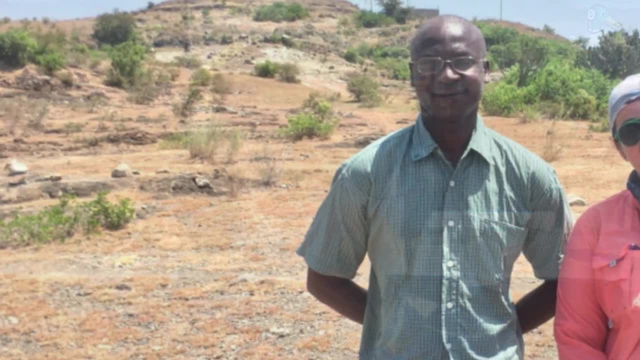 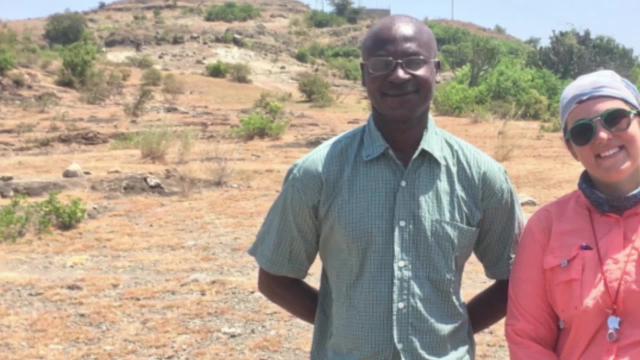 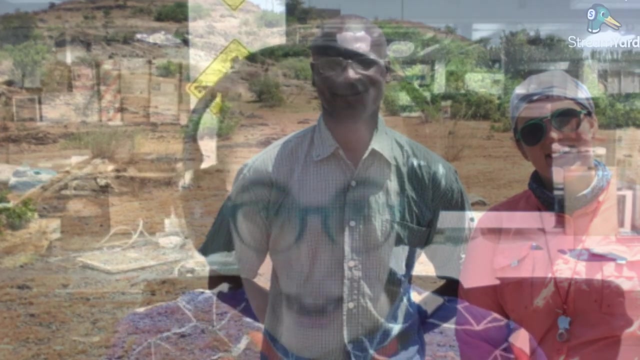 exactly. it was everything i wanted. so when i was in kenya, i would. i was often the only paleobotanist and i was often the only paleobotanist a lot of these anthropologists knew um, and so i would kind of joke that what i was doing, you know, i was the context, because what they were looking at were 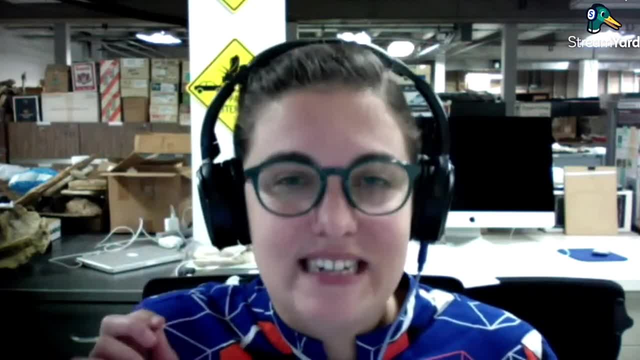 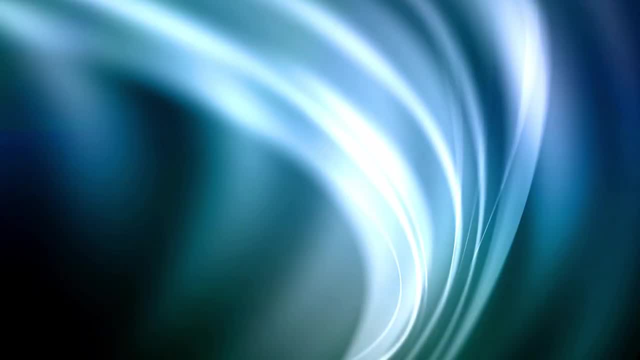 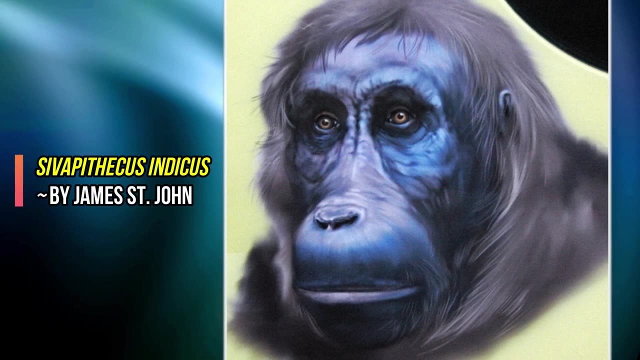 these just very minute details and look, counting the number of cusps on a tooth to see if this is the same species or maybe you know, is this variation and people were were wanted to make these connections about the evolution of these miocene apes, but you really can't understand what's going on. 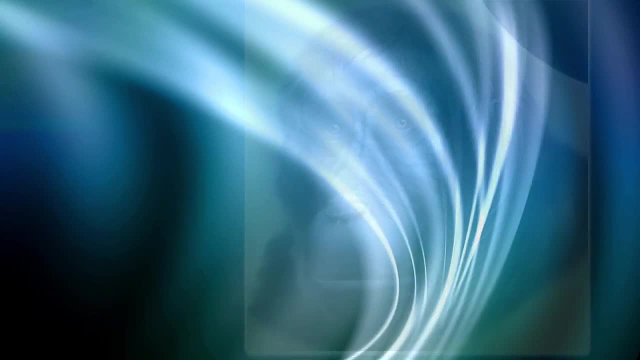 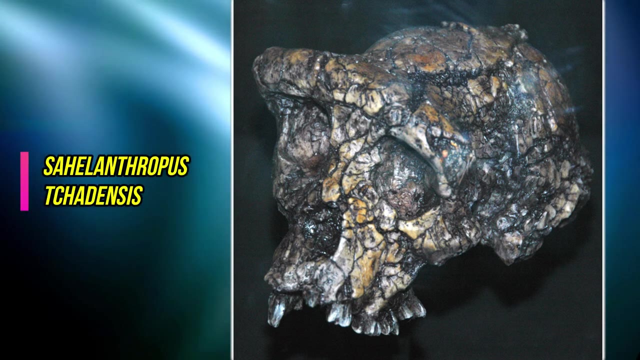 evolutionarily if you don't understand the context, if you don't understand the world that these animals were living in, if you don't understand the context of the world that these animals were living in, if you don't understand what the possible impacts on their lives were. so, in order to really 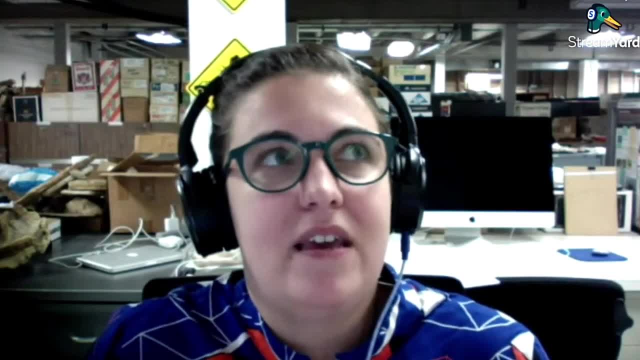 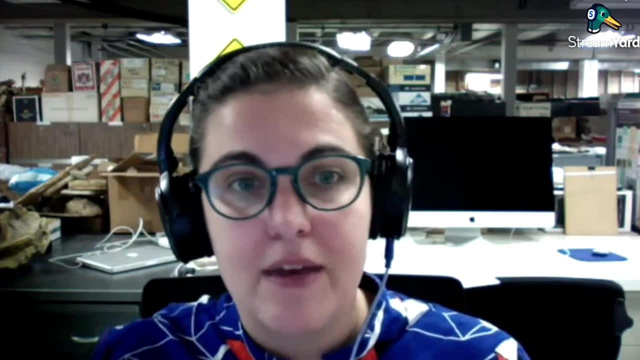 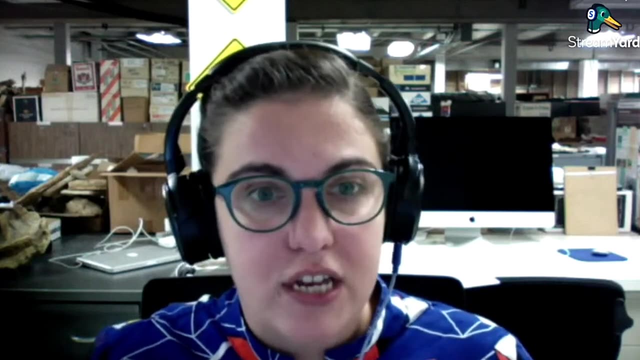 understand the mechanisms of evolution, the drivers of their evolution, um, you need to understand the climate, you need to understand the environment, you need to understand the ecology, how these things all play together and, as i mentioned, you often don't have um fossil plants and fossil animals. you don't have fossil plants and fossil animals. you don't have fossil plants and fossil 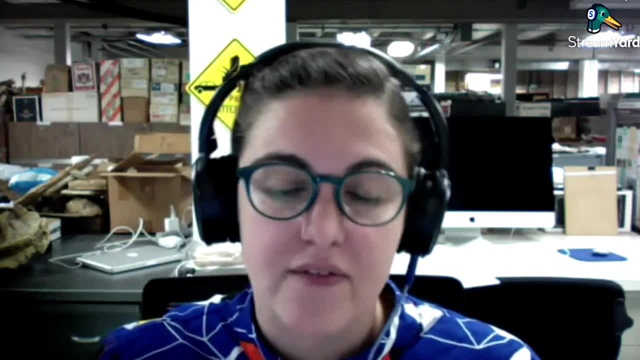 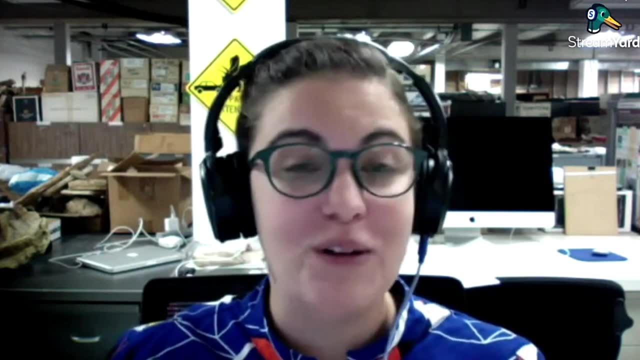 animals preserved together. so you have to get a little bit more creative in order to do that. and so, because you cannot easily make these connections- and there are a whole lot more vertebrate paleontologists and biological anthropologists than there are paleobotanists- often people will 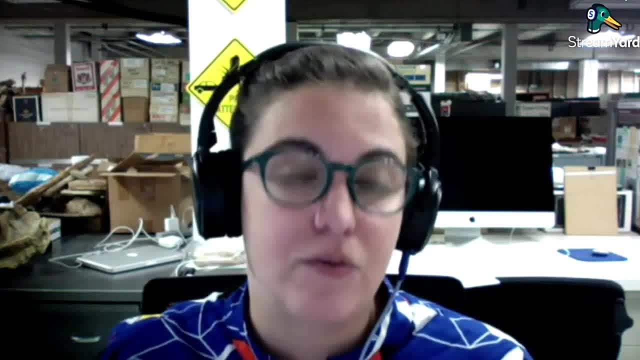 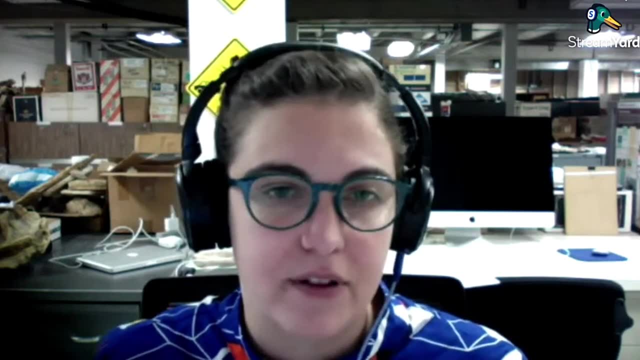 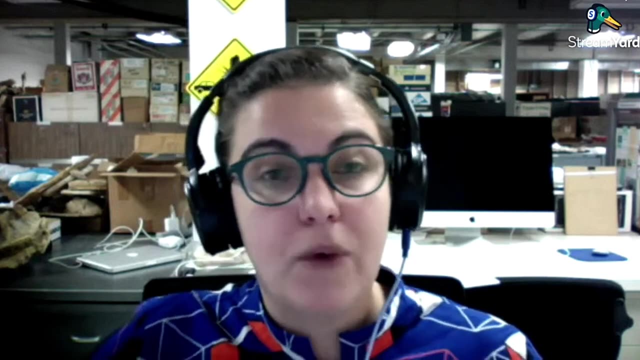 try to use other ways of getting there, and there's nothing necessarily wrong with trying to use animals to get a sense of the environment. there are ways that you can do that. for example, if you reconstructed an animal, probably um use brachiation, so they are swinging with their arms through the trees. well, in order to 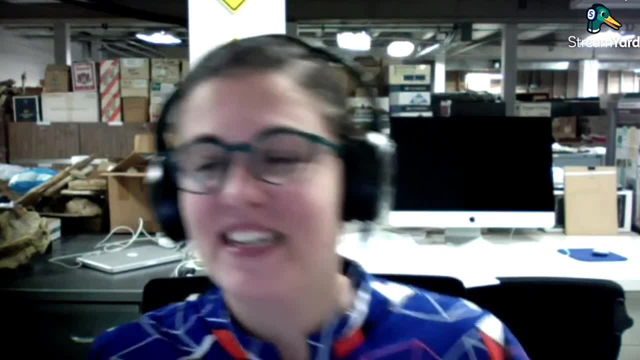 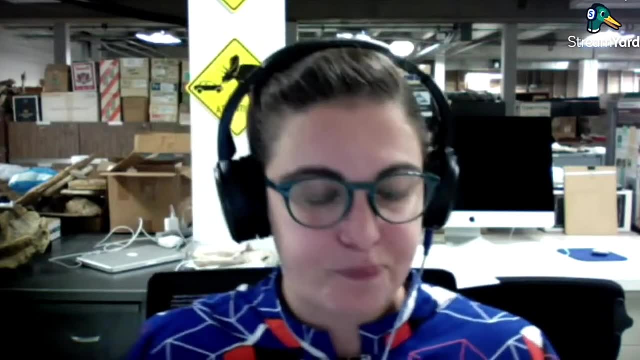 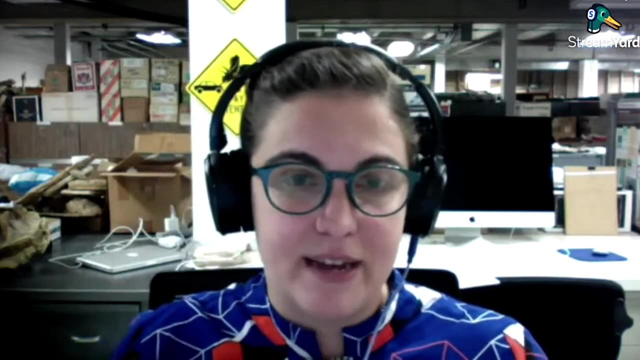 do that. there's got to be something to swing from. so, like you can, you can use things like that to get a general idea. but by and large, the reconstructions that are done that way um are very broad. um, you will reconstruct that it is an open environment or is it a closed environment? so 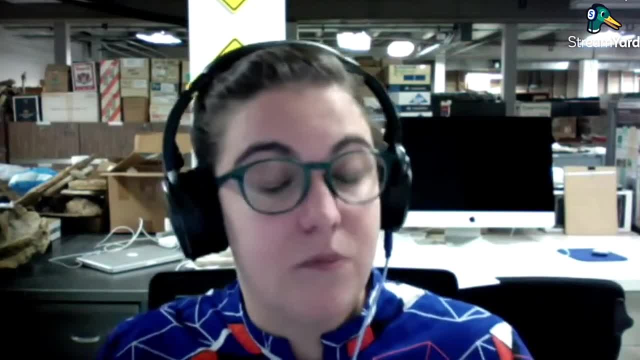 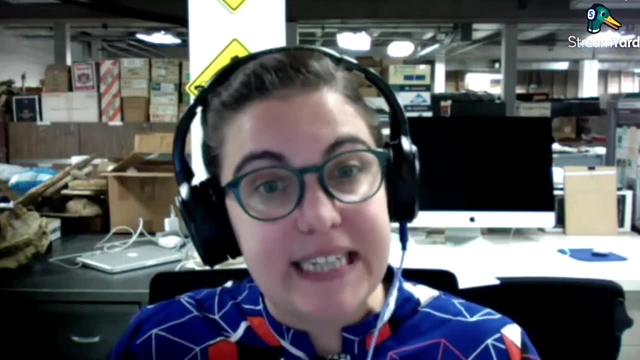 there's nothing above your head, there's a canopy above your head and that's broadened, the way that you see the image looking like that nose and background- and just sit there and think that would work, if but so, for example. what you would find then is that you would go into the fossil. 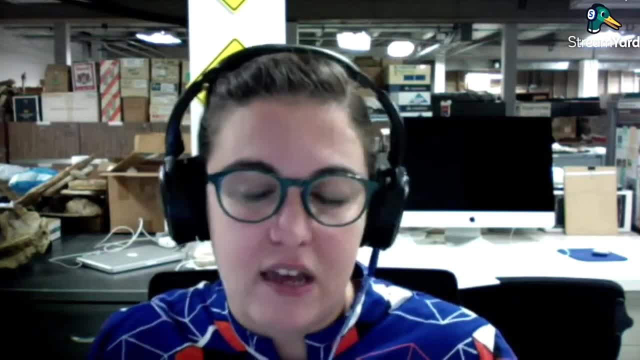 environment or fuckan complex. you might come up with these migrants, but you're just evil and those do. They hurry the way they are Ink it, building e from the philanthropy, but you're doing it because they have all these things that way. you're at that scale. they're wandering around and some of them are dead and 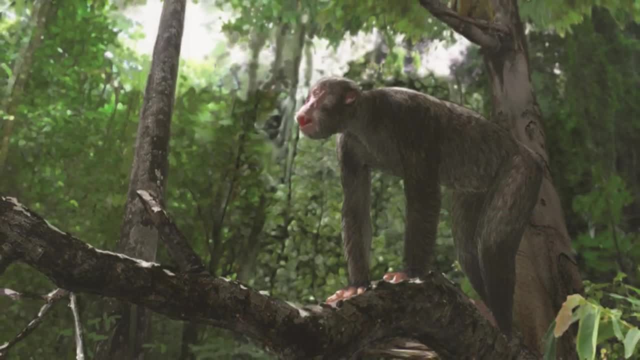 some of them are still in參i immunity and some can survive in lecturer cards. and then you're there like nothing really matters because there's so much of it. the human office is like: what are you going to get from it anyway? then, like the human health as such, it's just. 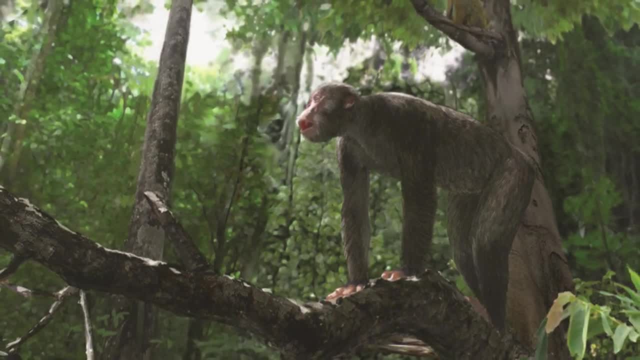 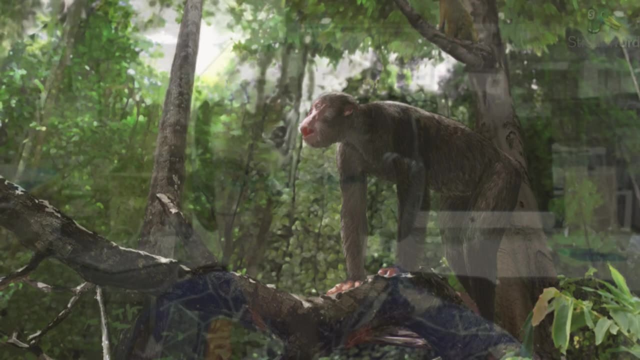 a normal level of that kind of thing that you still have to go back andIf you wanna think about that, that in terms of today we'll be maximal. họ gain agecalled the no that primates lived, or you know early primates. they lived in forests. well, we found early primates. 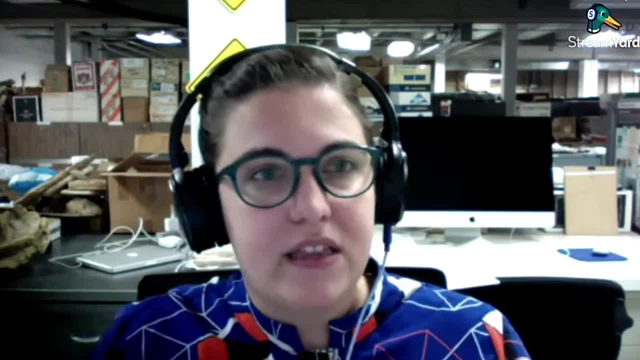 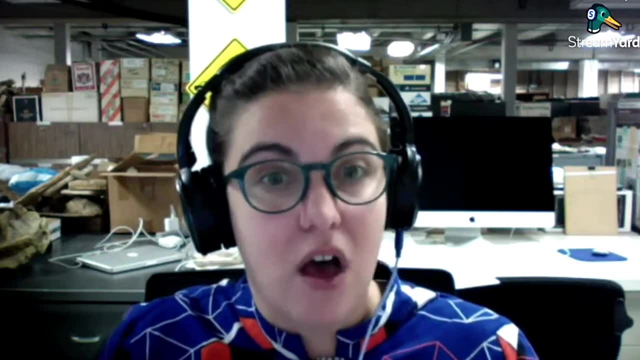 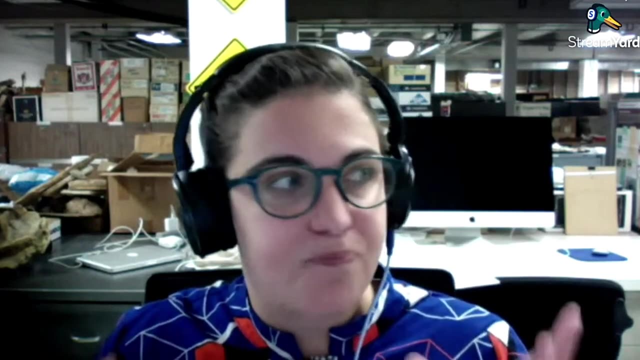 so they must live in forests, and we don't really we didn't necessarily have any other way of supporting that, except for that's what we expected. and so anytime we saw a early primate, we would, or early, um you know, hominid, early miocene ape, we would. basically, oh, we have one, it must be a. 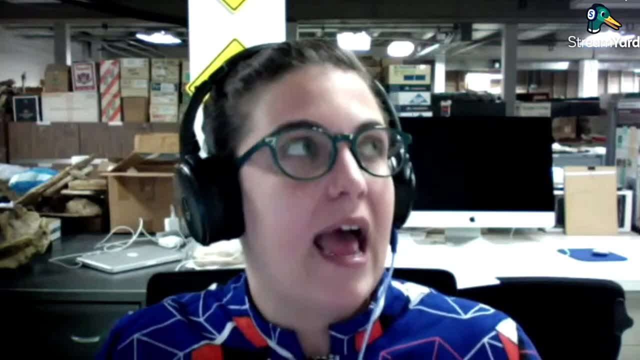 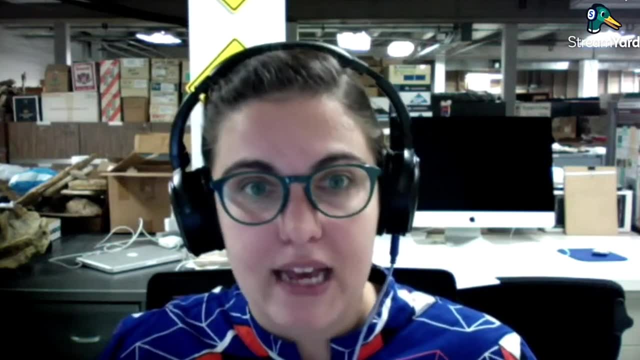 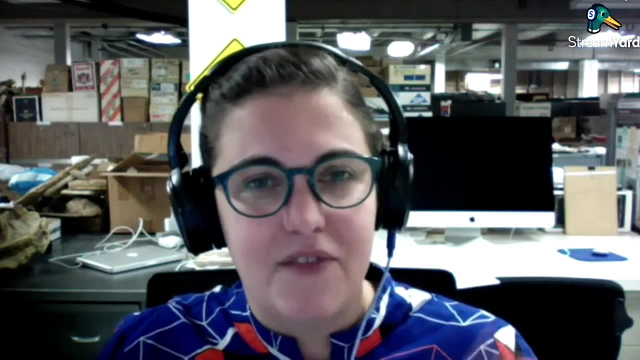 you know closed canopy, we have one. it must be a forest, and which has also led to a really strange understanding of the climate in the environment of the early miocene in africa, like there has been for years. there was this idea of the pan-african forest, basically that, like through the oligocene, 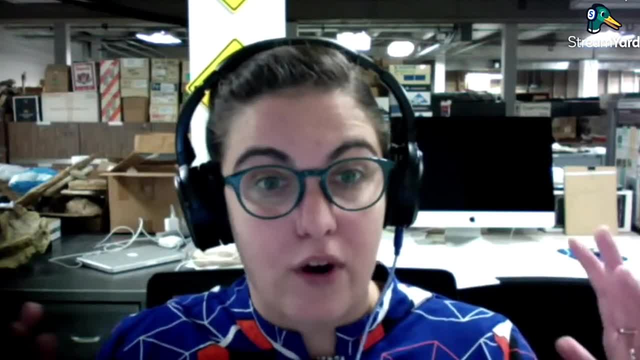 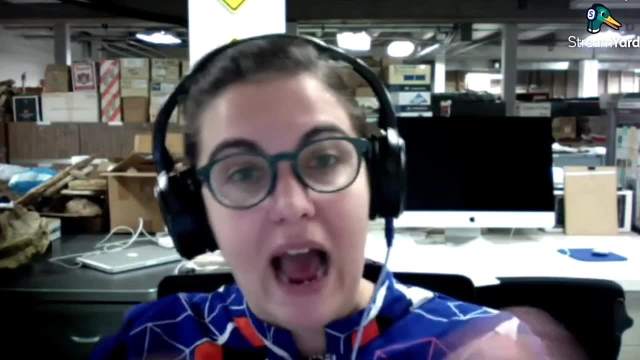 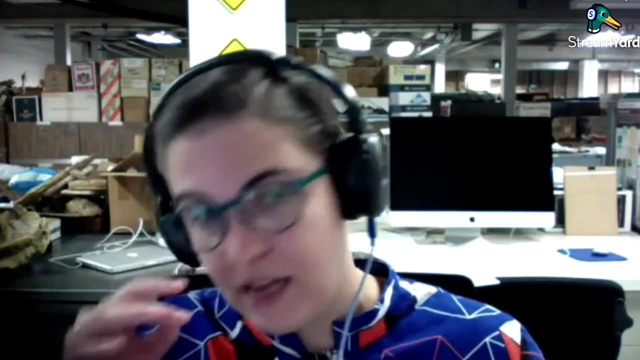 into the miocene you only had a forest. it was basically like wall-to-wall trees. yeah, that was much more nuanced than that, because if you actually look at the different fossil floras um and look at the reconstructions of their climate and their environment, you can see that. 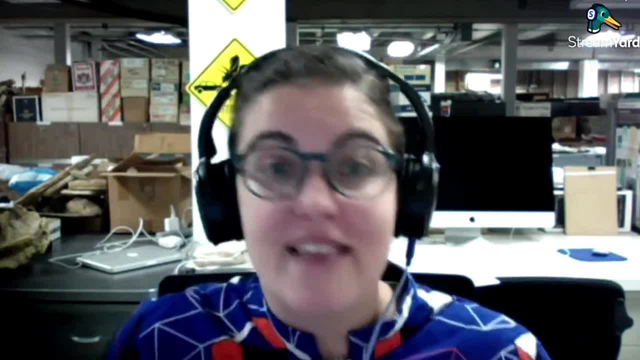 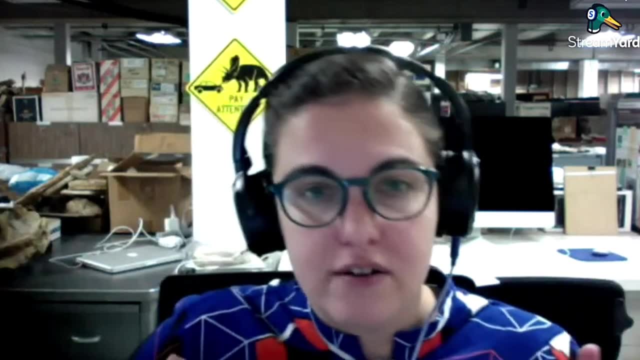 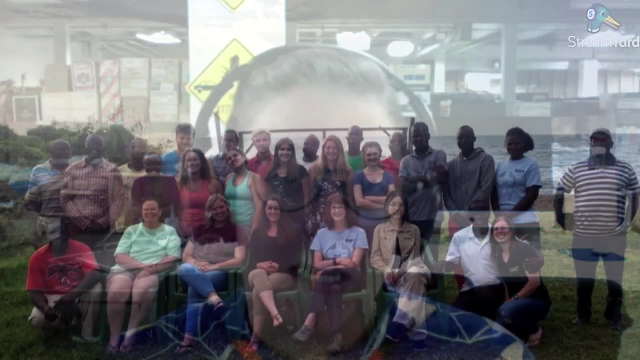 like africa today. it was a mosaic, so you didn't have grasslands yet- it was too early for that- but you had more open environments, more closed environments. it wasn't just like wall-to-wall trees, and that was one of the things that we found with um, the research that we did in uh. 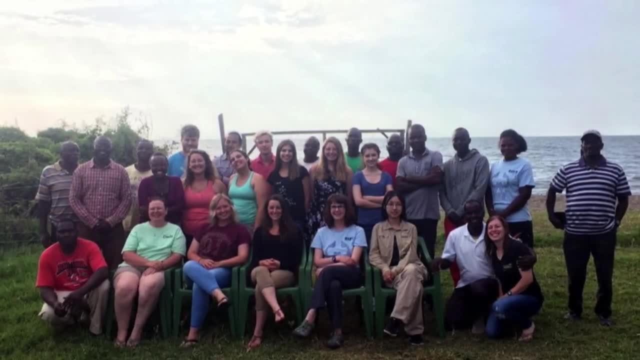 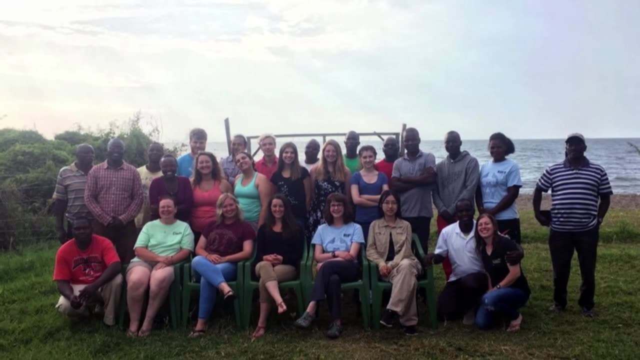 western kenya from the early miocene and the early miocene, and the early miocene and the early miocene was that we looked at these um different fossil localities that had closely associated plants and animals, so close enough in time that we were pretty comfortable um generalizing between 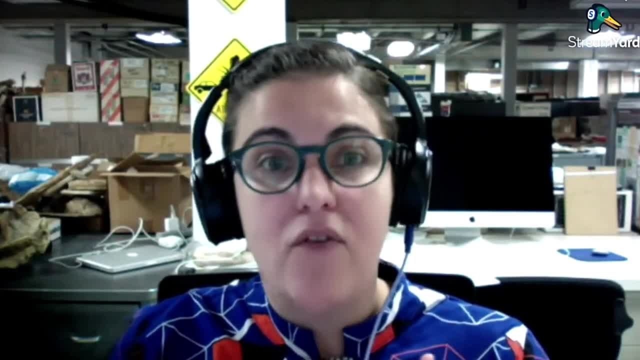 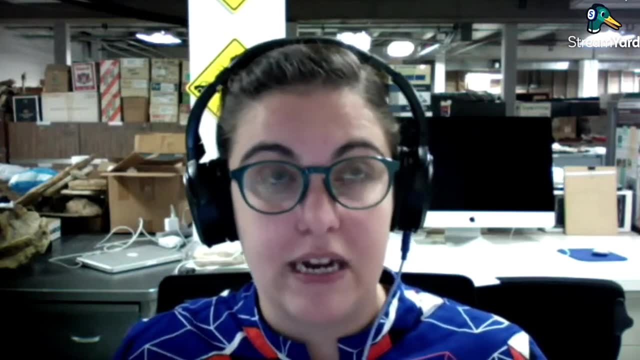 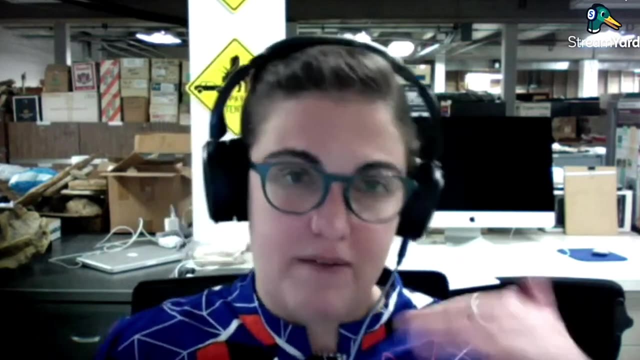 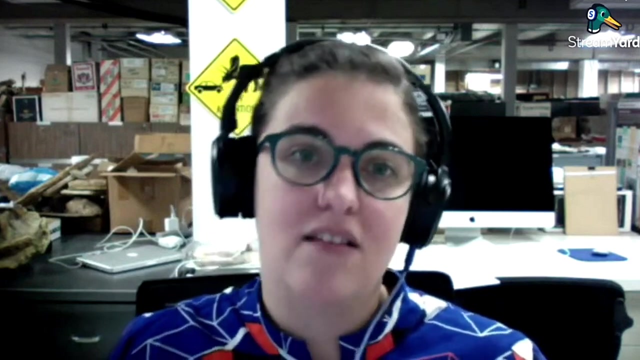 the two um and we found that we would have almost complete turnover of the plant community. like very little similarity in the plant community. we had very different uh environments, very different in terms of precipitation, similar temperature but very different amounts of precipitation- and most of the animal community would be entirely different, except for the primates you would have. 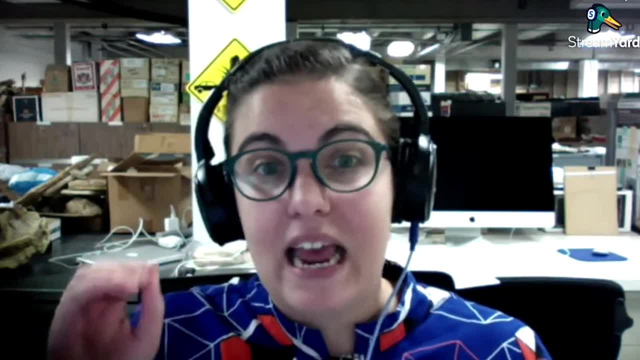 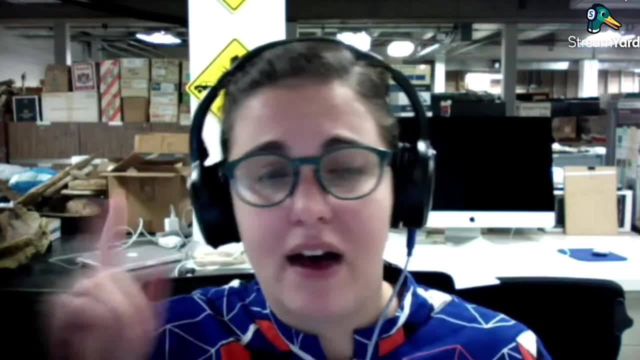 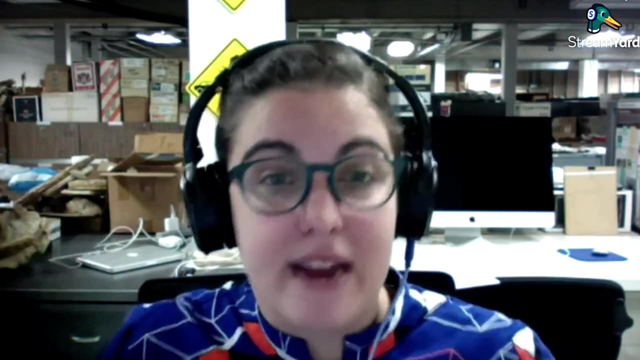 the same species of miocene apes in in in a? um open, canopy, um ephemeral pond, so a pond that's going to dry out seasonally, as well as in a closed, canopy rainforest environment. so, instead of use, instead of the circular reasoning that we had been using, that oh. 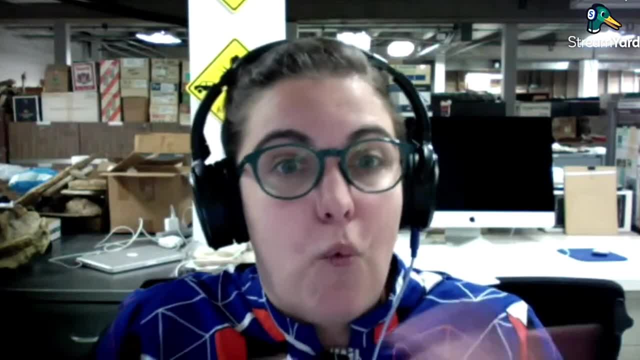 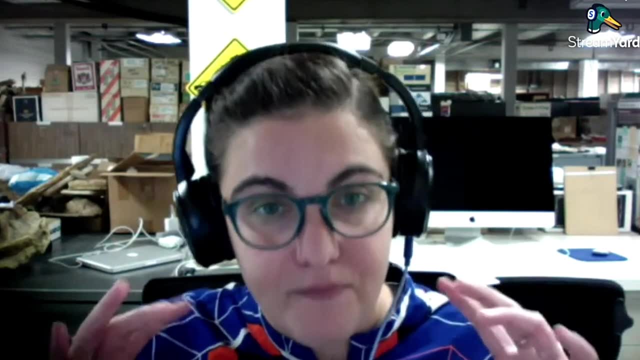 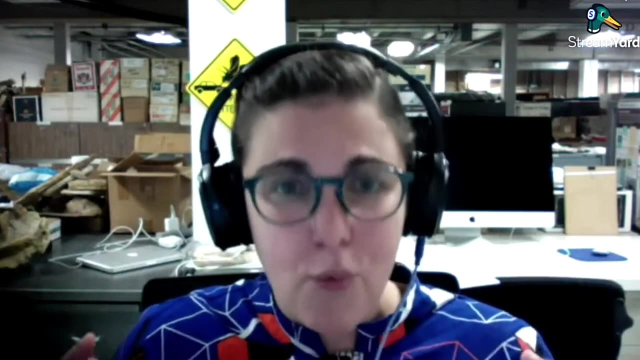 primates. that must mean for us, it's the opposite: we could live anywhere. that was what was actually driving us. that we were not restricted um to these very small environments, that we were able to adapt and change and live in open or closed environments. we weren't limited to the forest. and that changes. 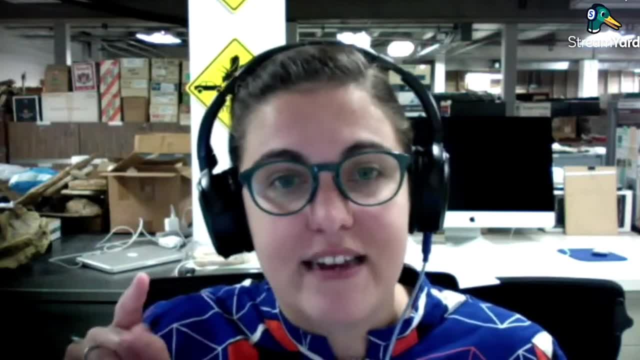 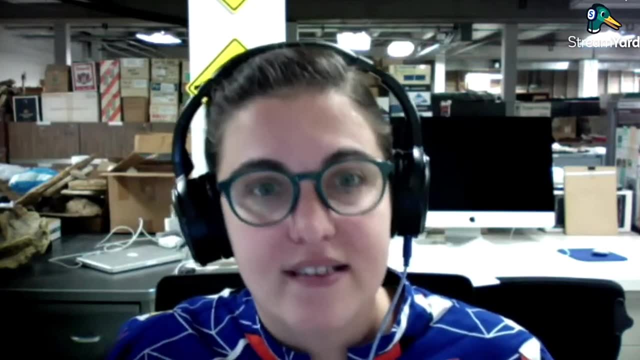 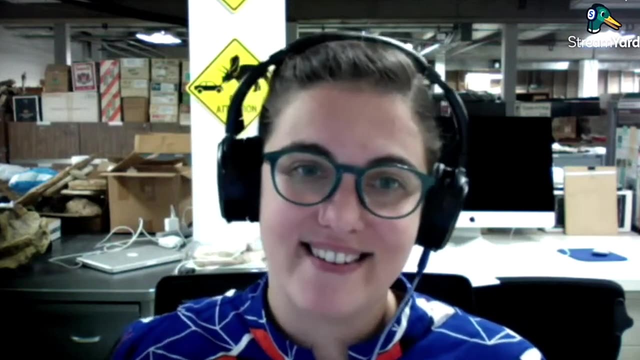 our understanding, you know, not being limited to that circular reasoning. seeing the nuance helps us get a better idea of, okay, what were the drivers then? if it wasn't, you know, oh, suddenly everything opened up when we had the grassland expansion in the miocene. yeah, so that's why we persisted. i 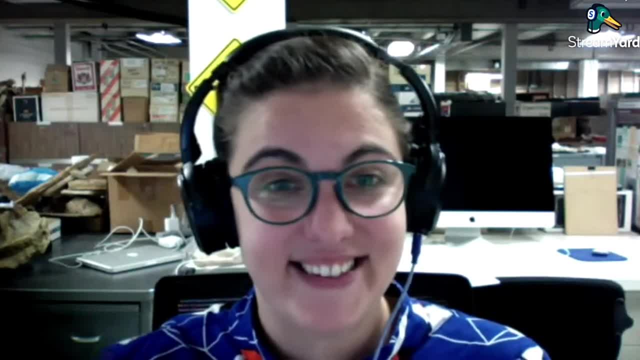 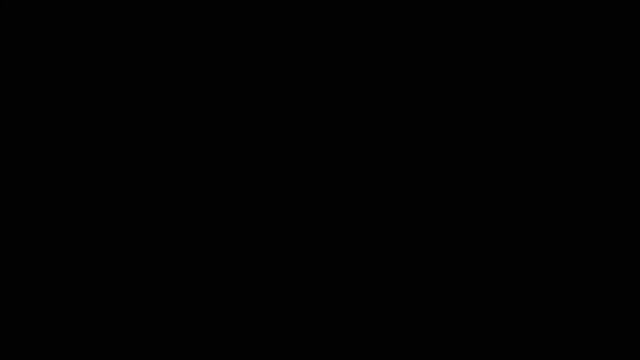 suppose because, uh, we thought, oh, here's a problem, let's not just sit on our asses, let's let's adapt to this and move on. exactly exactly. it's been great having you on the show, ali. paleobotany was always something that intrigued me, and i think it's been a great experience for me to be able to.